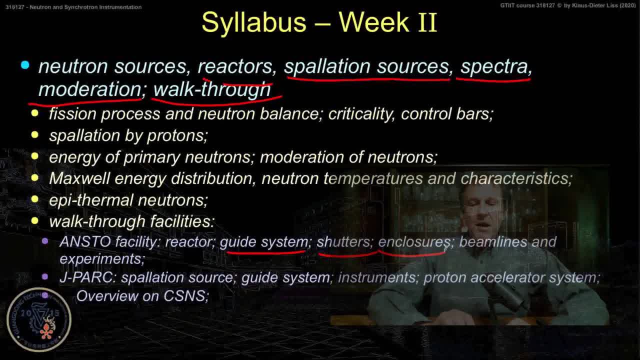 At J-PAC. I demonstrate a spallation source, a neutron source, and then I talk about the energy distribution. We have neutron temperatures and I specify the characteristics of those, And then an external buildings, The external buildings, which is based on the proton accelerator. 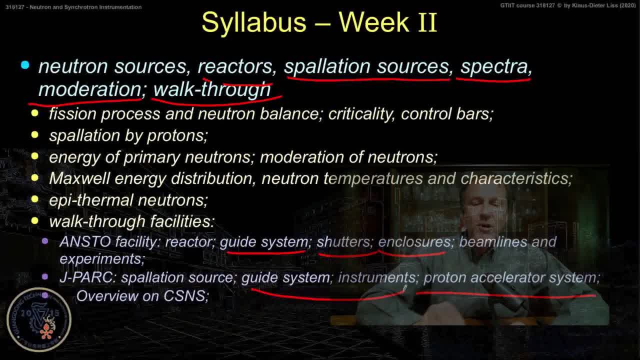 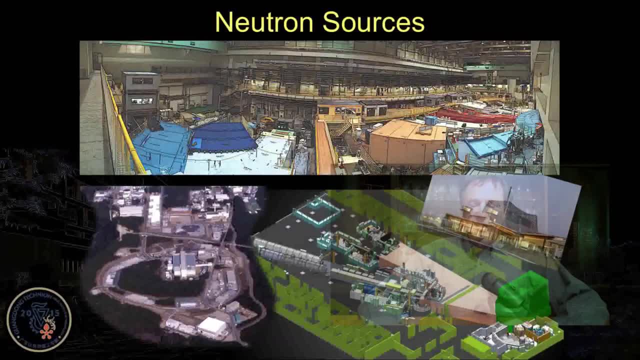 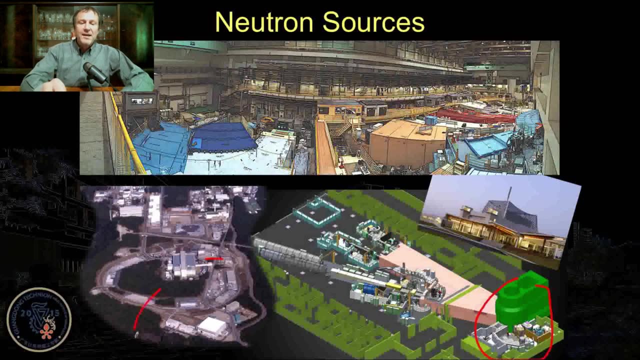 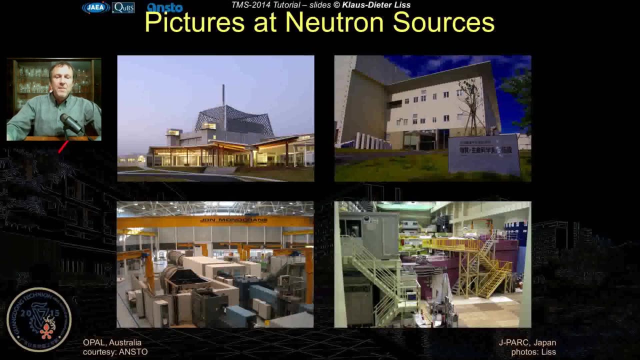 system. briefly introduce the experimental halls And at the very end a very brief overview of our CS&S. a Chinese spallation neutron source. So what are neutron sources? I mentioned already they can be nuclear reactors Or they can be spallation sources. Here are few images. So the external buildings, they are pretty. 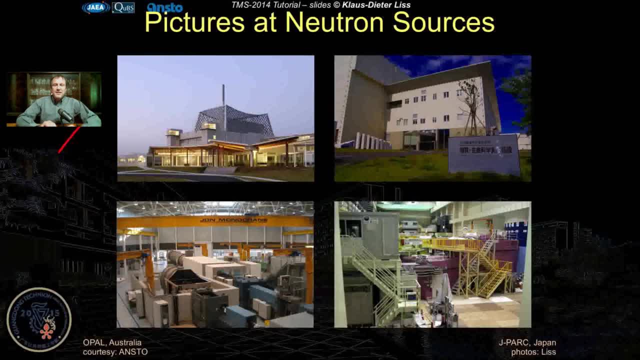 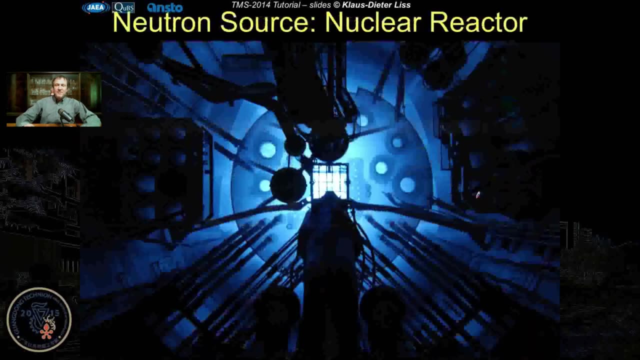 big user facilities. We see here the ANSTO facility and the J-PAC facility to the right. Typically those facilities have big instrumental halls which are shown to the bottom, hosting immense instruments. Let's talk about the nuclear reactor. This is a view into the opal nuclear reactor pool. So we have the 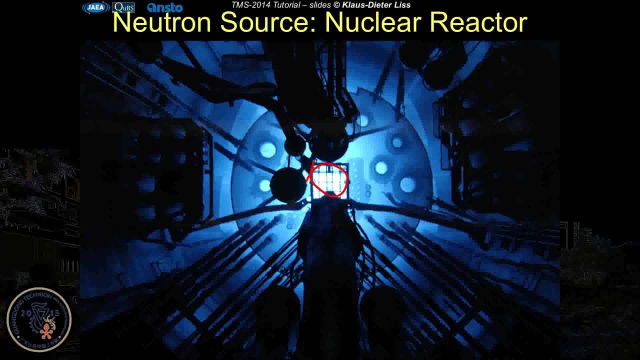 reactor core. underneath here There is a lot of radiation coming. The blue light is the Cherenkov radiation, which is the ultra relativistic electrons. They go through water and emit that light. We have a vessel here. This is a vessel later we see- of heavy water reflector and moderator. and then we have a few. 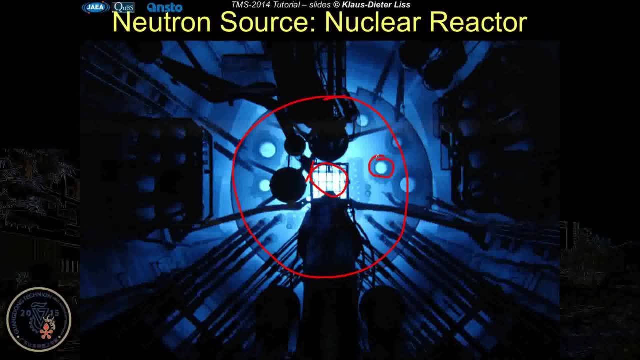 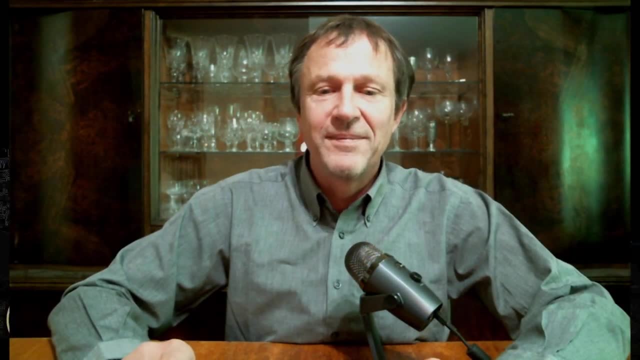 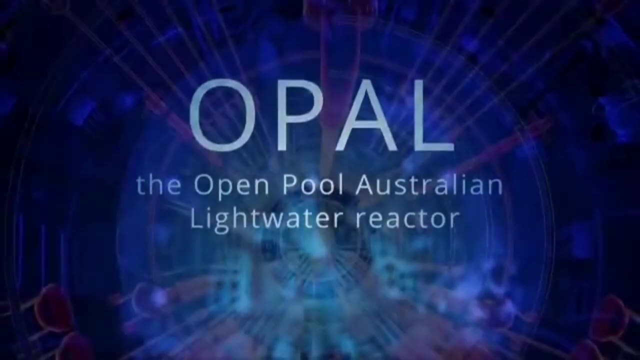 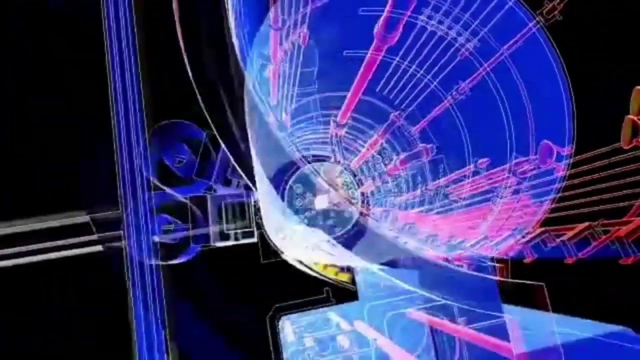 other inserts for irradiation of isotopes and as well as a cold source. With this in mind, I like to play you the movie Opal: the open pool Australian light water reactor, A multi-purpose research reactor that produces more than 80% of Australia's nuclear medicines Irradiates. 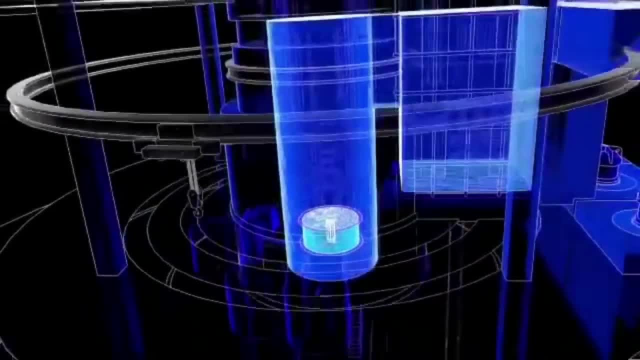 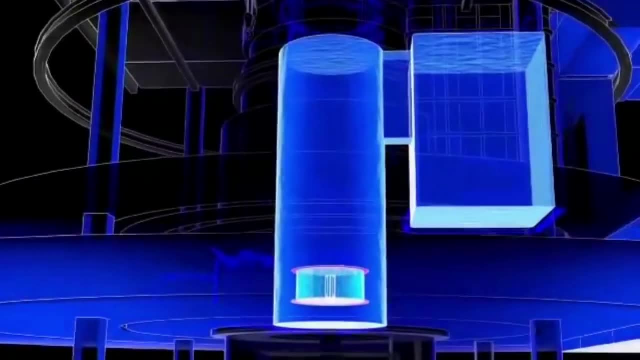 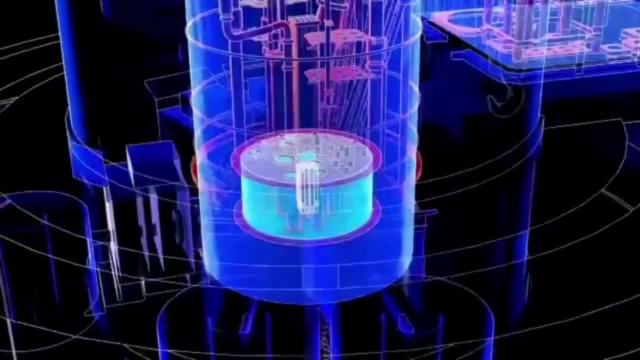 more than 10% of the world's silicon and produces neutrons for materials research. The reactor pool is 13 meters deep And filled with super clean demineralized water. At the bottom of the pool is the reflictive vessel and within that vessel 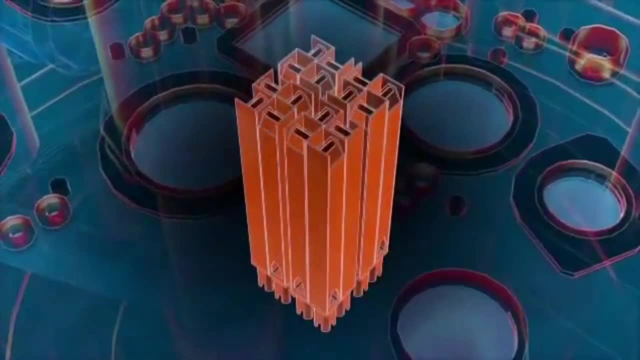 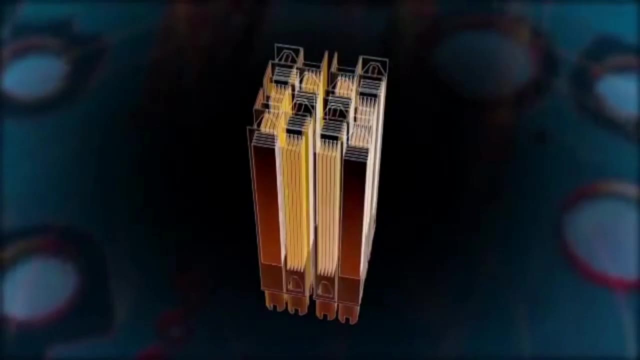 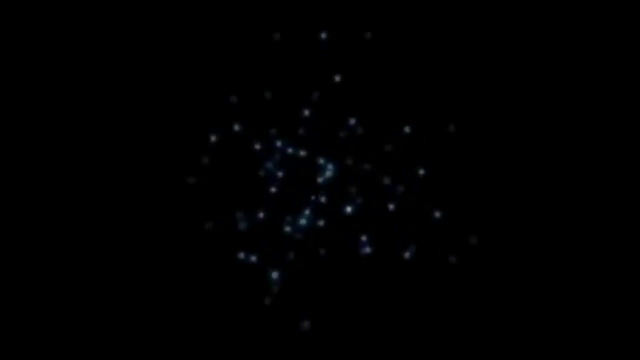 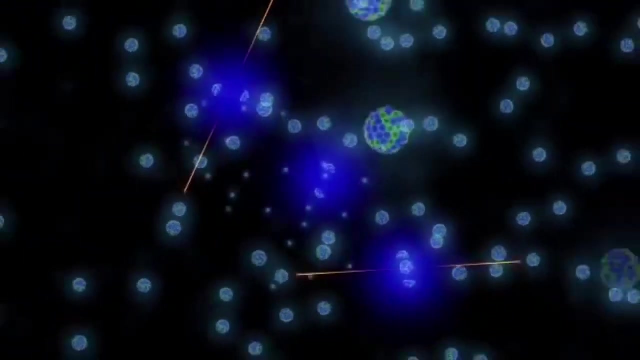 the reactor's heart, A compact core of 16 fuel assemblies. Inside is less than 6 kg of uranium 235., The naturally occurring isotope of uranium that can sustain efficient chain reaction. Some energy and generally two neutrons is released when a uranium atom is split by a single neutron. 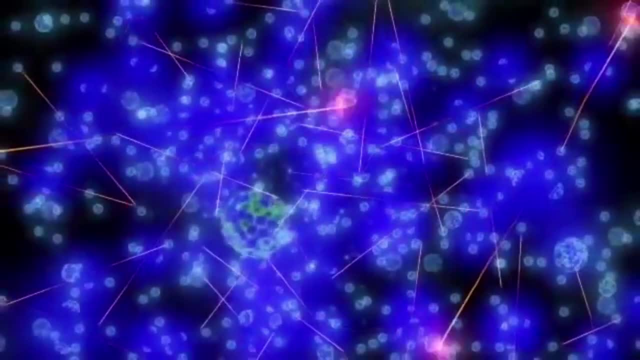 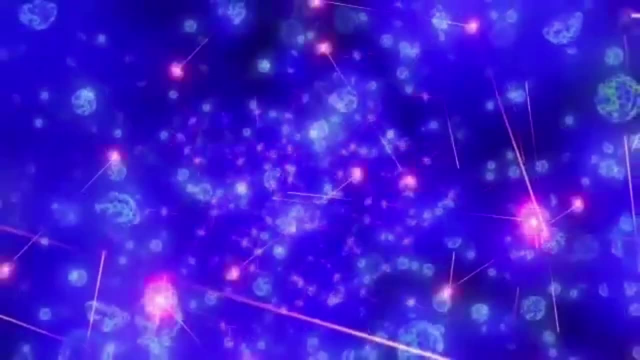 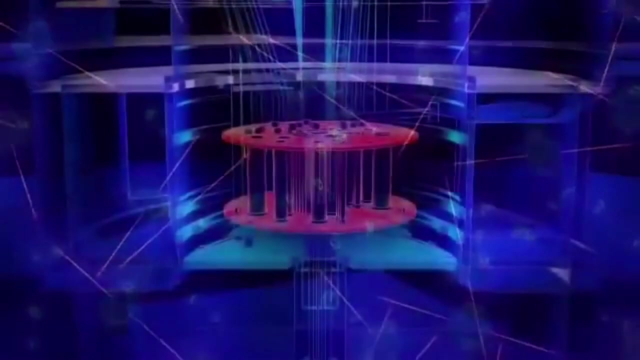 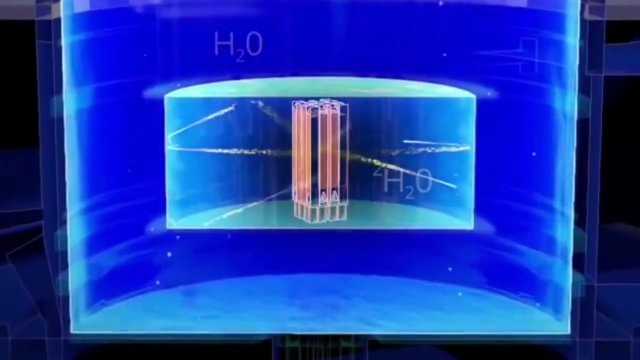 Two neutrons turn into four, four into eight and eight into sixteen, and so on to a maximum of 400 million million neutrons per square centimetre per second. The reflector vessel acts like a mirror and reflects neutrons back into the core to maintain fission. 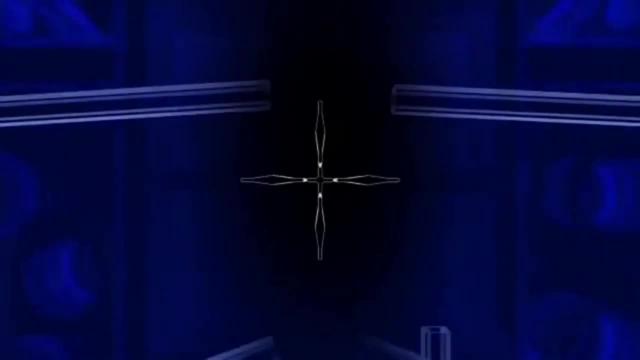 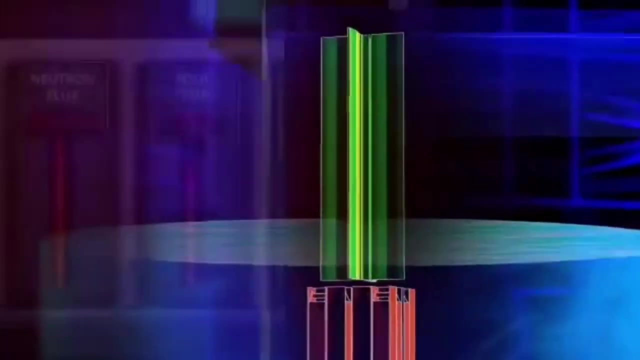 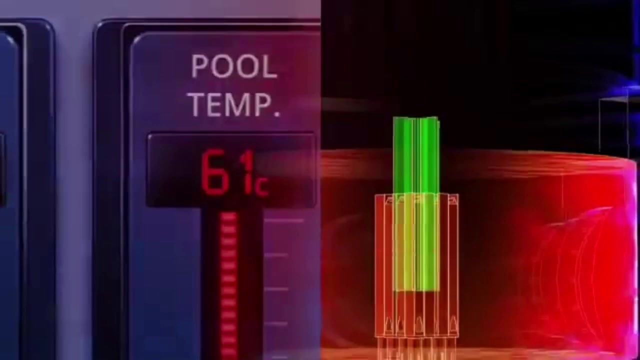 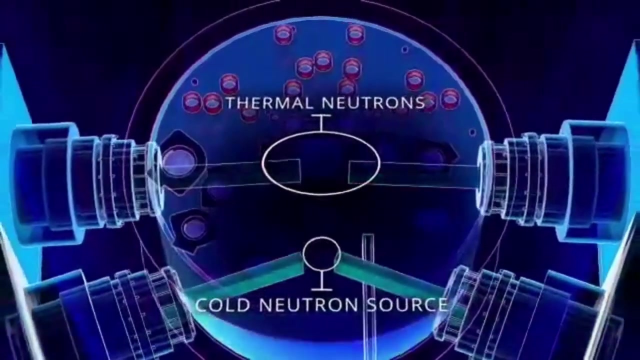 Five neutron-absorbing plates called control rods help manage the fission reaction. If the reactor temperature exceeds 60 degrees Celsius, the control rods are automatically inserted in less than half a second. OPAL is a neutron factory for research. Two neutron sources supply cold and thermal neutrons into the Neutron Guide Hall. 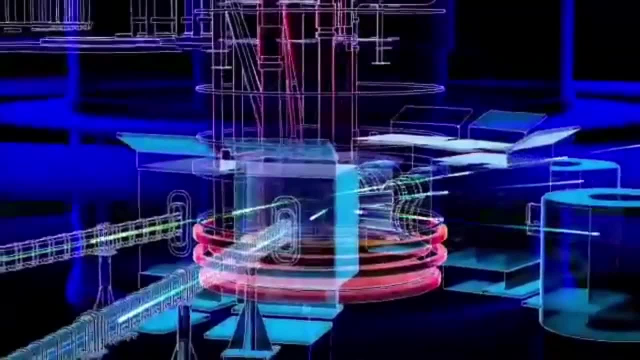 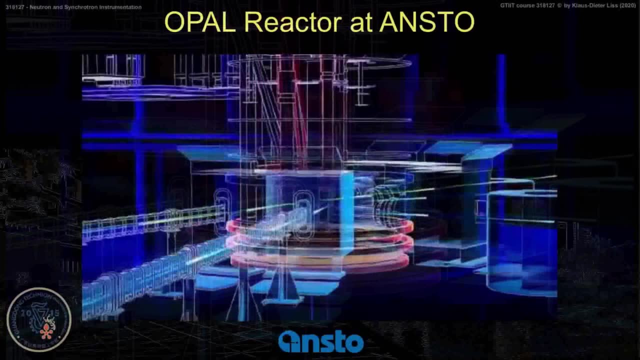 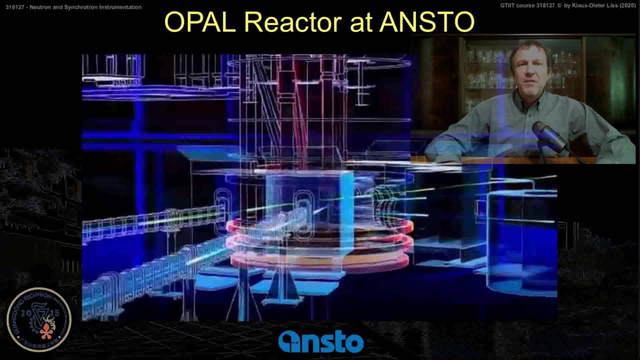 where an amazing array of scientific research is conducted. Yes, nice movie. So after this introduction, I want to go a little bit through the processes and the details. what is happening here? We have had a reactor core, we have had a reflector vessel. 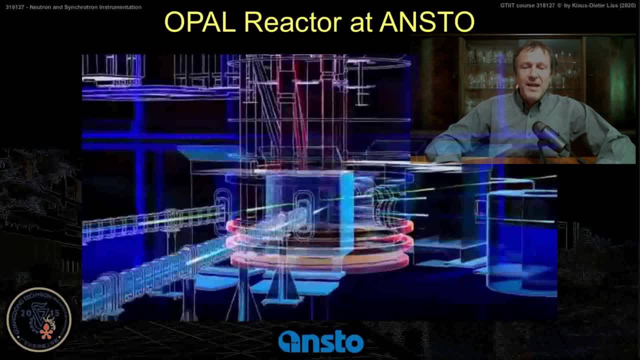 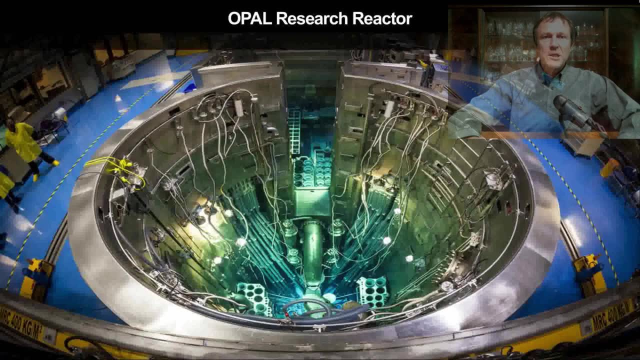 we have had a cold source and we have a moderator and neutron guides where the neutrons are taken away to the instruments. Again, a nice picture of the OPAL facility, The reactor pool here filled with water. OPAL stands for Australia's Open Pool Australian Light Water Reactor. 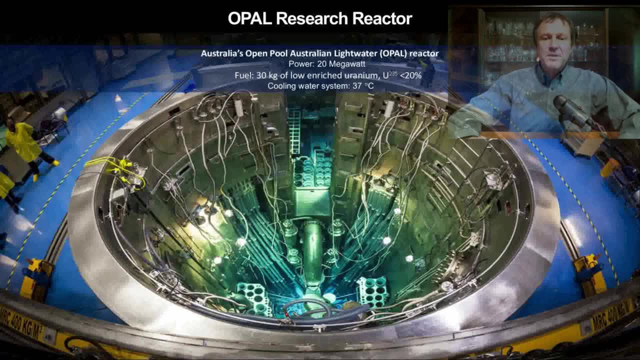 The power is 20 megawatts and the fuel is about 30 kilograms of low enriched uranium- uranium-235.. The enrichment is less than 20% And the cooling water system is about 37 centigrade. so about your body temperature? 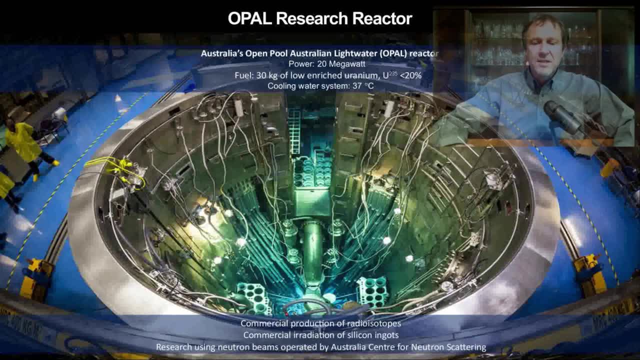 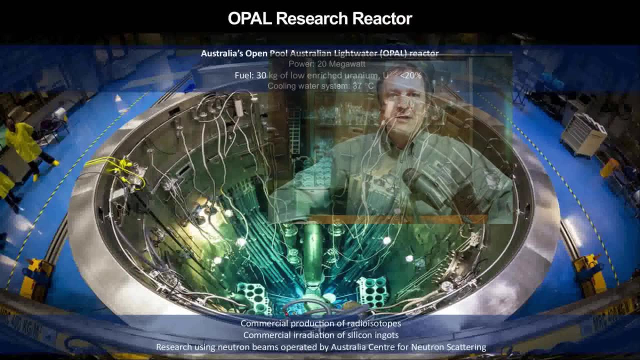 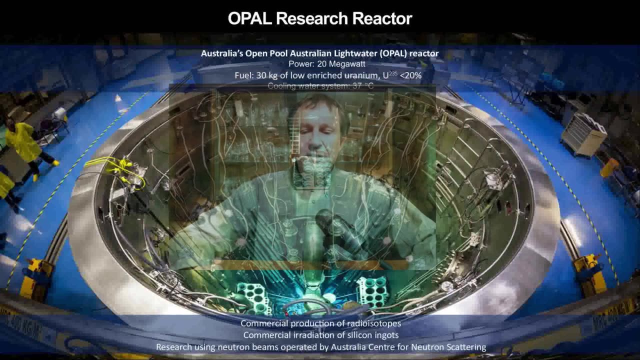 OPAL produces commercially radioisotopes, also for nuclear medicine and irradiation doping of silicon ingots for the semiconductor industry in the world. But there is also research using neutron beams operated by Australia's Centre for Neutron Scattering or the former Bragg Institute. 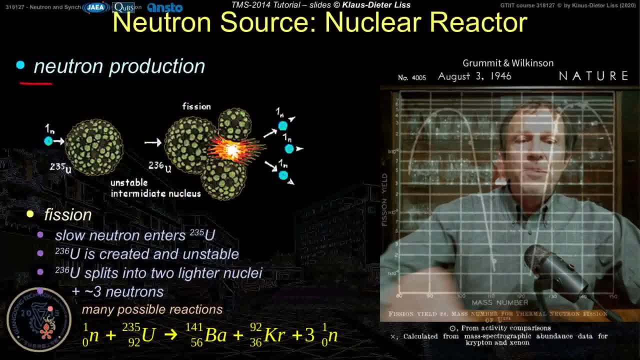 And this is what we are interested in. The neutron production in the reactor occurs by nuclear fission. So we have uranium-235, and we have a neutron coming into the nucleus and sticking to it. So temporarily we create uranium-236, which is unstable. 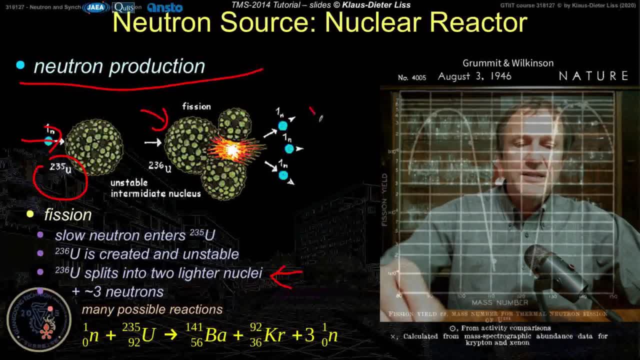 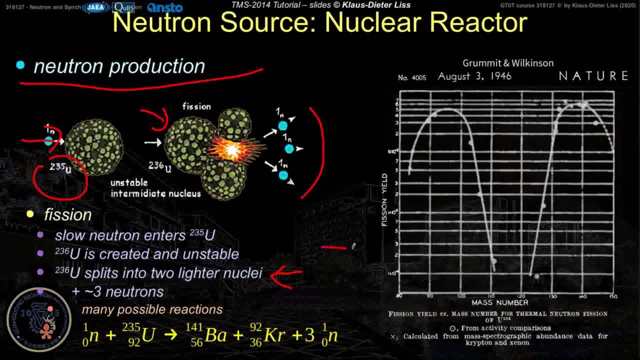 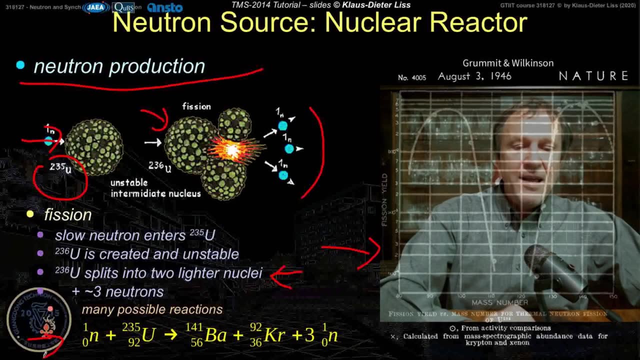 and splits into two lighter nuclei plus about three neutrons. Some reactions two, some reactions three neutrons. There are many possible reactions as shown here to the right. So we have a distribution. One of the reactions is like one neutron plus uranium-235. 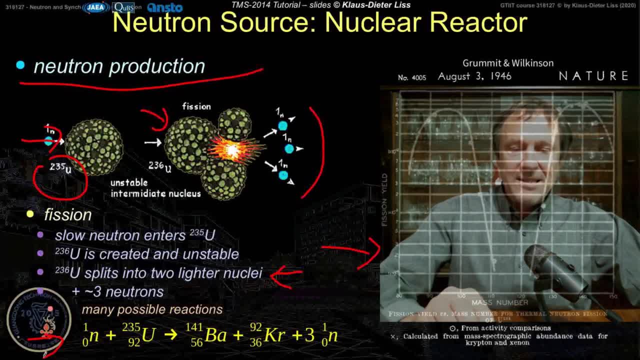 becomes barium-141 plus krypton-92 plus three neutrons, And the balance of this equation is the number of nucleons, which is the upper index at the isotope. So one plus 235 equals 236, equals 141.. Plus 92 plus 3.. 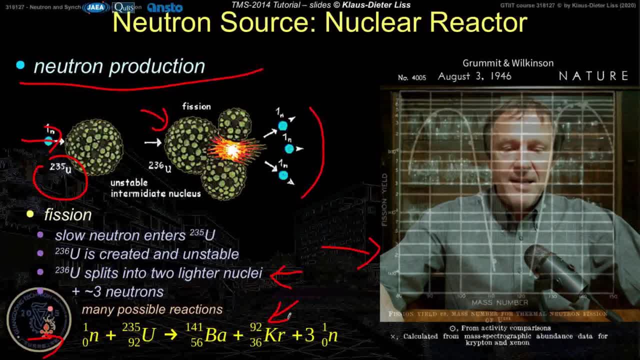 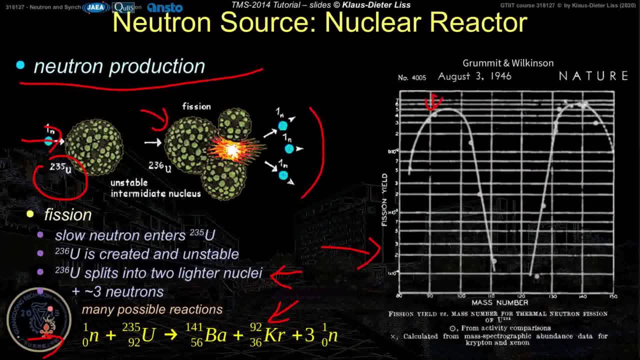 The distribution is shown here, to the right, The example of barium-141 and krypton-92.. So this is the krypton-92 and the 141 is about here. There are the isotopes at the maximum yield. However, there are other reactions. 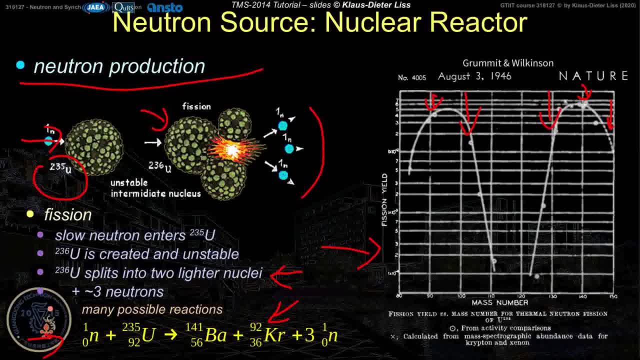 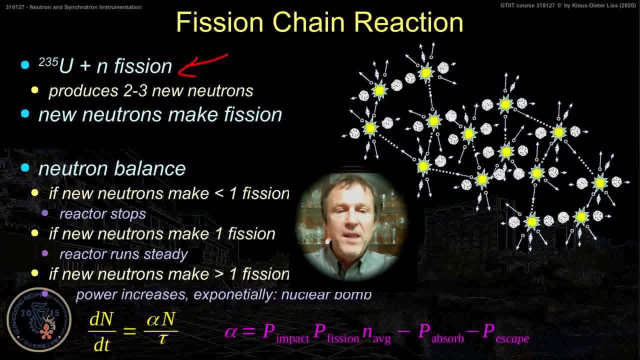 For example, this goes together with one here, And so on. So once we have had the first nuclear fission by introducing a neutron, we produce two or three more neutrons which can make another fission again, And this is called a chain reaction. 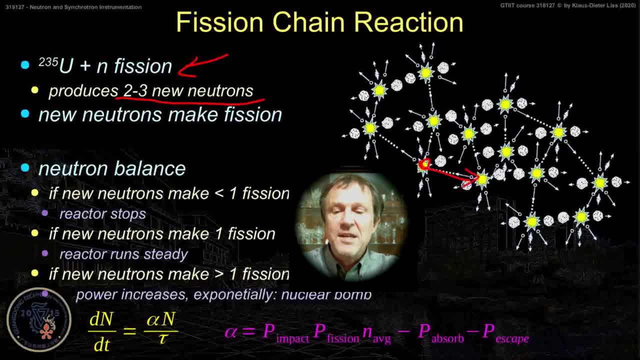 The fission or nuclear chain reaction. We have one fission here. The neutron produced hits another nucleus and induces a fission there. For a continuous chain reaction we need to regard the neutron balance If the new neutrons make less than one fission. 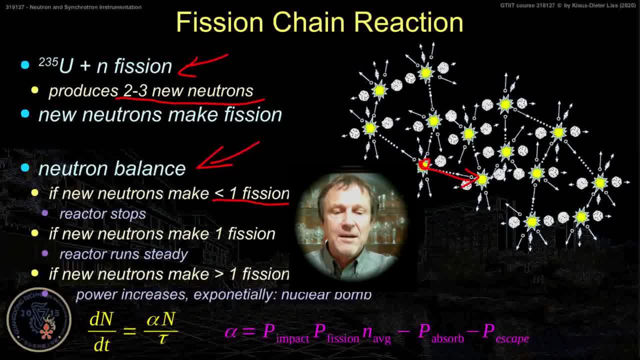 of course. then the reactor stops because it's not sustainable. If the new neutrons make about one fission each and two neutrons escape or get absorbed, then the reactor runs steadily. And if the neutrons may make more than one fission, 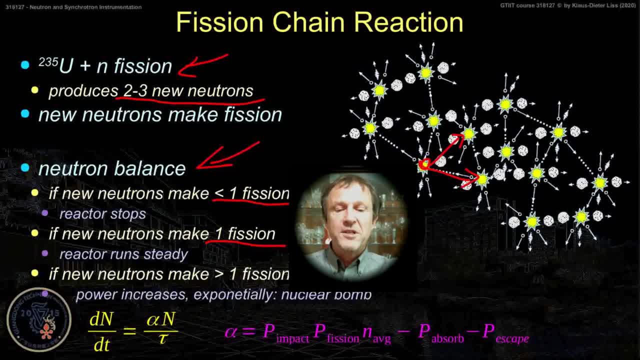 so two of the produced neutrons make another fission, then the power increases. If we look to this equation here, dn over dt equals some probability times, n over a reaction time, tau, where n is the number of fissions. So if alpha is constant, 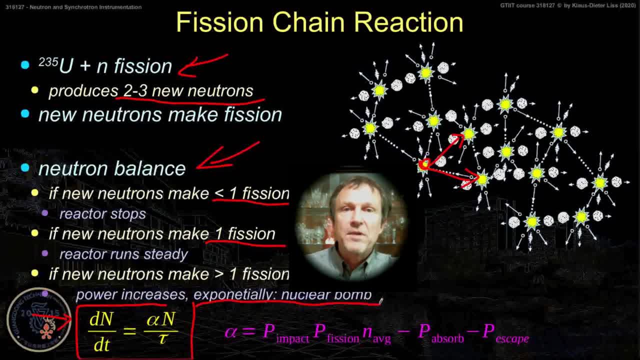 then n would increase exponentially and we would have a nuclear bomb. We don't want that here, So we have to continue. We control the alpha as a function of the fission, So alpha equals the probability for impact, so it's kind of the cross-section. 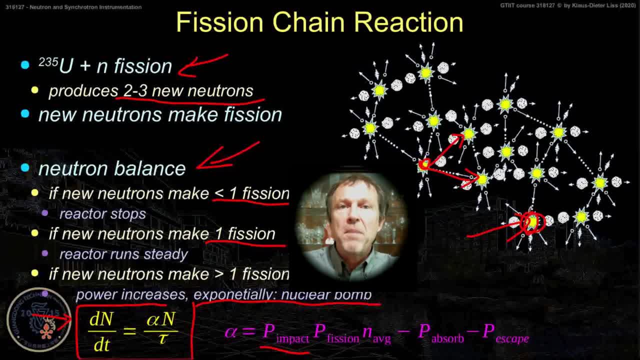 the impact to the nucleus, then the probability of the nucleus to make a fission times the number of neutrons produced in average. So I say there are two to three neutrons produced, depending on the nuclear reaction, Minus the probability for absorption. 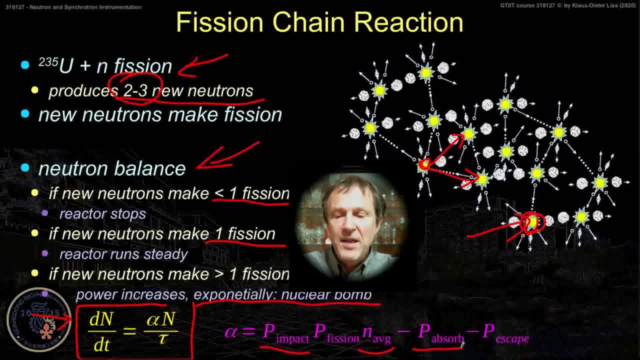 So some neutrons are disappearing from the system and others they may just escape from the system. They may go to our neutron guide, Those neutrons who escape which we want to have for neutron experiments. But we need a certain number to keep the fission chain reaction going. 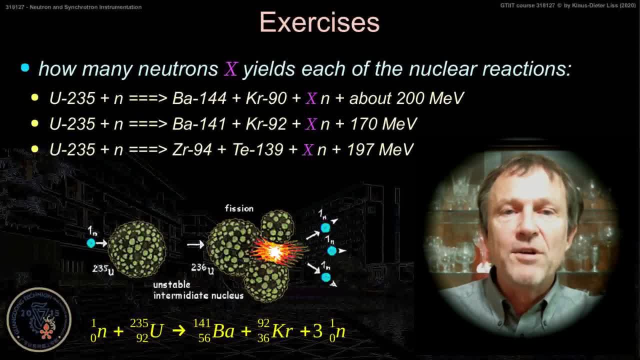 I like to give you the exercise how many neutrons x yield each of the nuclear reactions. I've given you one nuclear reaction here which you may find up there, and there are two more nuclear reactions, So please tell me for each. 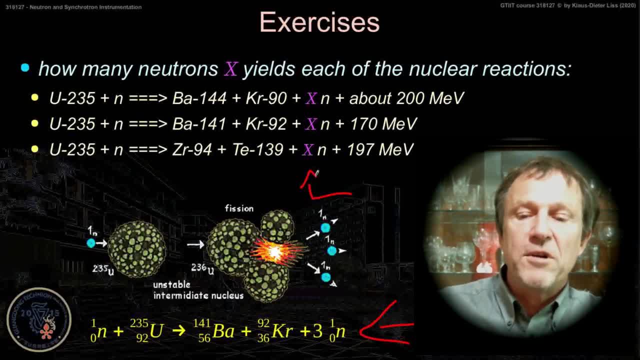 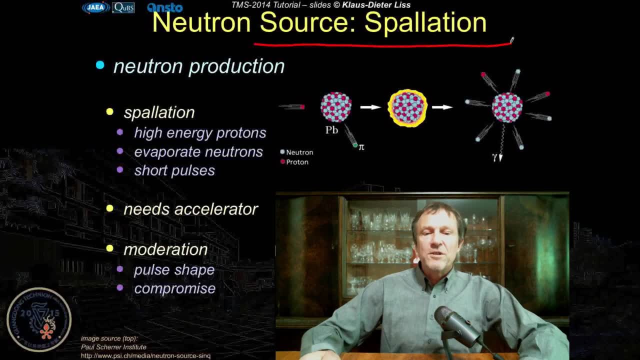 what is the number x of neutrons coming out of those reactions? In contrast to the nuclear reactor, we have the spallation source. In the spallation source you take a high energy proton, a high energy nuclear particle, and bombard some heavy metal. 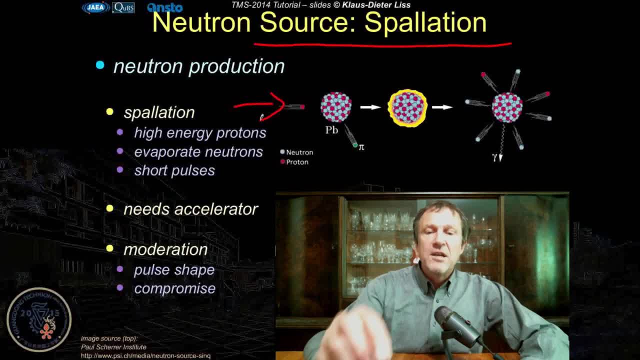 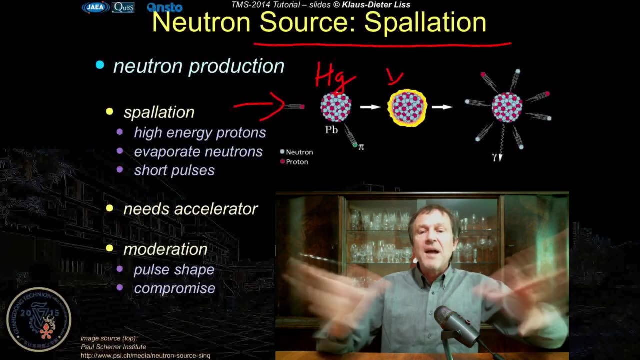 some heavy isotope with a lot of neutrons. So lead or mercury, Hg are those heavy metals used for spallation. Then when the proton hits this nucleus, it gets excited, so it starts vibrating and eventually it gets so hot. 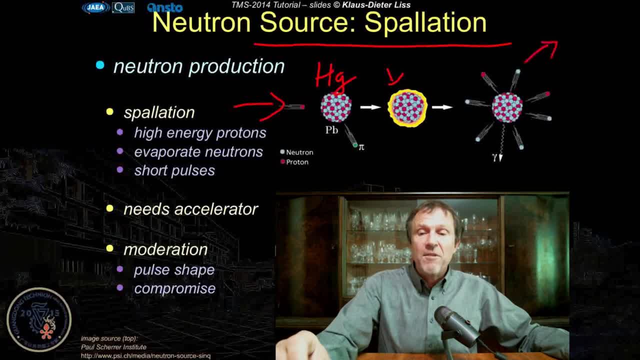 that it evaporates some of the nucleons. so it will evaporate some neutrons and some protons generally. One advantage of the spallation source is that one can make short pulses of the proton beam, so we get short pulses of neutrons coming out. 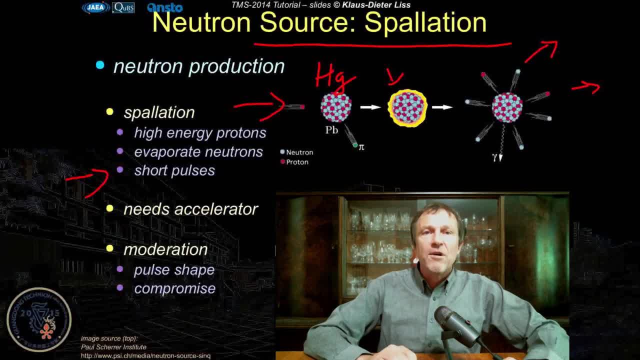 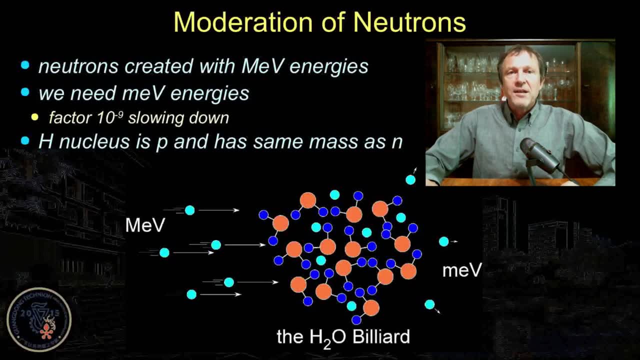 short time flashes of neutrons And that we can use later on, as I will show you in subsequent lectures, The neutrons created in the reactor, in the spallation source. they have mega electron and volt energies, So one mega electron volt. 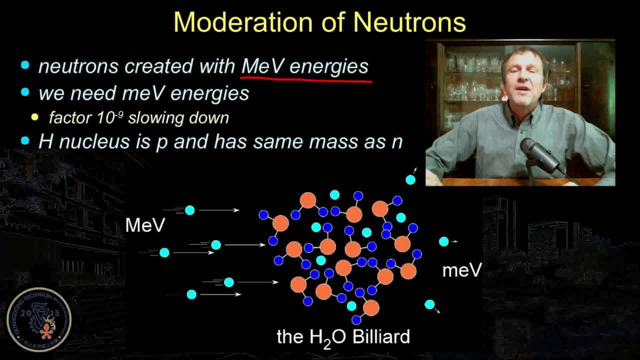 equals ten to the sixth electron volt, And they even can have hundreds of mega electron volt of energies. But for the solid state physics, for the investigation of materials, to have wavelengths around one angstrom, we need millielectron volt energies. So we have to. 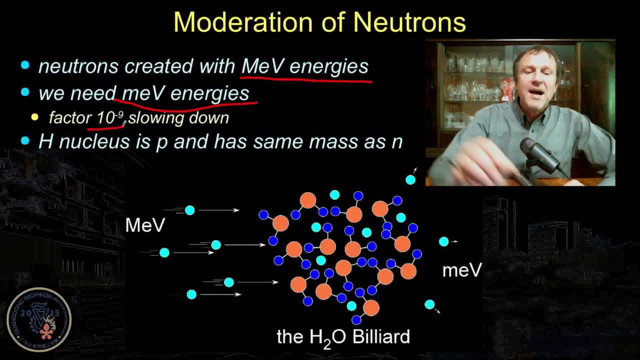 slow them down at least by a factor of ten to minus nine. And that we do by playing billiard. You all know the pool game. We take balls which are hydrogen nuclei, nothing else but a proton which very much has the same mass as a neutron. 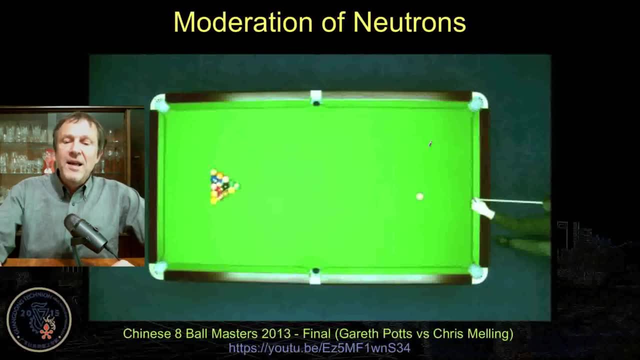 So how does this work? this nuclear billiard? Let's say to the left: this white ball is the high energy neutron and you have protons sitting here in this triangle at rest. Now what happens when the white ball hits this triangle? They scatter. 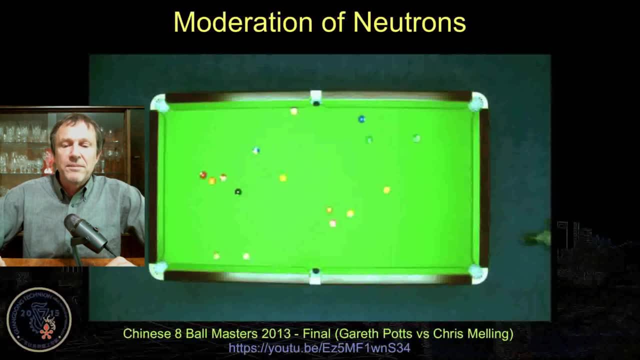 and you see the white ball is going towards the top and loses a lot of energy. I will play that again. So watch the white ball. it will go to the top and later on it will be hit by a yellow ball and retake some energy. 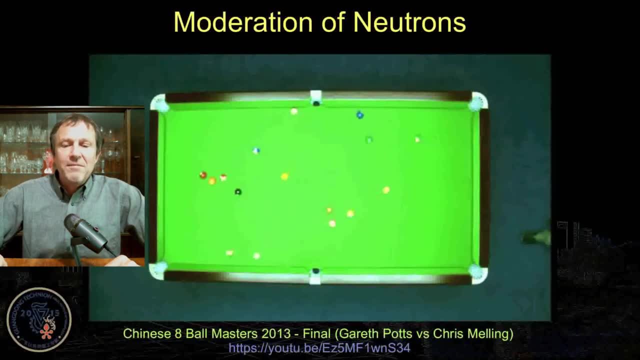 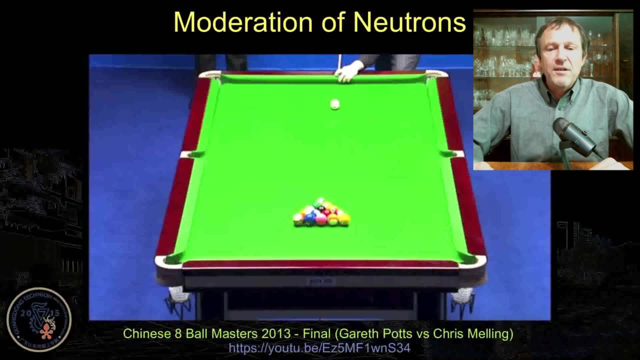 But over time now the white ball was hit by the yellow ball again. Here is the same short scene out of a different perspective. So the white ball will hit this triangle and watch. it will go to the left a little bit and then it will be hit by the yellow ball. 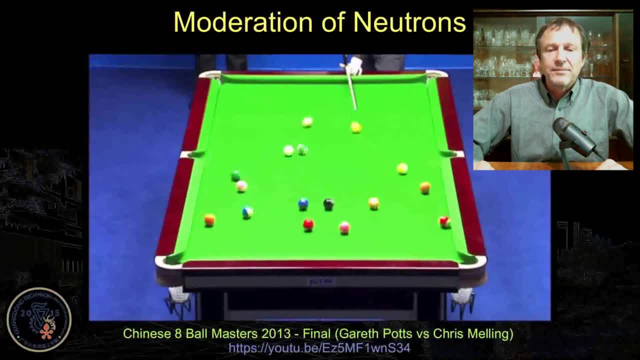 and go to the right. So we see how efficiently the white ball loses energy. upon its first hit. It transfers the energy and the momentum to the other balls And this is most effective when the white and the other balls have the same mass. So if we take protons, 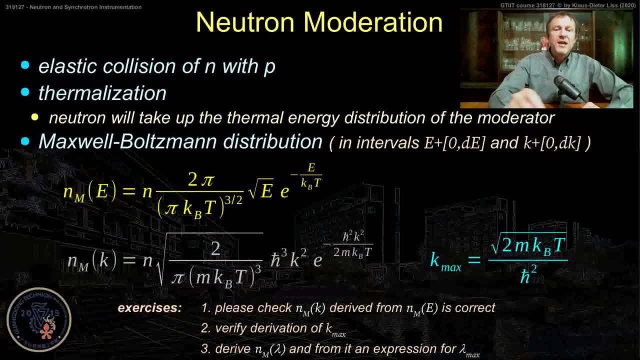 which have the same mass as the neutrons in water. Neutron moderation takes place by elastic collision of neutrons, for example in water, for example in liquid hydrogen, And this we call thermalization, because the neutrons, they will take up the thermal energy. 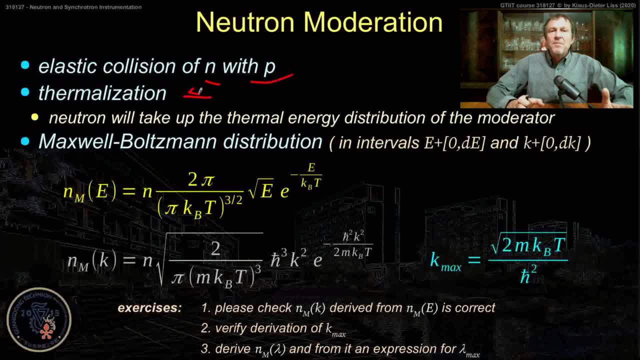 distribution of the moderator. In the billiard game. all the balls in the triangle they have been at rest and the neutron was the only ball moving. So then the neutron will stop eventually. However, in the water, all the protons they have this thermal. 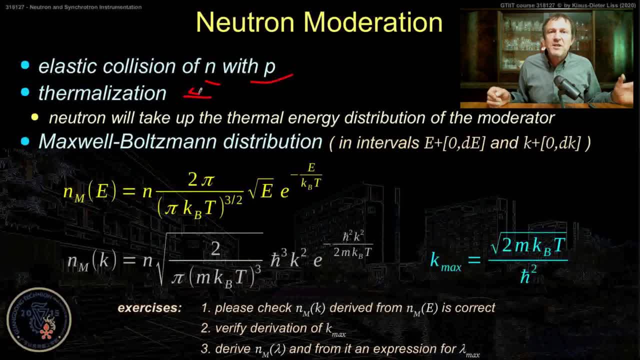 Maxwellian distribution of velocity, of momentum, of energy And therefore you have to consider the initial motion of the hydrogen and the motion of the neutron which then thermalizes, and in average the neutrons they take over this Maxwell-Boltzmann distribution for that given temperature. 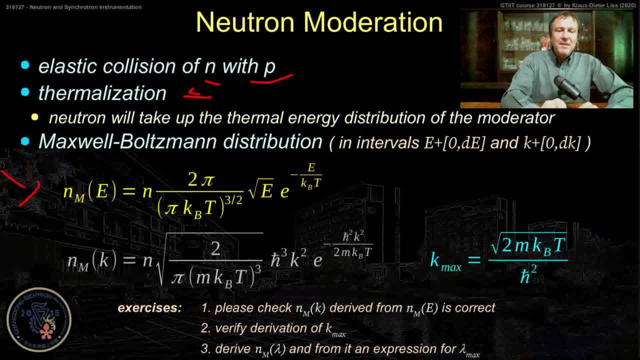 Which we can write down here, namely the neutron density of moderated neutrons in an interval: energy plus energy plus dE equals sum n0. so the total neutron density: 2 pi over pi kB T to the 3 half. then important here is the square root of E. 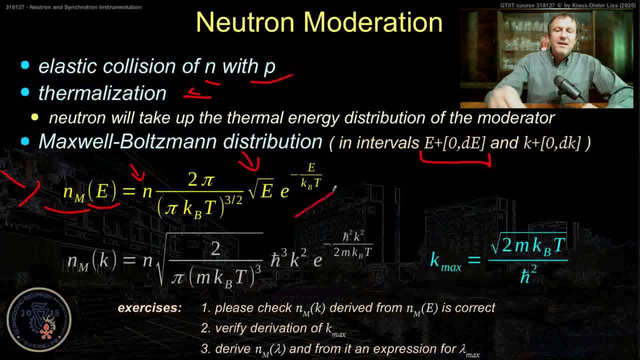 E times E to the minus E over kB T. so this is a activation factor. We can transform this to momentum space. then the moderated neutron density is a function of wave vector k. so in the interval k and k plus dk equals the total neutron density sum pre-factor square root. 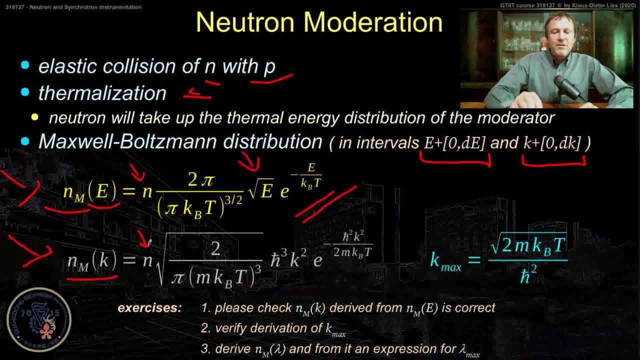 over 2 pi mkB. T to the 3 times h-bar to the 3, and then we have this k-squared. so this is important, we have the k-squared and that comes in here through the dispersion correlation between energy and k, E to the minus. 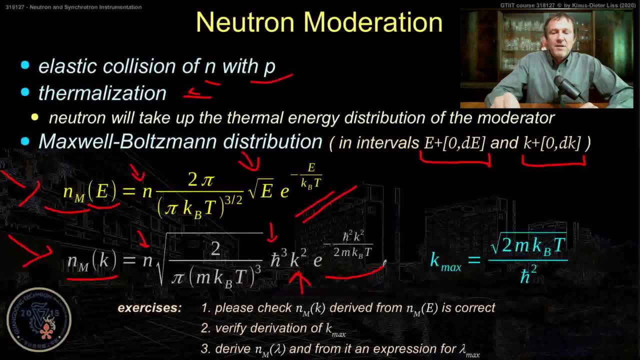 h-bar squared, k-squared over 2 mkB T. so we see, here it's the same factor, put the kinetic energy here and here we have the transformation term which produces the k-squared. I will give you some exercises. so the first exercise is: please check. 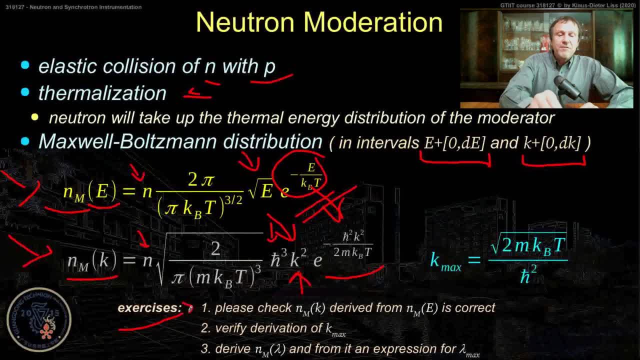 how to derive the second formula nm of k having the first formula nm of E. use the dispersion correlation. we can look to the maximum of this curve. so the maximum is then given by k. max equals square root 2 mkB T over h-bar squared, and I also want you to verify this. 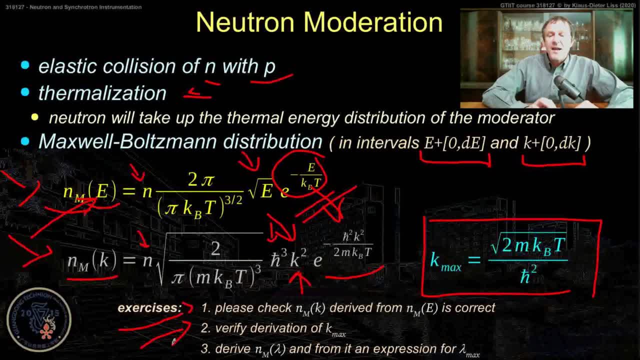 as I have derived already nm of k and the k max in my homework I let you derive nm of lambda and from it an expression for lambda max. so please derive that formula, nm of lambda- and give an expression of lambda max, and let's discuss the formula. 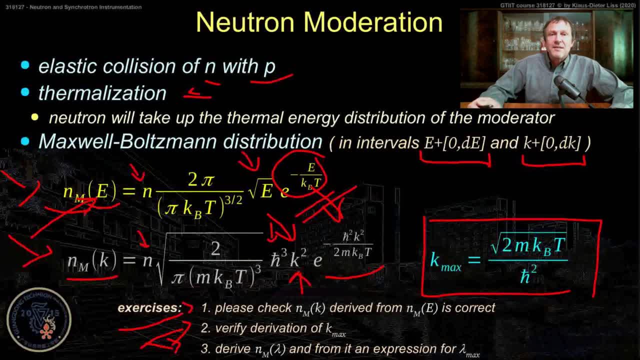 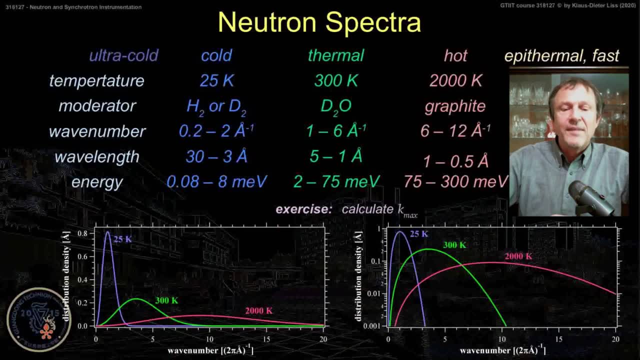 let's discuss them together next time. in some of the office hours we can plot this Maxwell-Boltzmann distributions for different temperature. so typically we consider cold neutrons, thermal neutrons and hot neutrons. so we can plot this Maxwell-Boltzmann distributions. 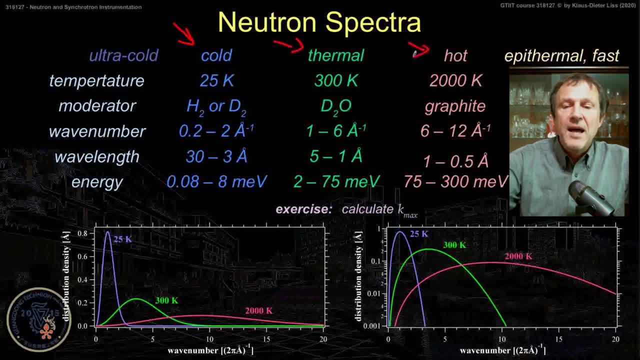 for different temperature. so typically we consider cold neutrons and hot neutrons in literature which are moderated by 25 k, 300 K and 2000 K temperature. the moderator for thermal neutrons or room temperature is 300 K. is D2O. we don't take. 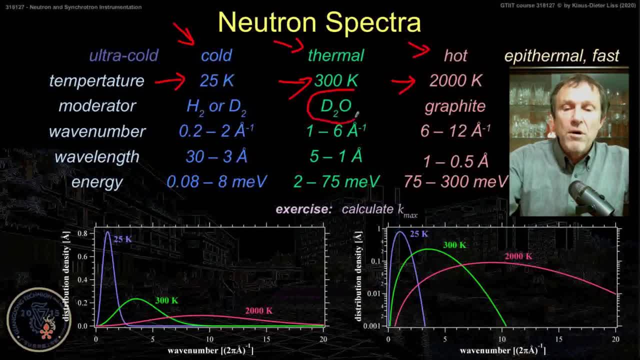 H. we take deuterium because hydrogen absorbs more neutrons than deuterium and the temperature is D2O. as we want to have more neutrons at the end, we want less absorption. so we take D2O for the moderation of thermal neutrons. 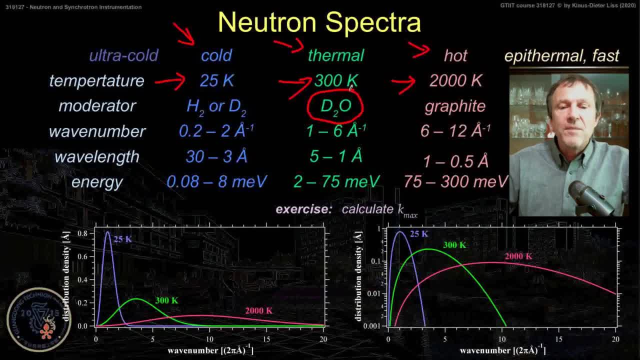 for the cold neutrons at 25 K we say we take liquid hydrogen or liquid deuterium. actually it's not liquid. it is a supercritical state where the gas and the liquid become one, where the gas and the liquid become one state of matter. so it has. 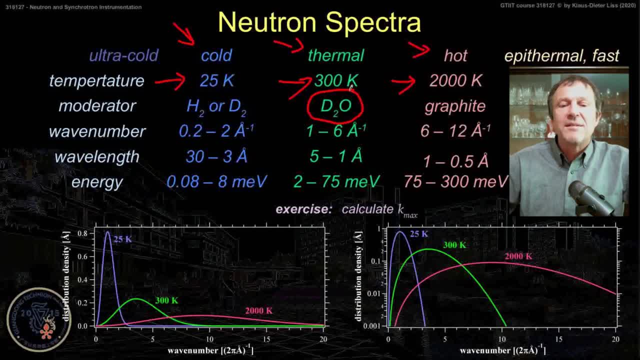 a density of a liquid, but it's half gas, half liquid. moderators for hot sources at 2000 K are typically graphite. you know, carbon graphite can glow at 2000 K, it's very stable and it can moderate the neutrons. hydrogen is not so suitable. 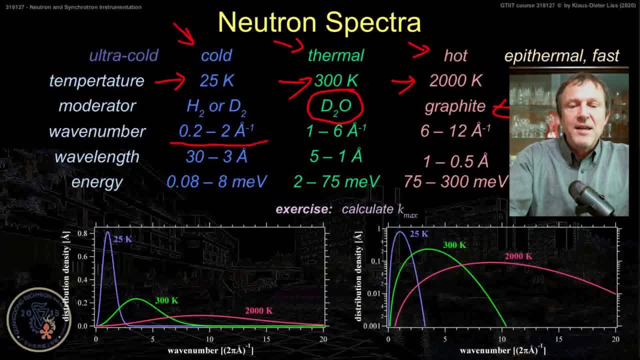 at those temperatures after moderation. the wave numbers are given here: 0.2, 0.3, 0.4, 0.5, 0.6, 0.7, 0.8, 0.9, 0.9, 0.10. 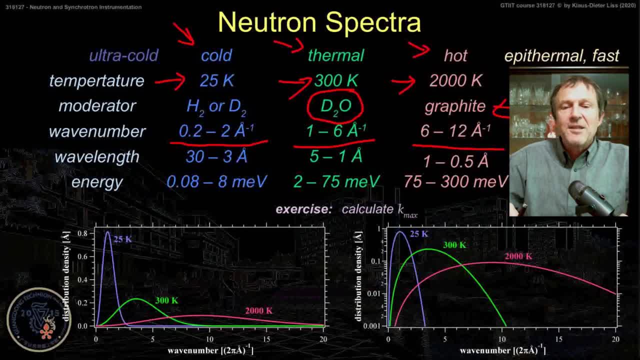 0.11, 0.12, 0.13, 0.14, 0.15, 0.16, 0.17, 0.18, 0.19, 0.21, 0.24, 0.25, 0.26. 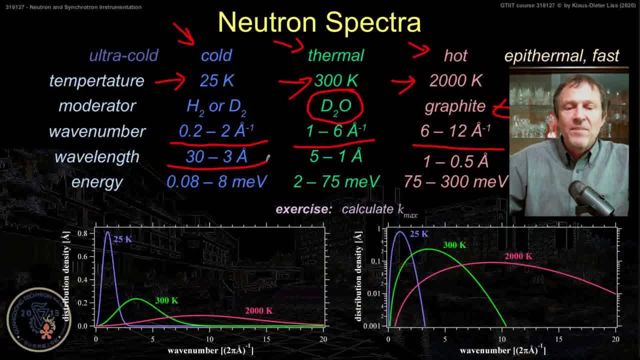 0.27, 0.30, 0.31, 0.33, 0.34, 0.35, 0.36, 0.37, 0.38, 0.39, 0.41, 0.42, 0.43. 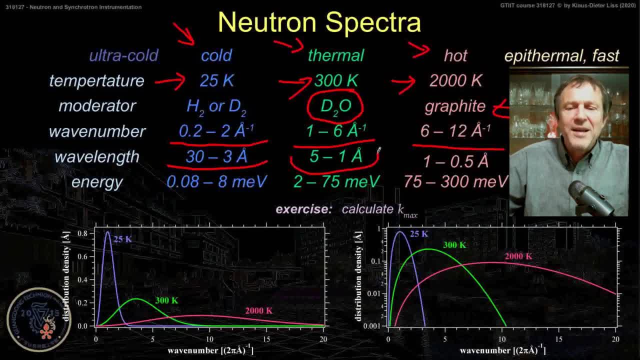 0.45, 0.46, 0.47, 0.49, 0.51, 0.52, 0.53, 0.54, 0.56, 0.57, 0.58, 0.59, 0.59. 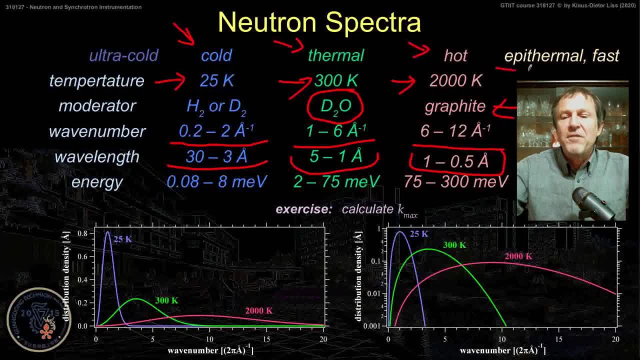 0.60, 0.61, 0.62, 0.63, 0.64, 0.65, 0.67, 0.68, 0.69, 0.70, 0.61, 0.72, 0.73. 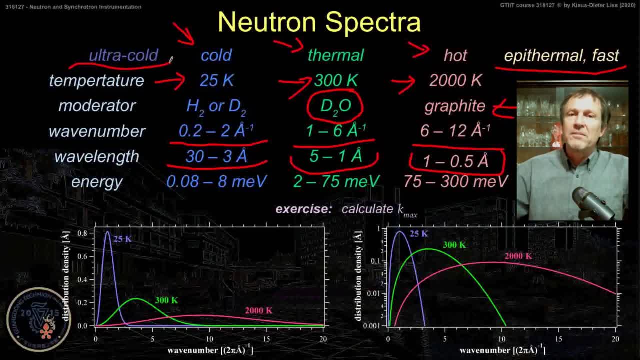 0.64, 0.63, 0.64, 0.64, 0.77, 0.77, 0.77, 0.77, 0.86, 0.87, 0.86, 0.98, 0.09. 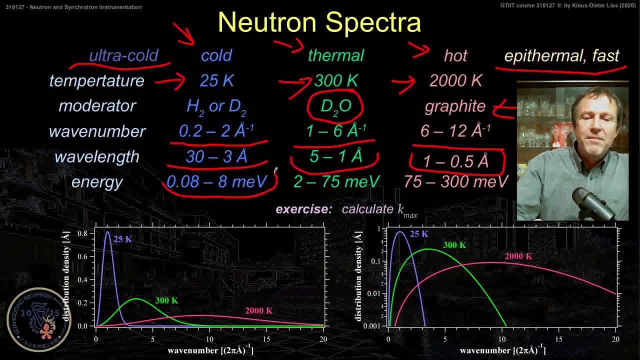 0.11, 0.12, 0.13, 0.14, 0.15, 0.16, 0.17, 0.19, 0.22, 0.23, 0.25, 0.26, 0.29. 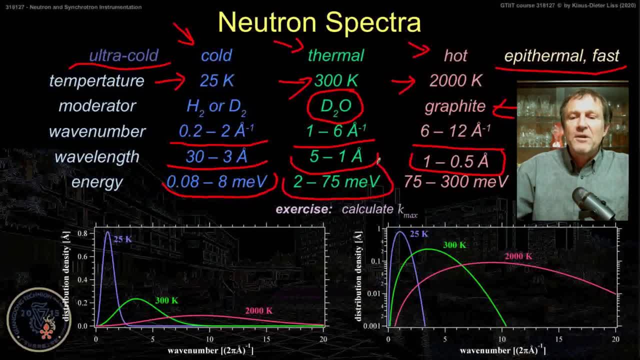 0.30, 0.31, 0.32, 0.33, 0.34, 0.35, 0.36, 0.37, 0.38, 0.39, 0.41, 0.42, 0.43. 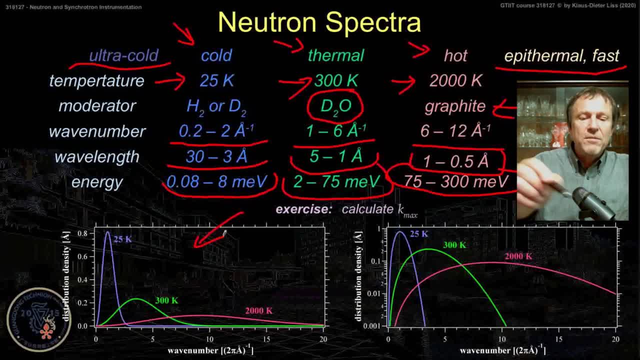 0.44, 0.45, 0.46, 0.47, 0.48, 0.49, 0.51, 0.52, 0.53, 0.53, 0.54, 0.56, 0.56. 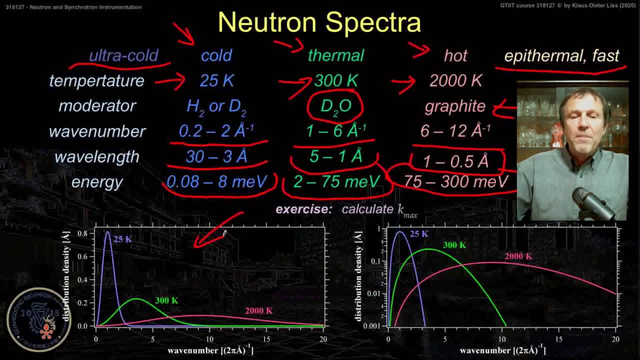 0.57, 0.57, 0.58, 0.59, 0.59, 0.59, 0.60, 0.61, 0.62, 0.62, 0.63, 0.64, 0.65. 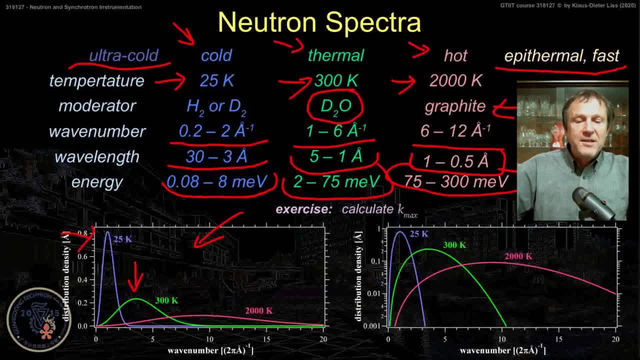 0.67, 0.68, 0.69, 0.69, 0.70, 0.61, 0.72, 0.73, 0.64, 0.67, 0.68, 0.69, 0.72. 0.73, 0.74, 0.74, 0.75, 0.78, 0.69, 0.71, 0.72, 0.72, 0.72, 0.73, 0.74, 0.75. 0.78, 0.74, 0.78, 0.75, 0.46, 0.74, 0.65, 0.76, 0.78, 0.76, 0.78, 0.78, 0.78. 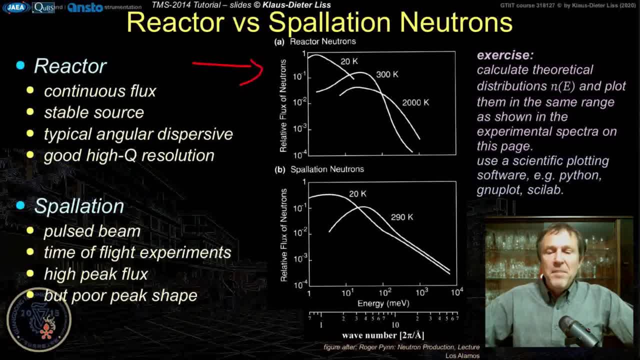 0.91, 0.92, 0.21, 0.24, 0.23, 0.24, 0.25, 0.25, 0.26, and for 2,000 kV, so not following exactly the Maxwellian distribution. 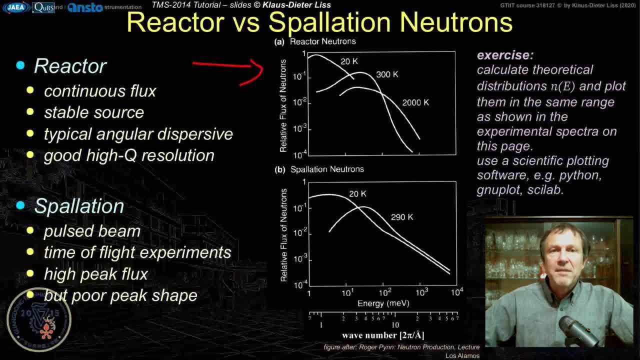 this is because there may be other scattering processes occurring and the moderation thickness may not be enough. We learned about cross-section and attenuation lengths, so you have to have at least an attenuation length for full moderation. Moreover, the reactor sources: they fall down pretty much at the higher energies. 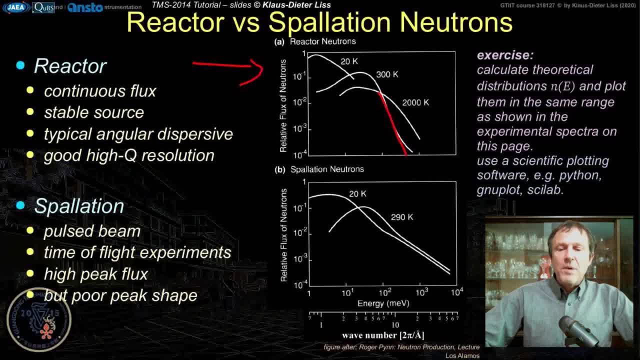 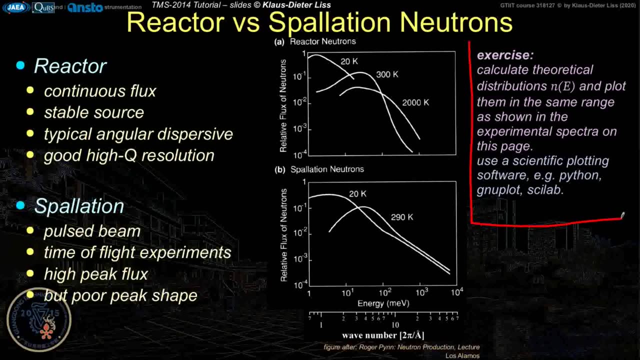 at the higher k vectors, while for spallation sources you have a longer tail of transmitted epithermal and fast neutrons. At this stage, I'd like to give you another exercise, which is written here, namely calculate the theoretical distributions N of E. 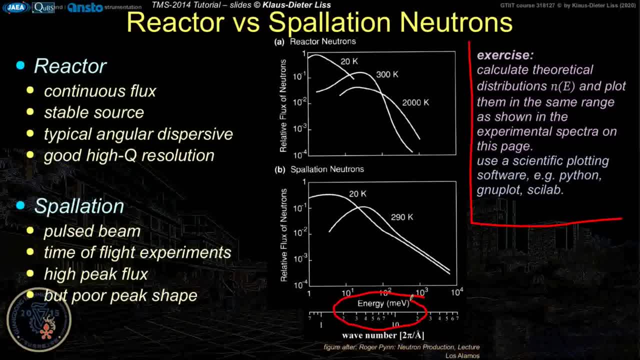 so here we have the energy on the plot and plot them in the same range as shown in the experimental spectra on this page. Actually, we have these diagrams which are experimental data, and I want you to add the theoretical curves for the Boltzmann-Maxwell distribution. 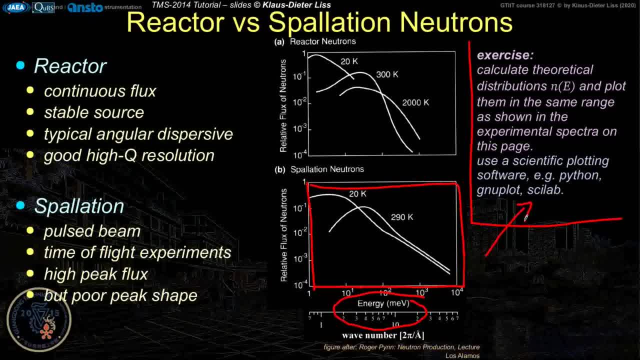 You should use a scientific plotting software, eg Python, Gnuplot, Scilab, And for the very good of you, you even can scan the experimental data. so you can scan the dot dot, dot, dot, dot, dot dot by a software which is called X-Y-Scan. 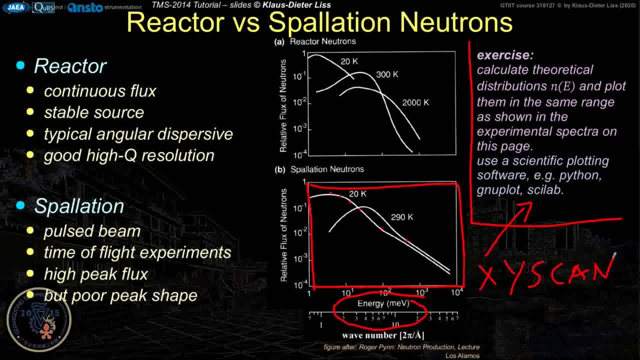 This is extended homework where you need a computer, kind of a computer lab, but it may be very useful for your academic career. When you write papers, you have to make presentations, you have to make plots and sometimes you also have to incorporate data. 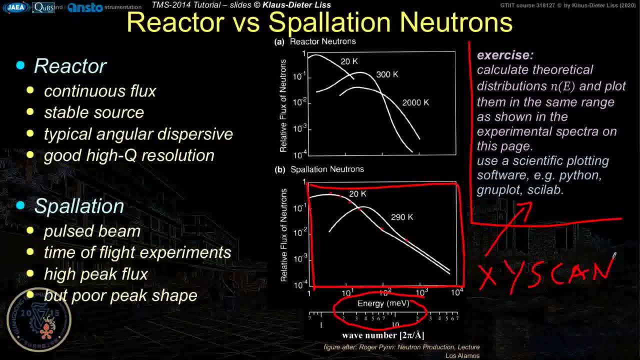 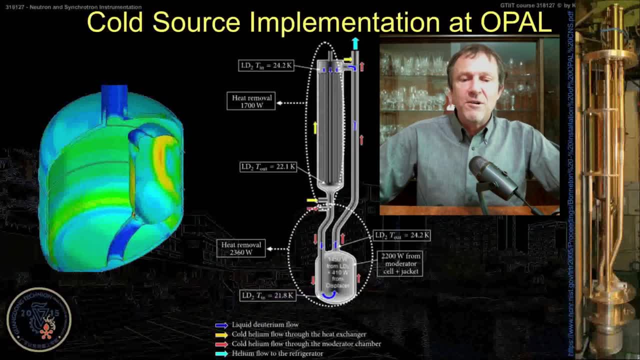 You have to integrate old data and you have to discuss experimental data with theoretical data. The cold source implementation at OPRA looks a bit like this, So this is an instrumentation lecture. We have a volume, which is cold, of cold gas. 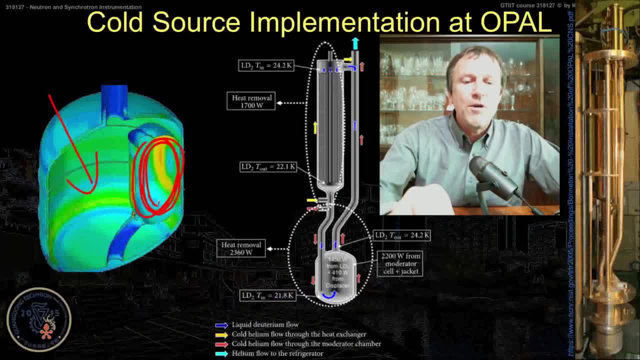 I think it's helium there and here we have the D2O in this volume. It streams in And it streams out, And neutrons, they may enter through the whole volume Fast. neutrons enter through the whole volume into the moderation volume. 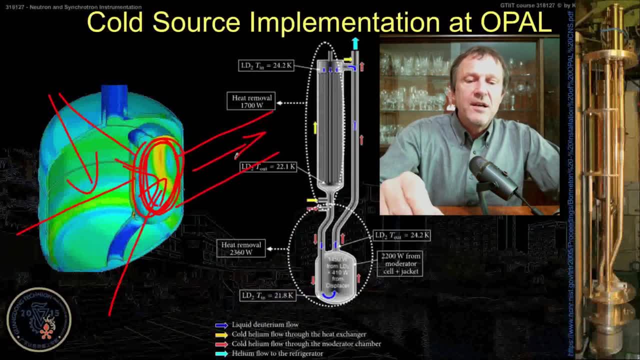 and behind we have a neutron guide into which the neutrons can escape and be guided to the instruments. More technical details is here. So we see that we have here liquid deuterium temperature. leaving The deuterium temperature is 24.2 Kelvin. 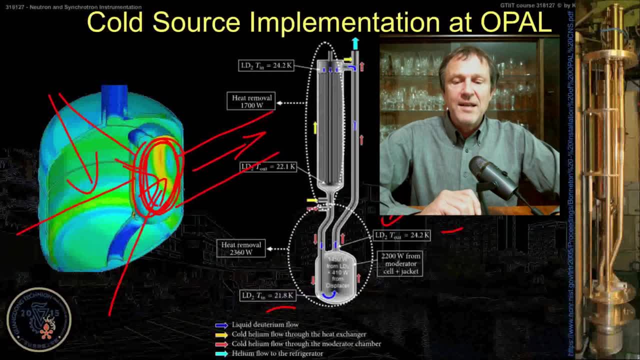 Incoming temperature is 21.8 Kelvin, So it gets heated up. There's a lot of heat removal, So we have 1700 watts dissipation here by that heat exchanger. Of course, this volume, this very cold temperature, is very close to the nuclear reactor. 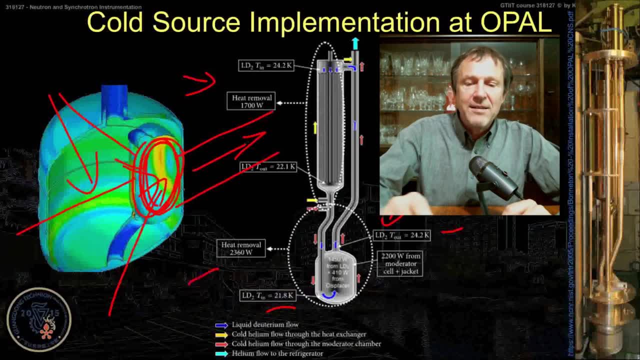 So it gets heated by a few kilowatts. Heat removal is 2316 watts. 2316 watts just towards the surroundings of the source, But then the gas itself gets heated as well. So we need a heat exchanger which removes another 1700 watts. 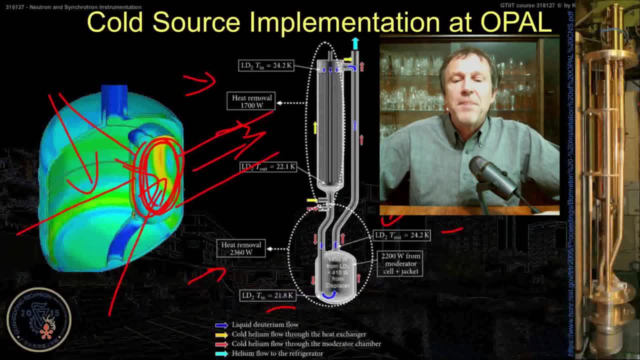 Altogether we have 4 kilowatt energy dissipation in this volume, which is a very high requirement to the fridge, to the cooling system, in order to keep it stationary. A nice picture of the moderator and the pipe system is given here, to the right. 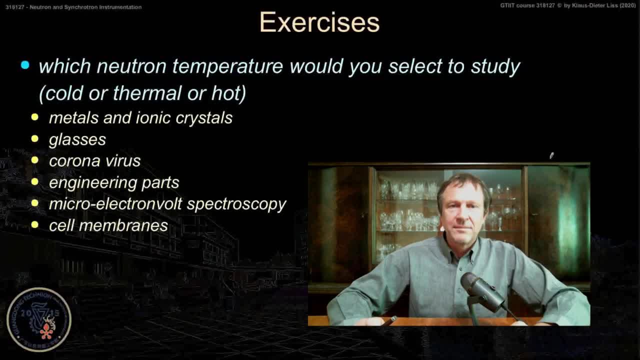 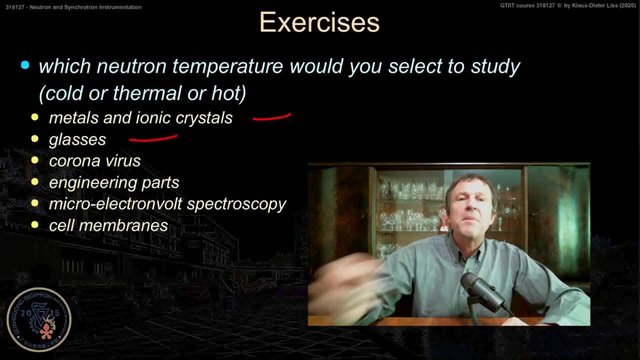 You can look it up here under this link. A few more exercises: Which Newton temperature would you select to study Metals and ionic crystals Glasses? So it can be metallic glasses, It can be oxide glasses. The coronavirus Engineering parts. 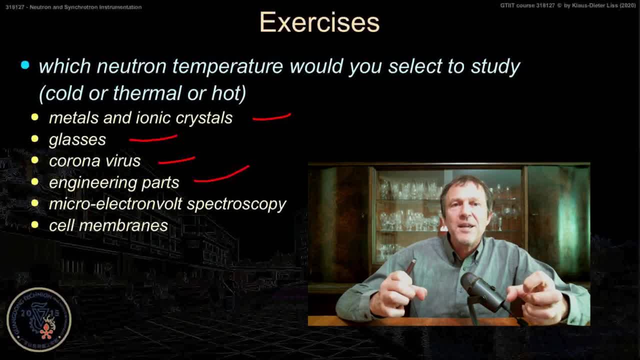 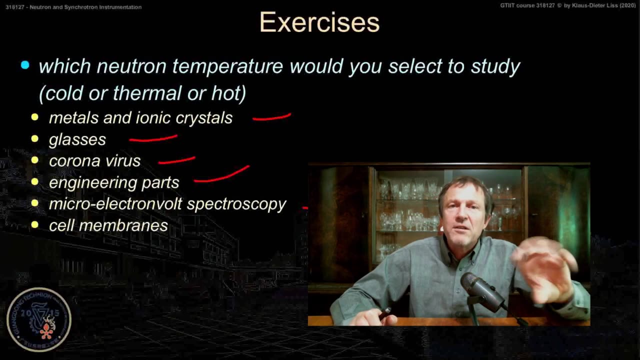 So I'm talking about bending a steel beam and measuring the stresses. Microelectron volt spectroscopy, So very high resolution, low energy. spectroscopy in a rotating tunneling group Or cell membranes. Phase transformation in cell membranes in vesicles, lipids. 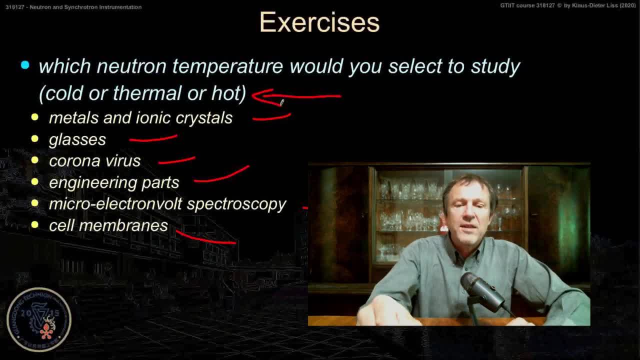 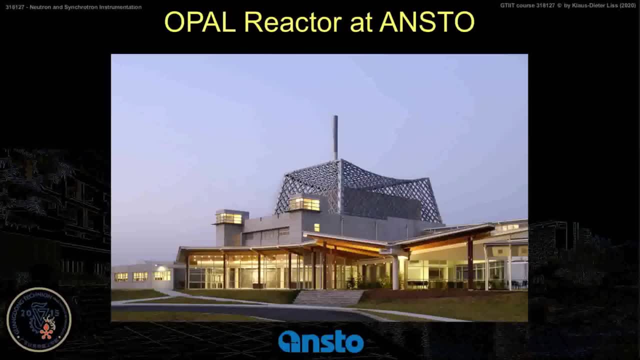 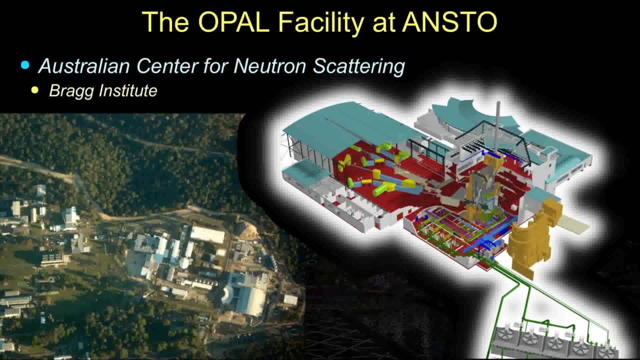 Think about it and tell me whether it's better to use cold thermal or hot neutrons. Now we will have a tour through the Opel reactor at ANSTO. I've shown you already a lot of pictures, but we also want to go through the instrumentation. 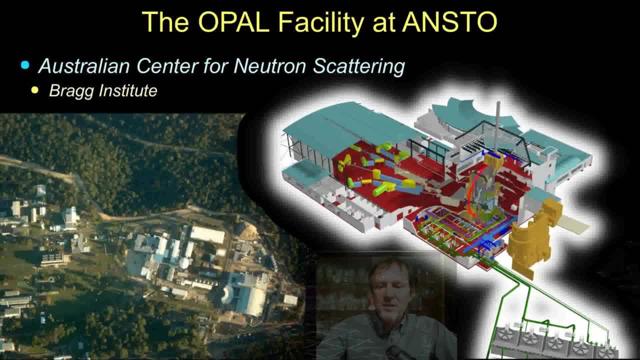 The Opel facility consists of a reactor, So we have the nuclear reactor here, But then we have these neutron guides and we have instruments. We have neutron spectrometers and diffraction instruments away from the reactor and also surrounding the reactor. This is called a neutron guide hall. 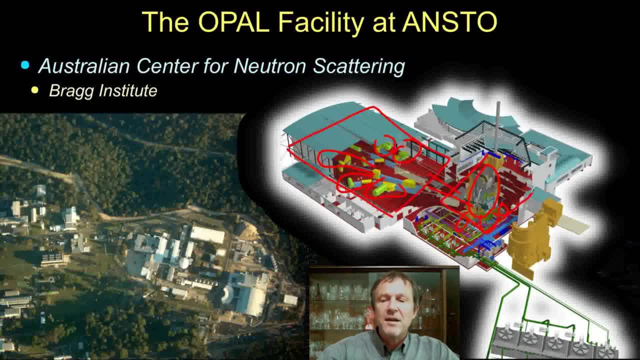 This is called a reactor, building The reactor core And of course there are annex buildings, Pump stations, heat exchangers and so on. A picture which I took from the plane flying over Sydney. Some people take the Harbour Bridge, I take this. 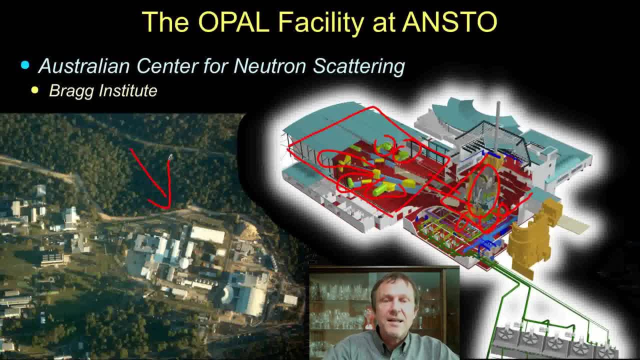 This is part of ANSTO. at Lucas Heights, south of Sydney, We have the old reactor, So this was the HIFAR reactor, And we have the reactor building of this new reactor, Opel, And here to the south we see the neutron guide hall. 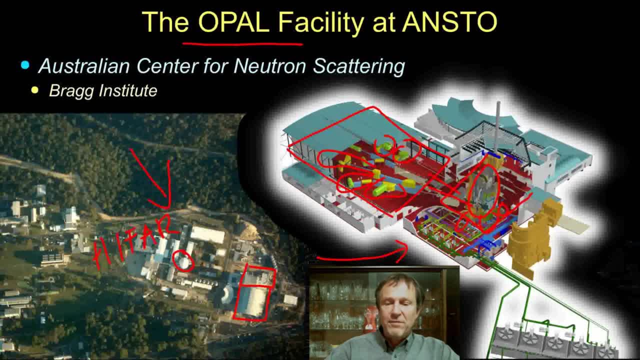 So the sketch is rotated a little bit with respect to the photograph. Here you see cooling towers, So these are the cooling aggregates for the reactor. There's a lot of heat dissipation which are shown here, And around there's a nice national park. 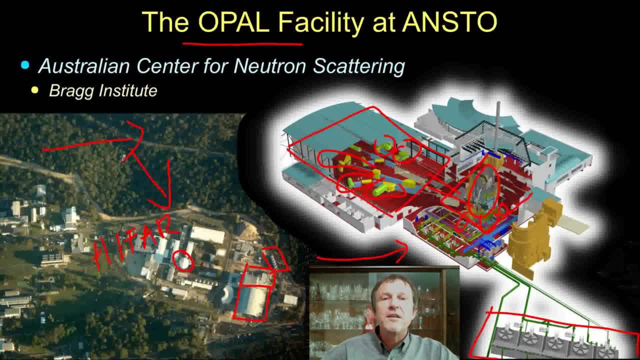 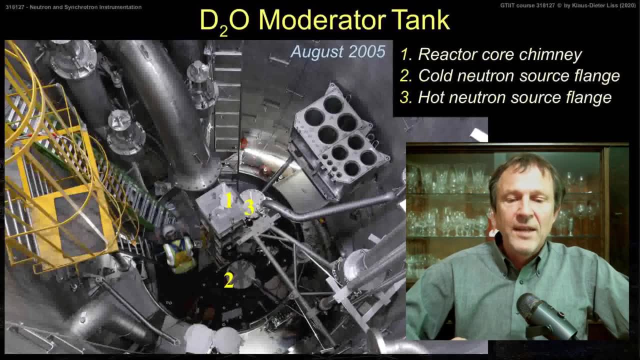 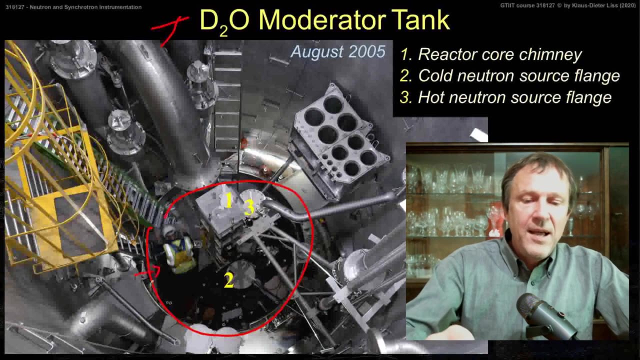 So there's nice bushland Australian Bush National Park. There's a Heathcote National Park just behind, Behind this road, There's a look into the D2OO moderator tank. So the tank is here. It looks open. 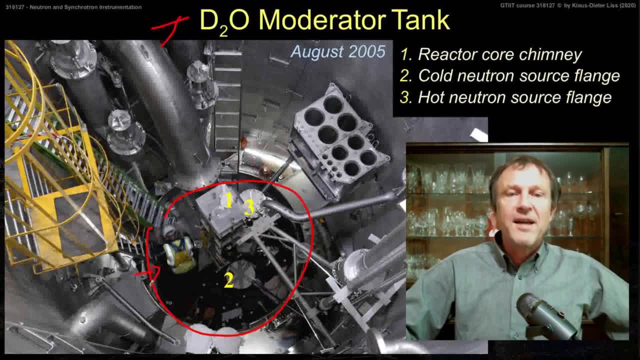 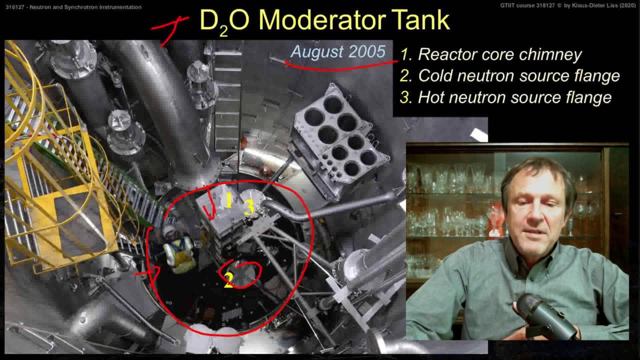 Some person working here. This is at the installation of the reactor, So it was built in 2005.. You see the reactor core chimney. This is for the cooling. We see the flange for the cold neutron source And we see a flange for the hot neutron source. 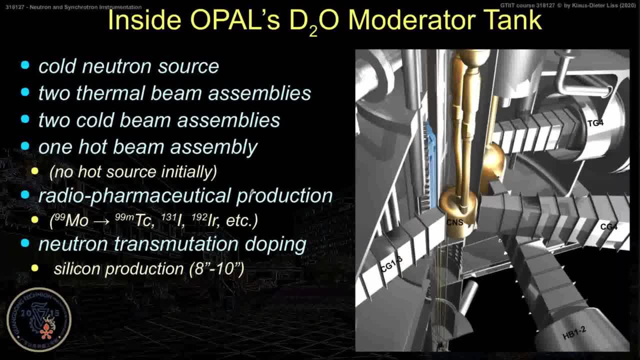 However, the hot neutron source is not yet implemented Inside the D2OO moderator tank. Again, we have the cold neutron source, CNS, Which points to this cold guide number 1 and 3.. And the cold guide number 4.. There are the thermal guides TG4.. 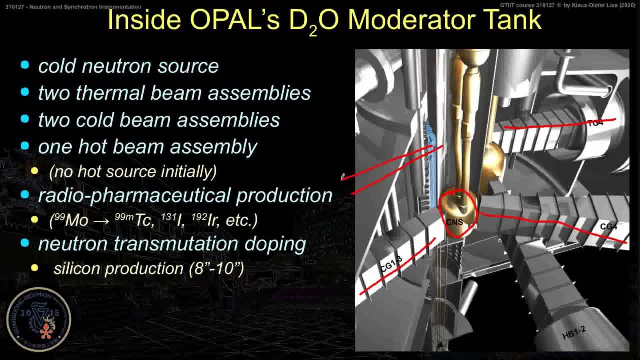 And there are thermal guides to the other side Which you cannot see here: 1 and 3.. So these cold guides, We call two cold beam assemblies, One hot beam assembly, Pointing here, As mentioned, at the moment there's no hot source. 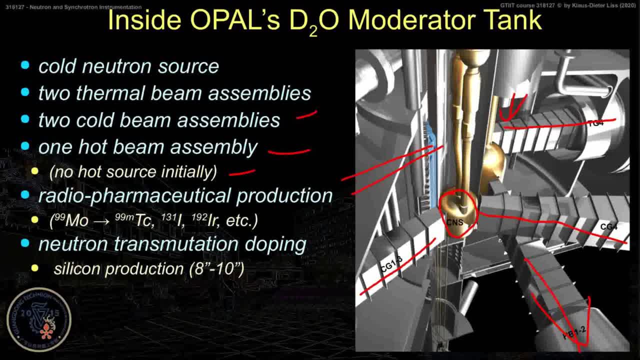 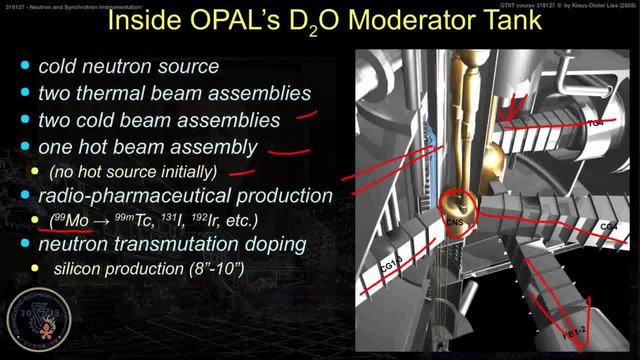 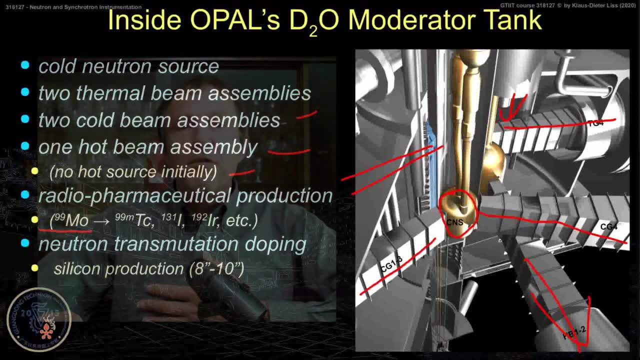 And there are other pipes and inlets For radiopharmaceutical production Where they produce Moly 99. Which decays to technetium 99. This is a radioactive tracer method In nuclear imaging of the body In medicine. There may be other isotopes- Iodine 131 is a famous one. And last not least, The inserts for neutron transmutation doping, Where you have whole big silicon wafers. They are put in a nuclear beam. The silicon may catch some neutron. 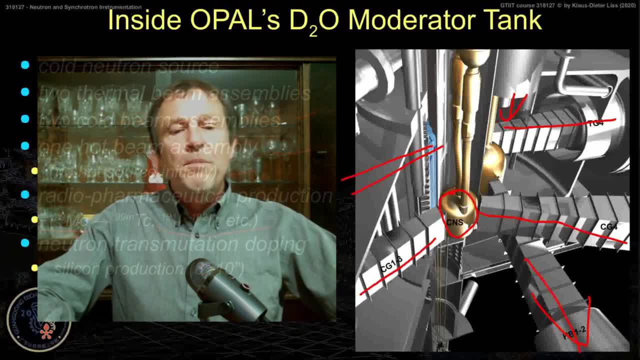 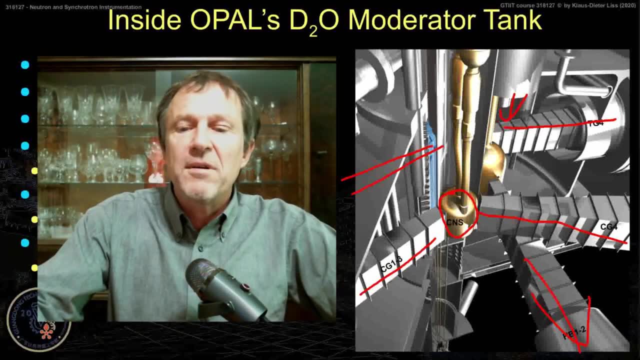 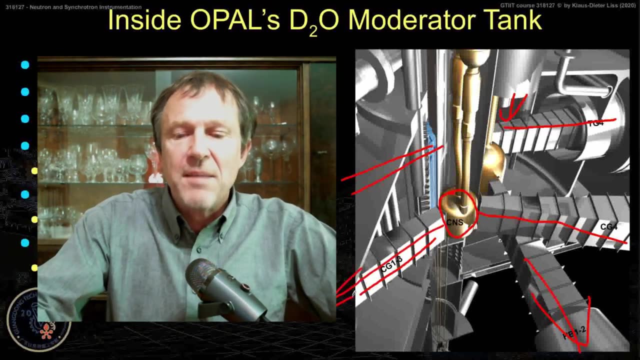 And undergo some nuclear reaction To produce doped silicon For the semiconductor industry. In the following slide I show you a movie: What happens to the neutrons When they escape from the cold source Into this neutron guide, Cold guide number 3.. 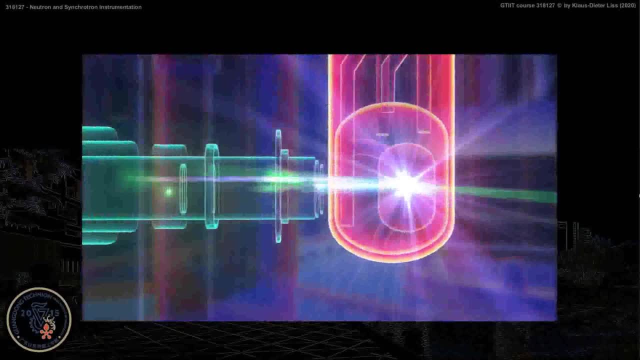 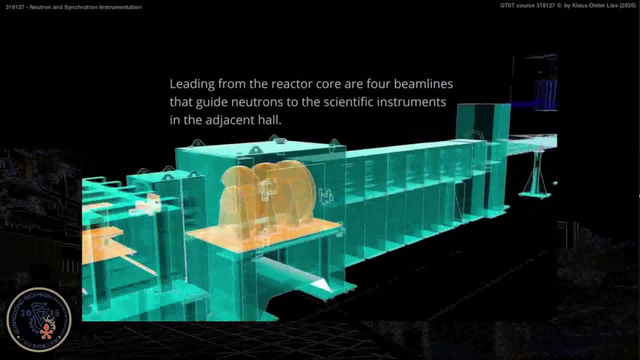 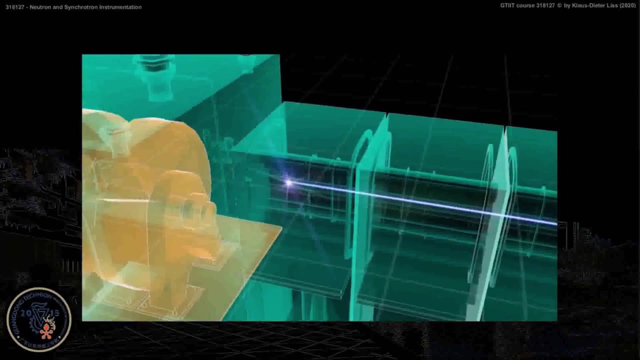 We have here the reactor Leaving neutron Cold source. Now it goes through the guide Quite far away from the source, Into the instruments Which consist of a chopper. So rotating wheels Will divide the continuous beam Into bunches of beams. 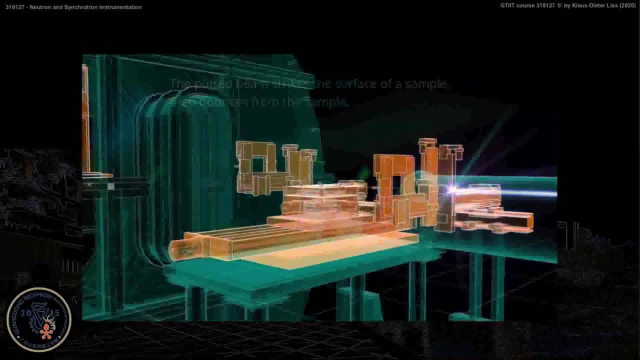 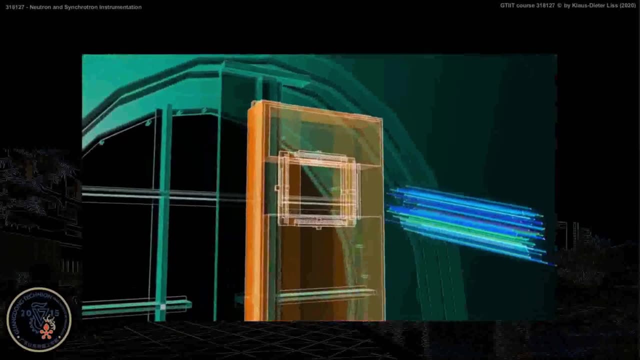 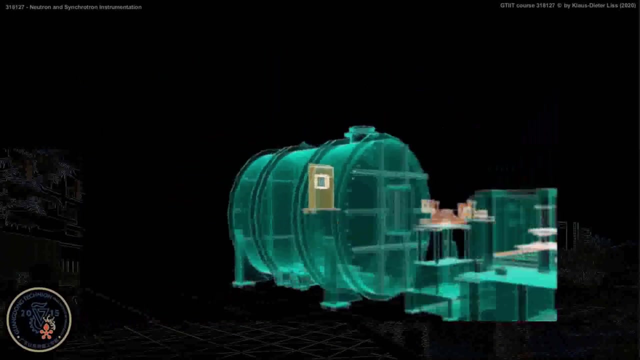 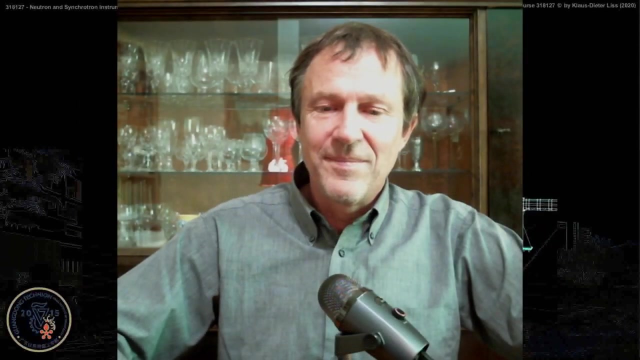 So you get a time structure, Then it will hit a sample here, The horizontal table, And scatter into a detector Where you record neutron diffractograms And make users happy. What we have seen was the escape. So production of the neutrons. 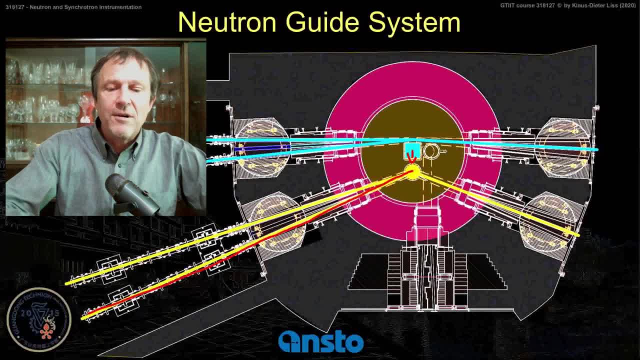 Hitting the cold source And then going along this guide And eventually going towards the instruments Here schematically shown: The neutron guide system. Actually, there is one more guide Now. there are three guides going out. This is an old display. 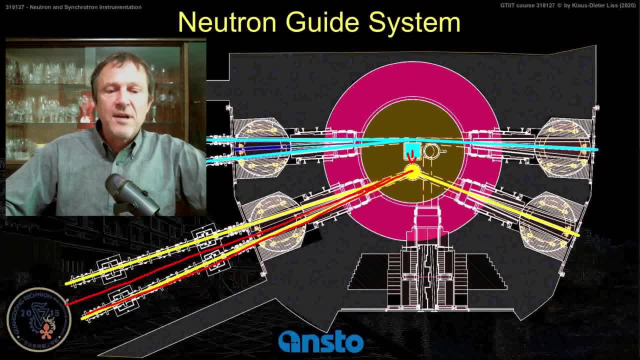 Meanwhile, more instruments have been Installed in the neutron guide hole, So there are three cold guides going out And two thermal guides Into the neutron guide hole To the left, While on the right hand side We directly have instruments here Also, instead of having the hot source. 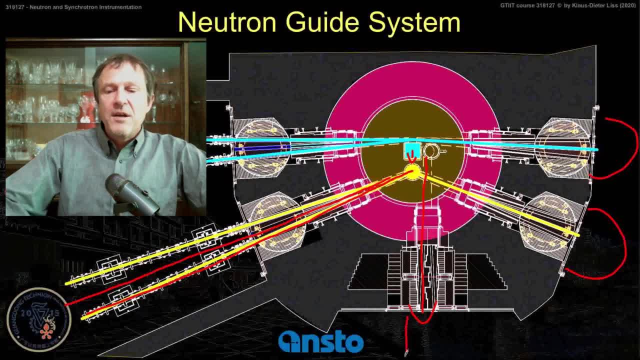 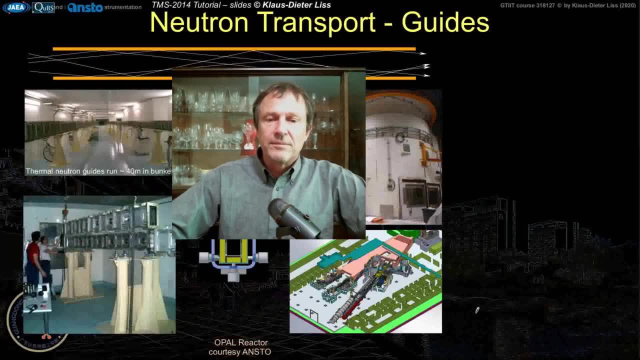 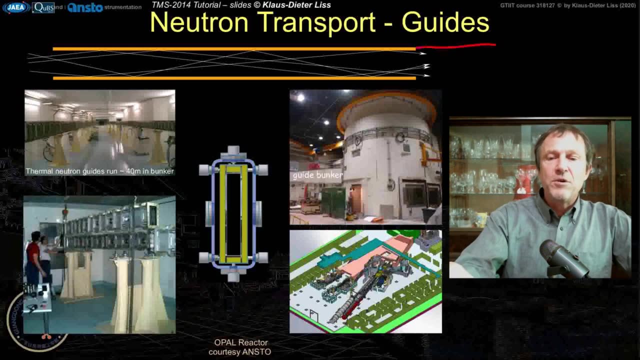 We have another direct Thermal neutron beam going here To another station, Which is the imaging station Called Dingo. What are neutron guides? Neutron guides are just reflecting mirrors. So we have two mirrors here, And neutrons that come in get reflected. 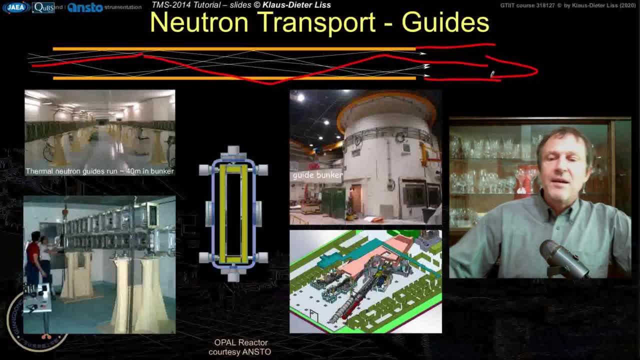 Up and down And so Can be guided away from the source To the target, To the instrument, These neutron guides. They can be several: 10, 20,, 30,, 40,, 50 meters long, As shown here. 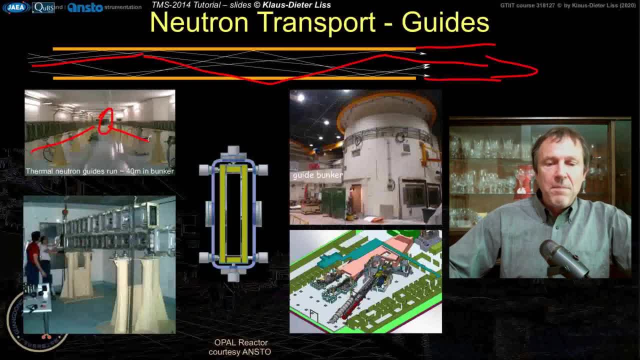 So there are two guide sections. They are pieces of glass. They need a very accurate alignment. The reactor core is shown here. That was in early stages, When there is not much instruments around And the guides, They would go here behind. 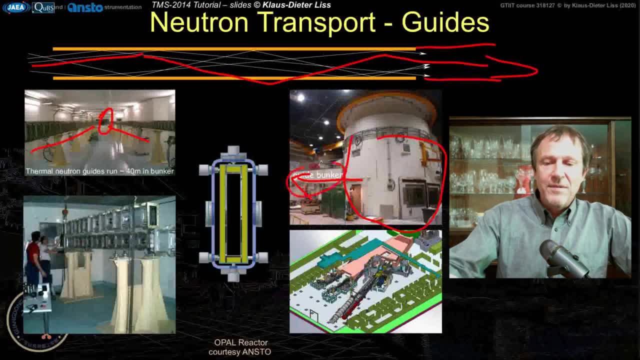 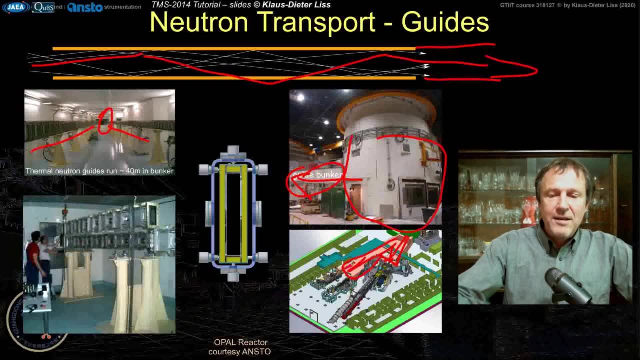 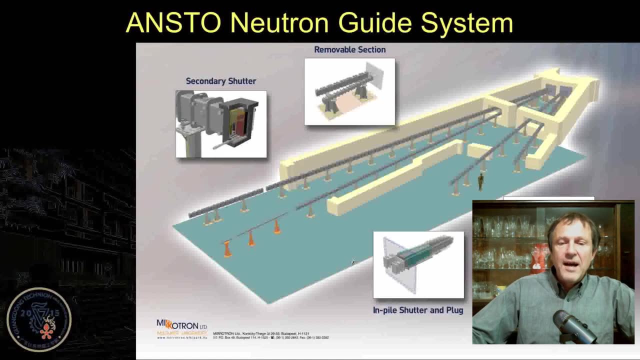 In this guide bunker To the instrument. So we are talking- the guide bunker- Is this orange thing here In the overall view- And guiding neutrons To the instruments, The neutron guides At ANSTAL. They are made by Mirotron company. 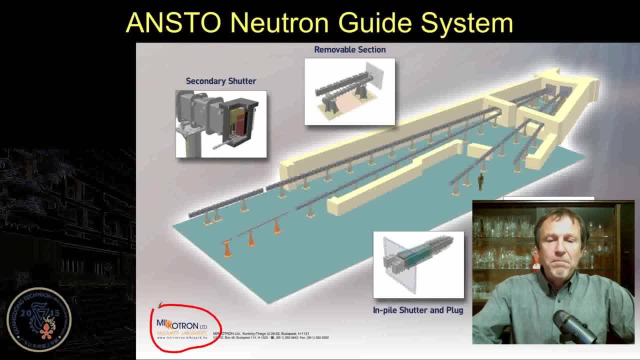 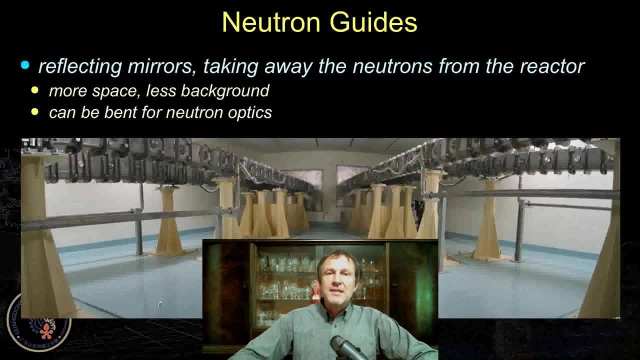 In Romania. They came out to install them. This is from their web pages. Repeating what I said, With another nice picture, They look like this. Actually, they are a little bit bent Because you don't want to see directly into the neutron source. 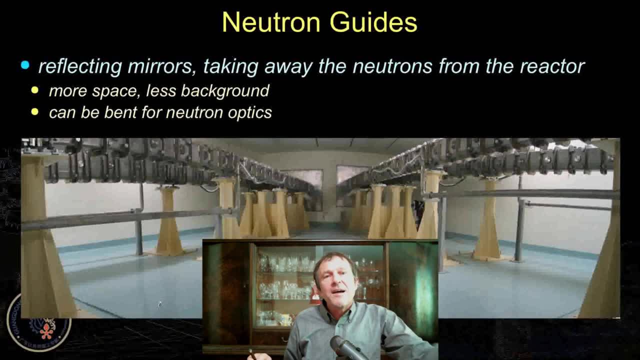 You don't want to see directly into the reactor Because there would be other Radiation coming down as well, Such as the very fast Unmoderated neutrons Or the gamma radiations, Which are not reflected by the guides. So if you bend the guides, 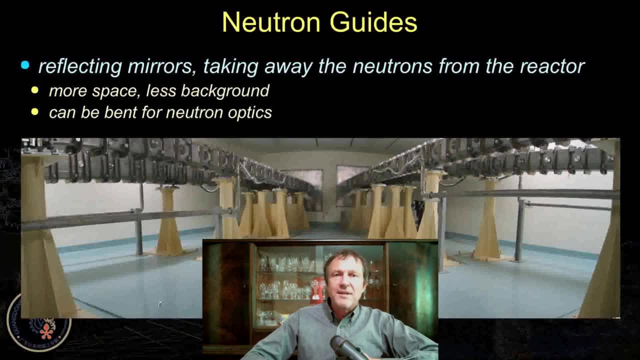 Gently. Then you get rid of this unwanted radiation And the nice neutrons, The moderated neutrons That are in the instrument, Giving you there less background And generally. I talked about bending, So nowadays the mirrors, They don't need to be flat. 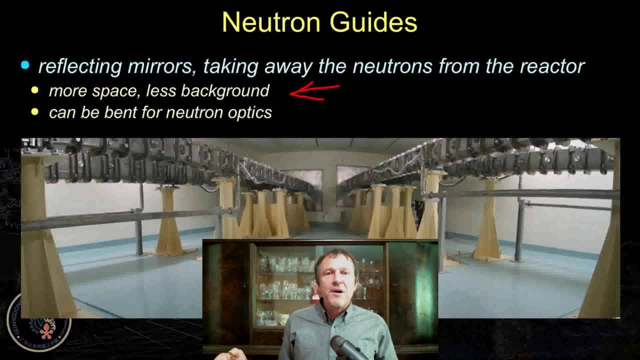 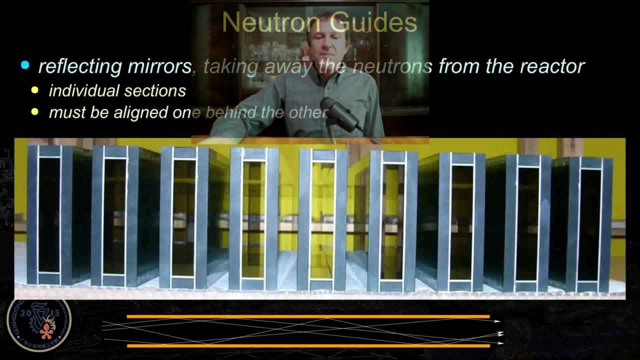 They can be bent on hyperbola, On parabola, To give you some neutron optics And to have some focusing Devices for the instrumentation. This is how they look like, So they are reflecting mirrors, The neutrons from the reactor. 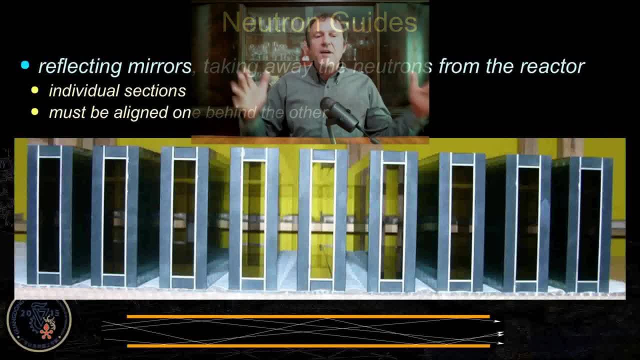 The individual sections of 50 cm length And you have to line them up One behind the other And the critical angle of reflection Is very small- It's maybe just one or two degrees. So you have to align them in displacement. 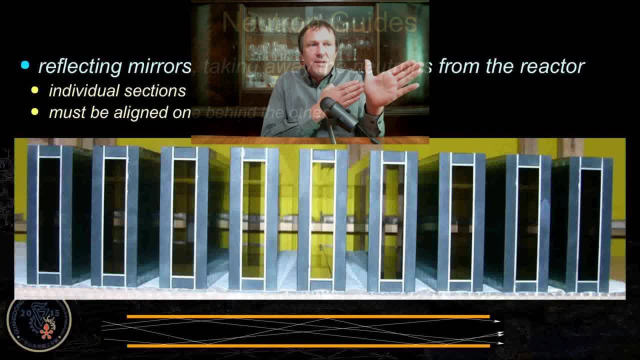 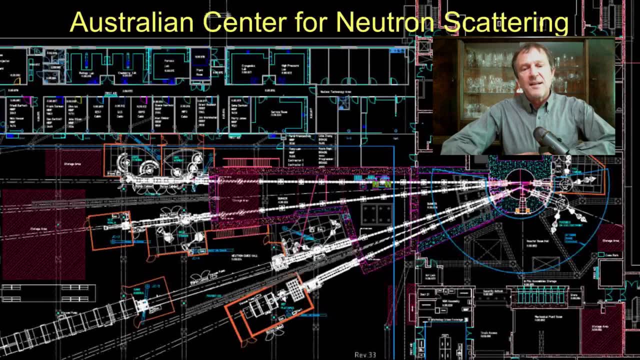 Just within a few micrometers, And then also in the angle, Within a few arc seconds. This leads to the Australian Centre for Neutron Scattering, The former Bragg Institute. We have again, For orientation, the reactor source. And now 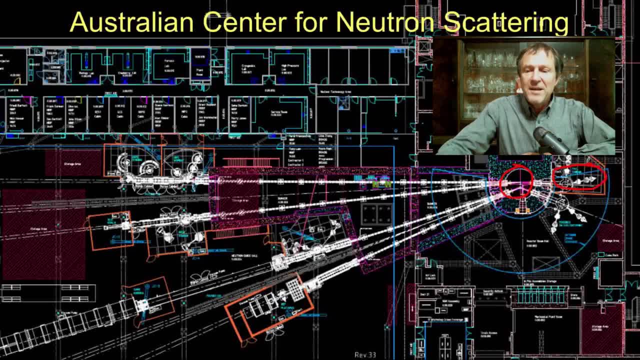 I quickly talk through the instruments. So we have spectrometers here. We have two Triple axis spectrometers Where you can analyze the energy Of the scattered neutrons. In contrast to diffraction, Diffraction takes place here. So we have the Wombat diffractometer. 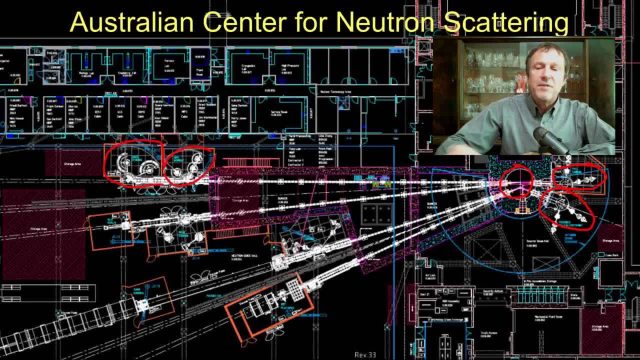 We have the Echidna diffractometer, Which I bear. We have a strain scanner, Which also is a diffractometer. Then we have small angle Neutron scattering here. This is for small momentum transfers. There is a second one now. 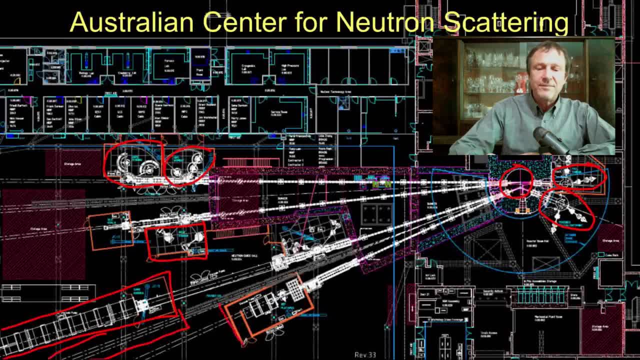 Which is not shown here on this sketch. We have the reflectometer. We have an ultra small Angle scattering here now Which is not shown, And there is a second reflectometer Called Spatz. now There is an inelastic Neutron spectrometer. 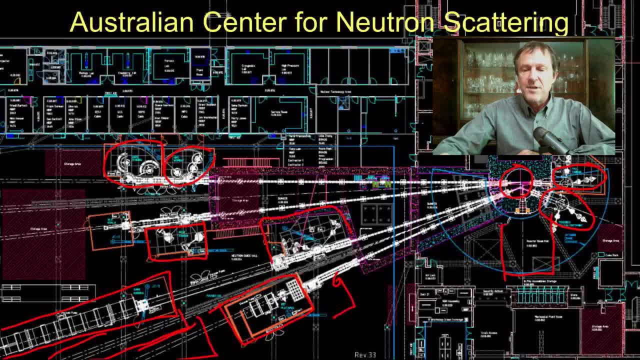 And there is an imaging station, Which I mentioned Already before, For radiography. Last not least, There are two wide beam diffractometers For single crystals For lower diffraction, The Koala and the Joy, Initially in 2005.. 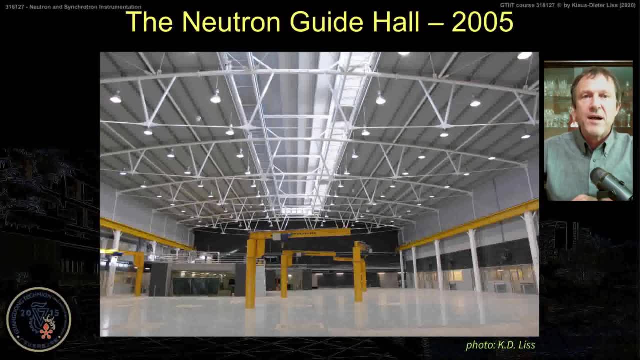 The neutron guide hole Looked like this, Actually, when I arrived there in 2004.. There was still a rock bed, A deep hole down to the rock bed Which has been filled with solid concrete For stability of the instruments. They are maybe very heavy. 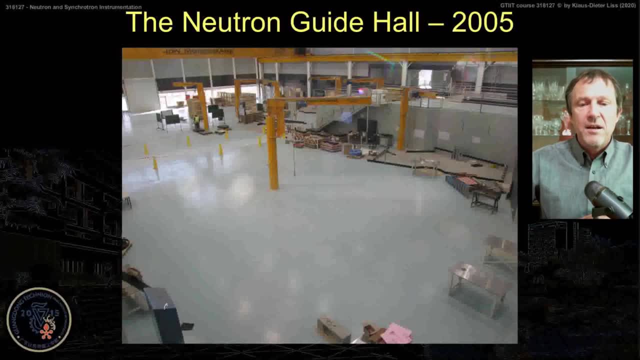 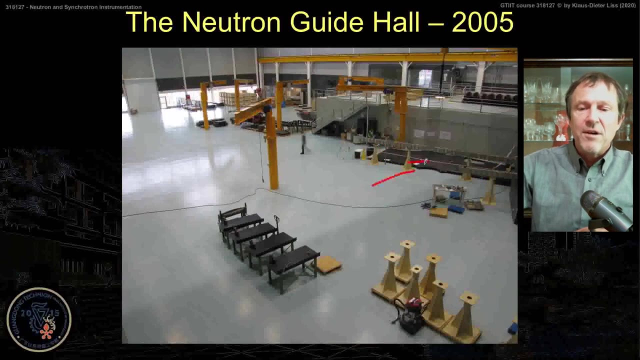 The shielding is very heavy, As you will see, Initially it fills up 2005. later We get boxes and tables in, We get frames here Where we build the instruments, Where we build the dance floor of the instruments. Now you see, 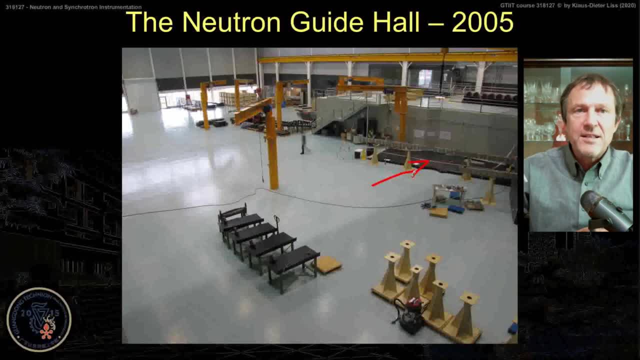 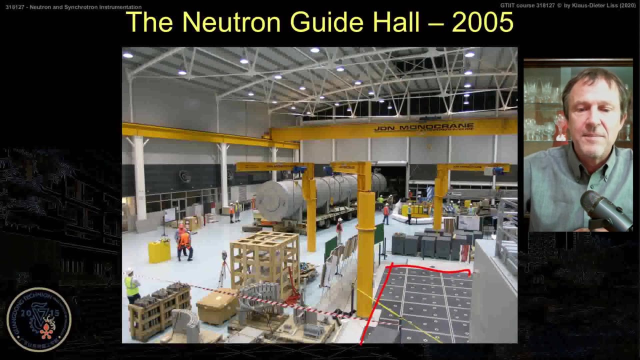 There are already tiles of granite lying. On these granite plates We put the instruments And with air pressure We can lift them up And move tons of equipment Easily over this air cushion. There is another Dance floor coming here, The small angle scattering. 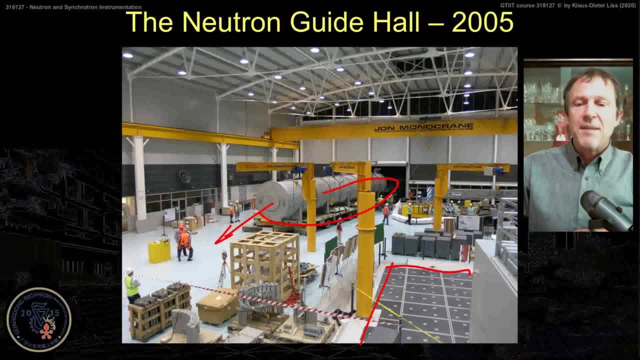 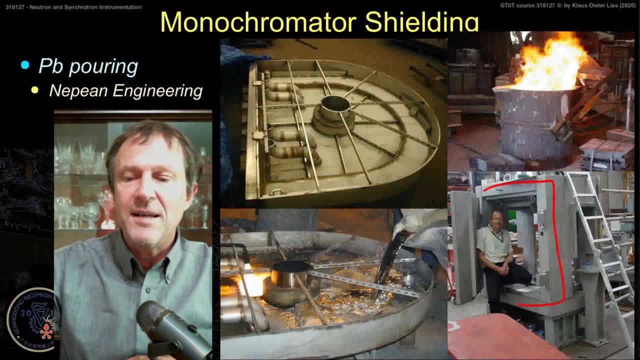 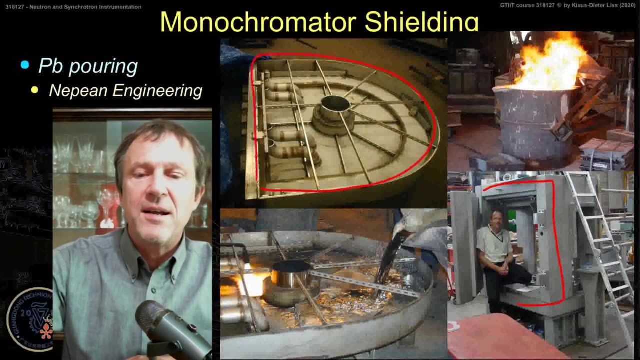 Tank- This is a detector tank- Is coming in through the door. here We had to build Heavy shielding, So here I am, sitting in the shielding At the company, At the Nippin engineering company, Which is a lot of lead. 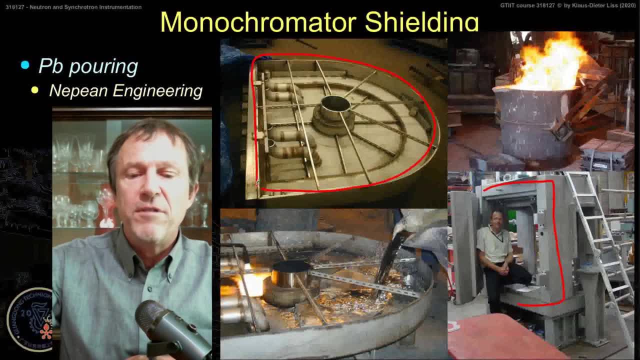 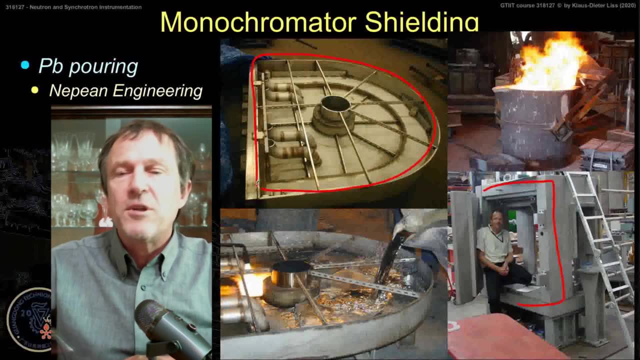 So first you have to design All the structure to hold the lead, Which is stainless steel, And then you fill it with lead And then you need Some neutron absorber Which is not lead. So lead is transparent for neutrons. 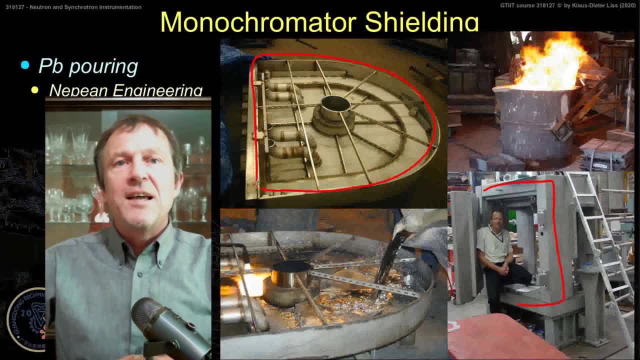 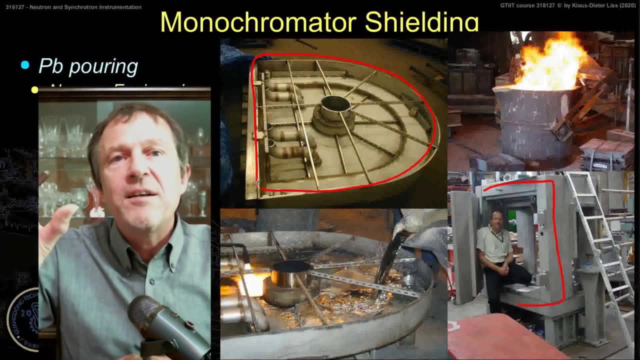 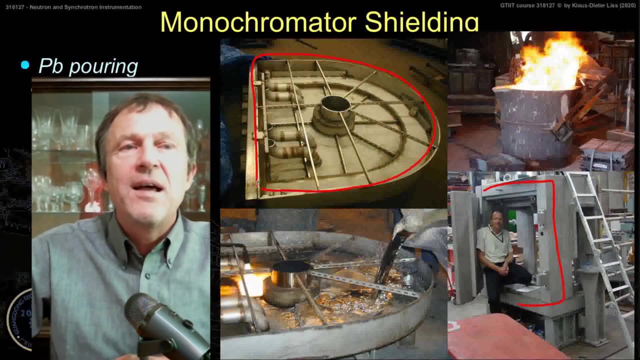 But fortunately we have hydrogen. I mentioned already, hydrogen Is a neutron absorber. So we put inside the lead, We line it with thick layers Of paraffine, Paraffine wax, Which you have in a candle Containing a lot of hydrogen. 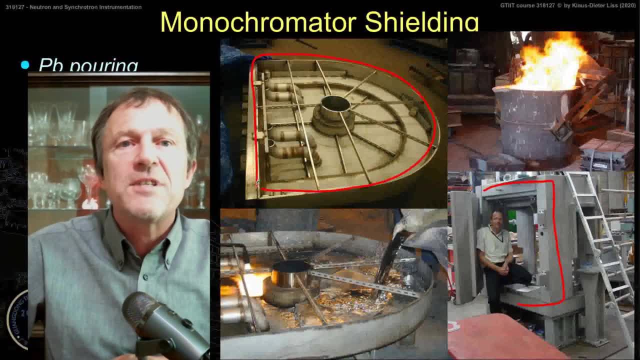 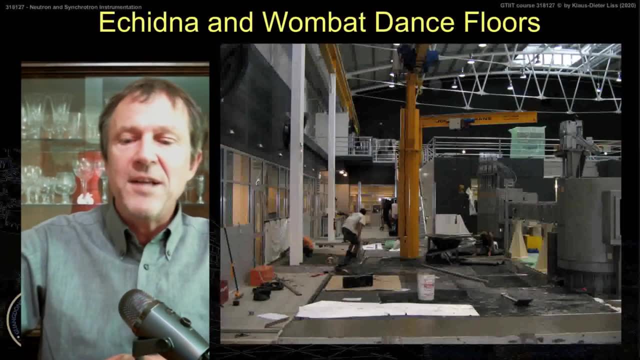 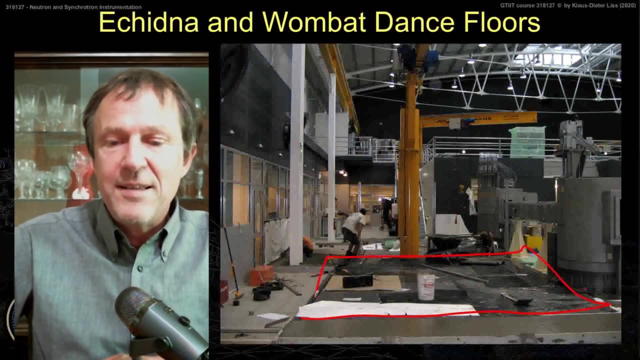 And this hydrogen Can absorb the neutrons, They produce gamma radiation, And this gamma radiation Then has to be shielded by the lead. Dance floor has been mentioned, So here is the implementation Of the dance floor, of the instrument Which I built here. 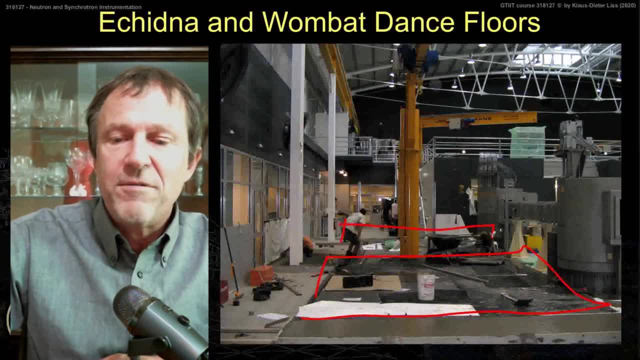 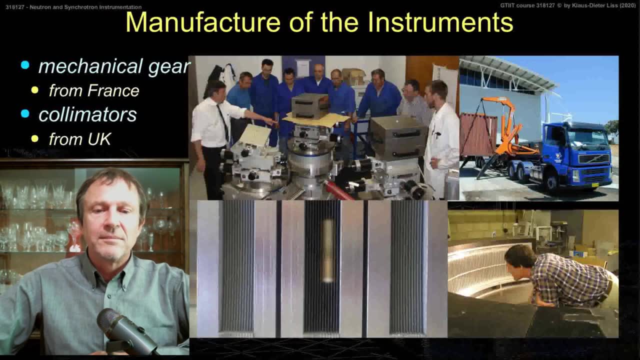 It is the echidna instrument Powder diffractometer, And behind there is the sister powder diffractometer, The wombat, Which I also used to be a beamline scientist on The instruments Which have been designed And manufactured by us. 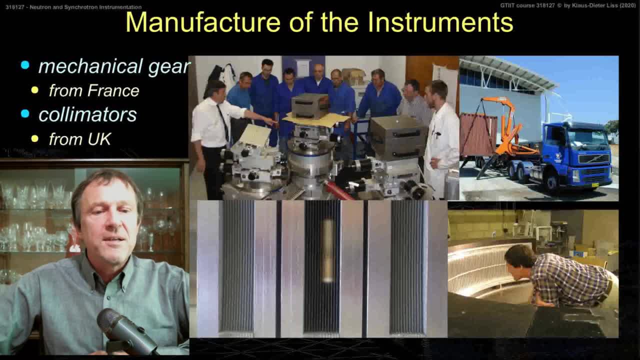 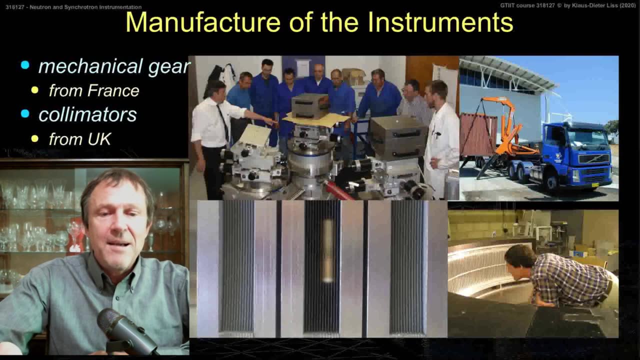 We have taken expertise From all over the world. So mechanical gear Has been built in France Near Grenoble. You know, in Grenoble There is a large neutron facility, The Institut Laurent Langevin, Where I did my PhD, And a company nearby. 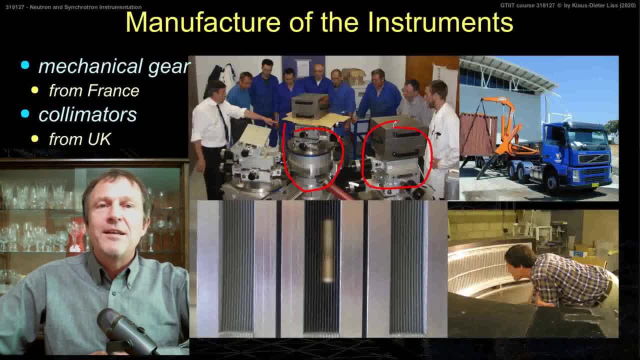 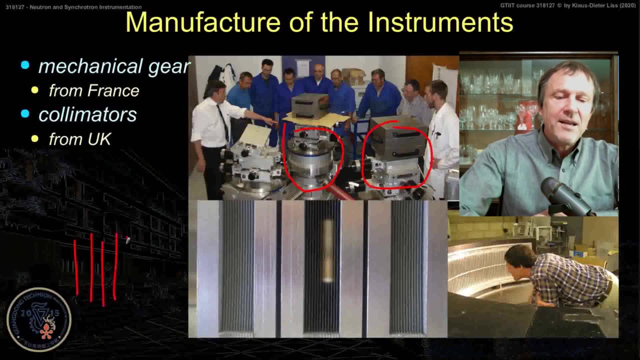 Produced the mechanical gears, So the towers. I had the opportunity In Australia For inspection And for factory acceptance tests And the same collimators. Collimators is When you look into A stack of absorbing plates, When you look in. 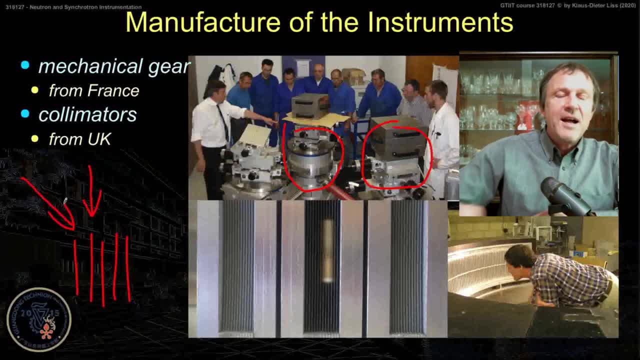 In the longitudinal direction You can look through. But if you look into it sideways You can not look through Because the absorber is in the way And that allows To accept neutrons From a very small, Narrow angular direction. 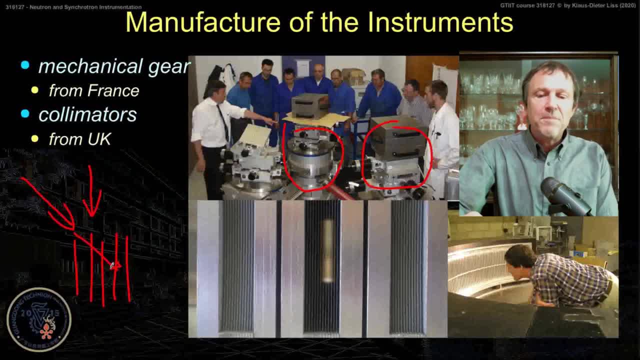 What we see here When we look through it optically. You see, here Is the transmission And here from the camera, Or from my eye, The angle is too big already So I cannot look through. You can do that experiment. 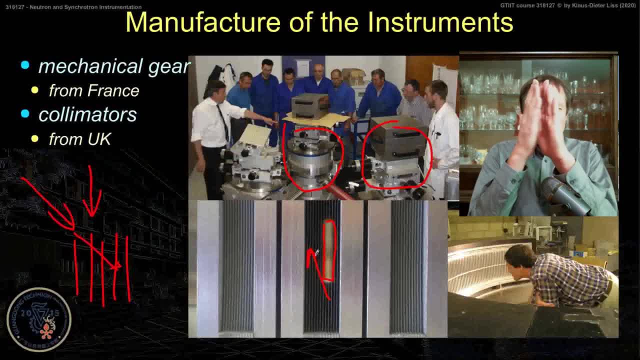 Just by putting the hands like this, And if you incline them You cannot look through. So this is called a collimator. In this case it is a solar collimator. Here I am In the UK, A little bit outside Oxford. 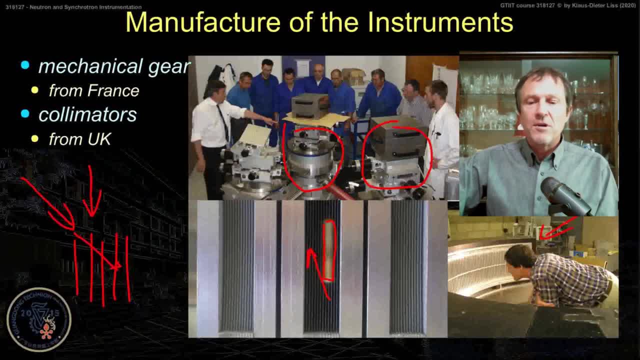 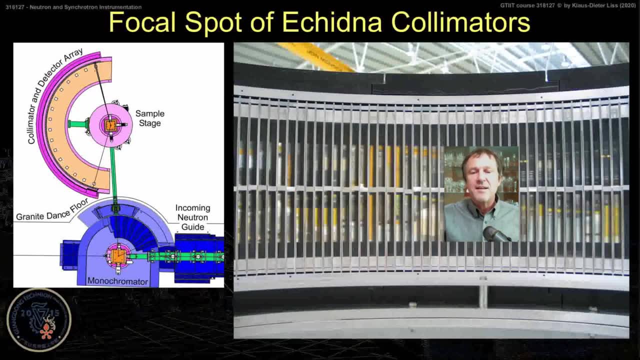 To check And accept the neutron collimators At the factory. Eventually They have been delivered to Australia Sitting here in the guide hall, And if we are in the center, Only in the center, We can look through all of the collimators. 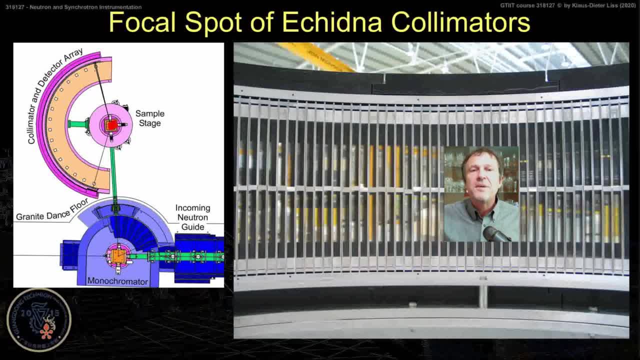 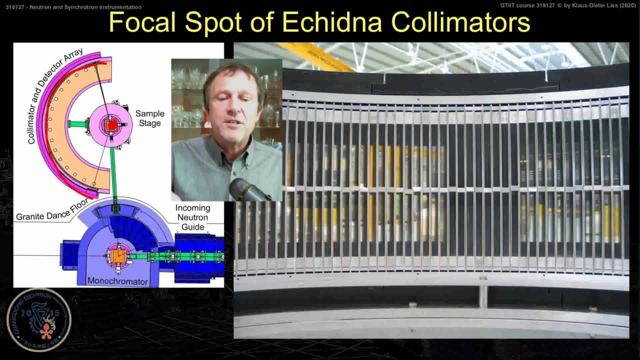 So this is Where the neutrons Are coming from. You only want to see Neutrons from the center Of this circle here, Namely coming from the sample. The entire instrument is here. Neutrons coming from the reactor. 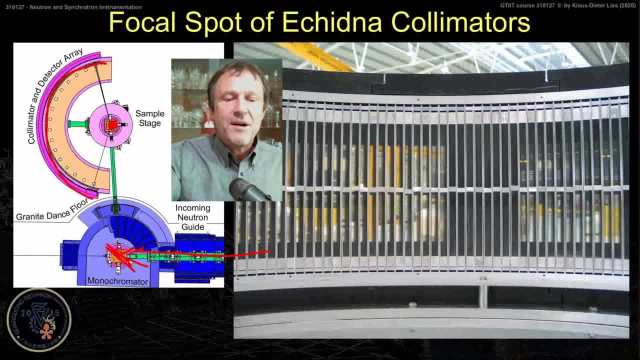 Through the neutron guide. Then you have a crystal mirror Reflecting some neutrons Of a certain k vector Towards the sample. At the sample you do something. You can hit the sample. You just characterize the structure Like x-ray diffraction. 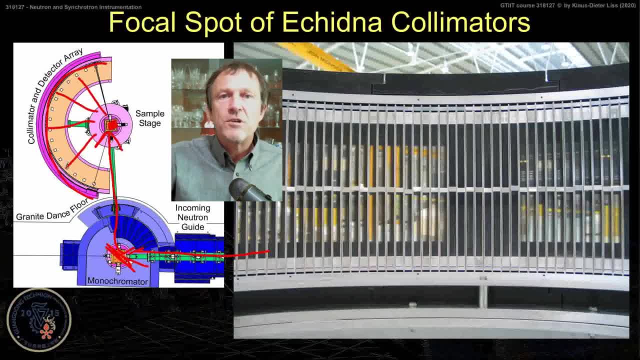 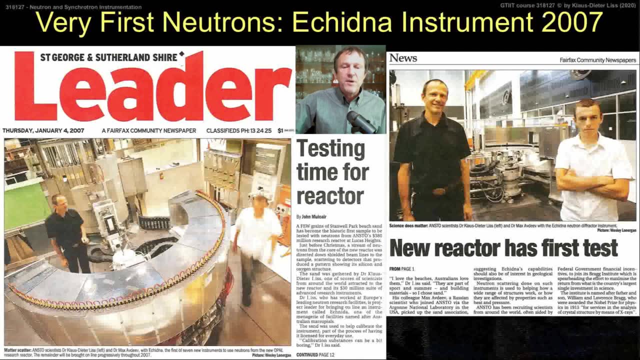 And then the beams. they go here Into the detector. Because neutrons are so expensive, We use a lot of detectors. So here we have 128 detectors Aligned in the circle, And eventually in 2007.. The instrument was 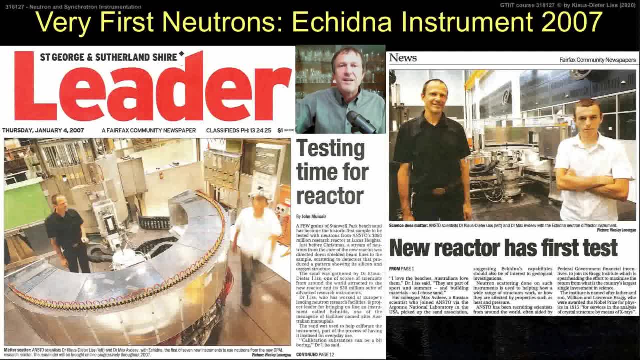 Ready for taking the way first Neutrons. So the detector Was turned on for the way first time And we got the way first. neutrons Through the neutron guide, Coming here to a specimen Which has been sent from a beach nearby. 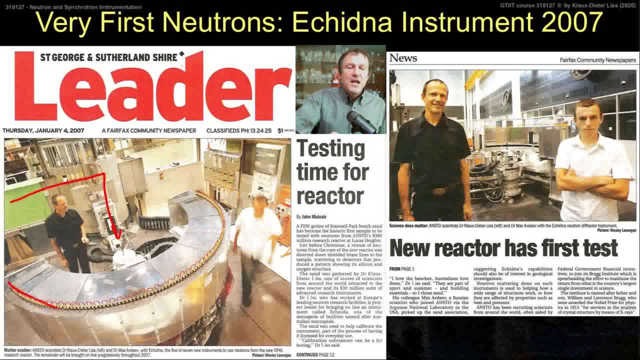 From Stanville Park, A beautiful beach, And intensity scattered into this detector. So there has been The way. first, neutron Defractogram and detection At the Opel reactor In 2007.. After that I became a senior research scientist. 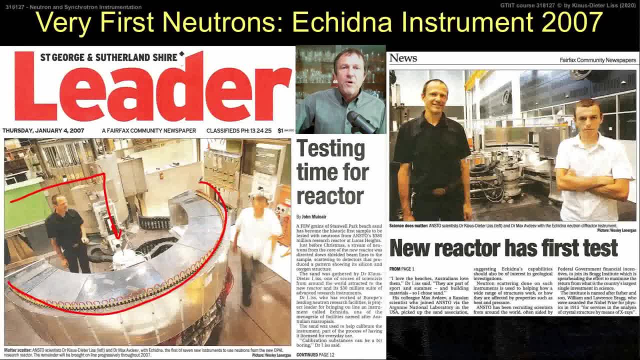 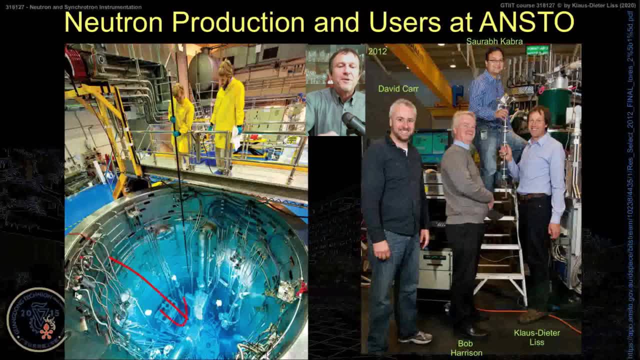 And could do research. So that's where I focused more and more On material science. Two other beautiful pictures, One from the neutron production site, Again here, the reactor pool Towards the wombat instrument Which is in the background, Big equipment on. 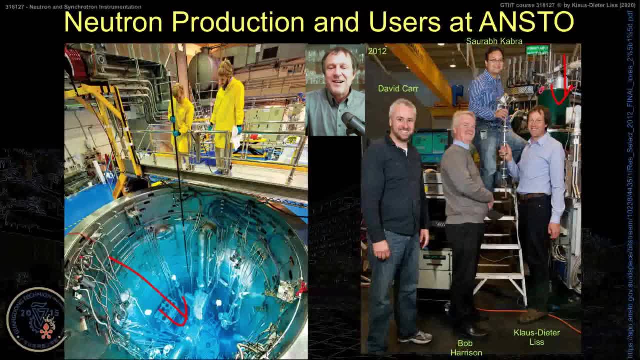 With collaborators. We have Dave Carr here With Bob Harrison, My postdoc at that time. He became scientist at ISIS In the UK, So very well placed now At Oxford And myself here Over the years. The neutron guide hole. 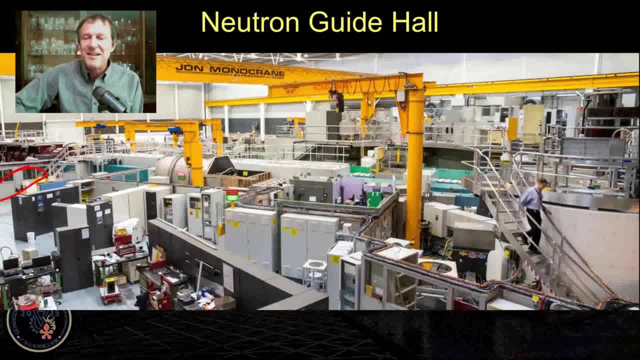 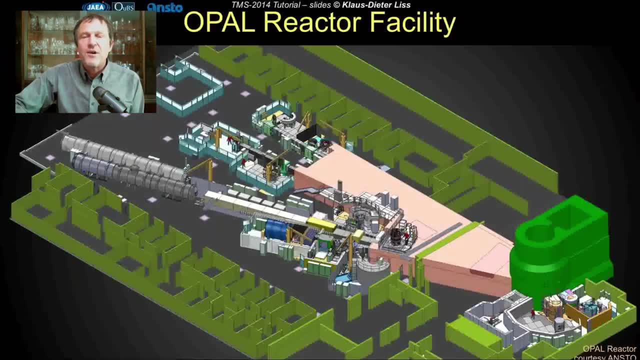 Has been filled pretty much. There is still a little bit of space Around here and there Where we can put one or the other instrument. If this is not enough, There is space to build a second neutron guide hole To the other side of the reactor. 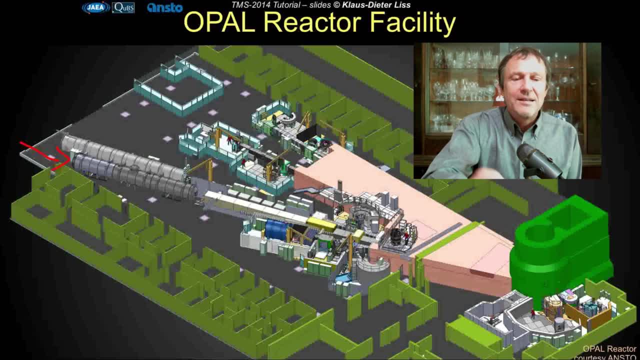 This is a beautiful layout Shown Showing two small angle Scattering machines And again all the instruments, The powder diffractometers Which I have shown under construction. They are shown here, The echidna Which I built. 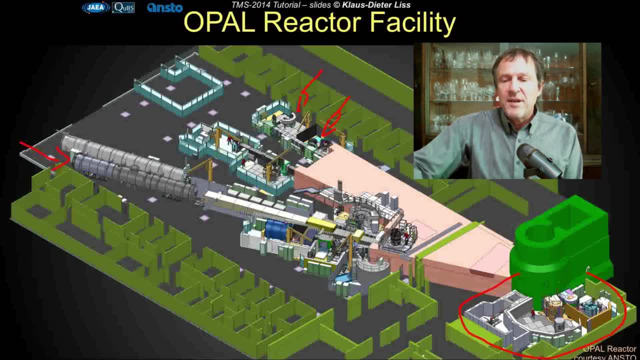 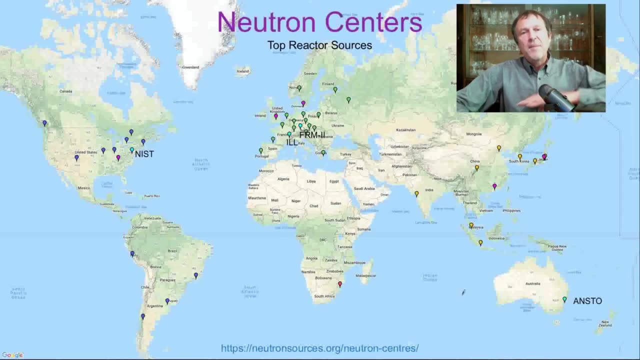 And the wombat Which I used on the other picture. Some instruments directly On the reactor phase- What I said previously- And then neutrons taken out To the second guide hole Of this size. There are many neutron centers in the world. 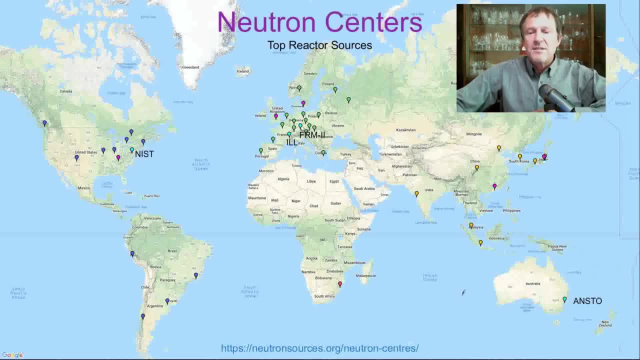 While it is not that many, This map shows Neutron centers According to neutronsourcesorg. Some of the centers Do not have their own neutron source, But they have a lot of instrumentation At some neutron sources Some distance away from them. 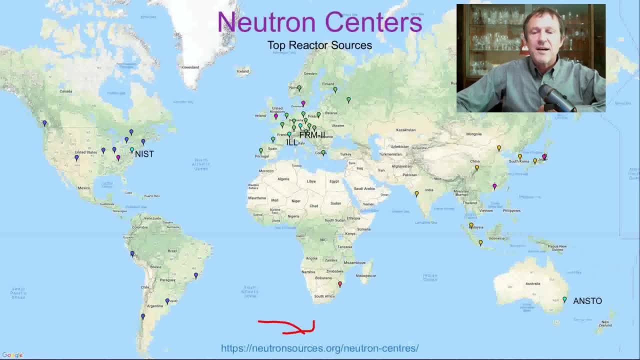 Such that they are listed here. So A few of the major Reactor facilities Are ANSTAL DILL In Grenoble And the Forschungsreaktor Munich FRM2.. At Munich, So I used to study. 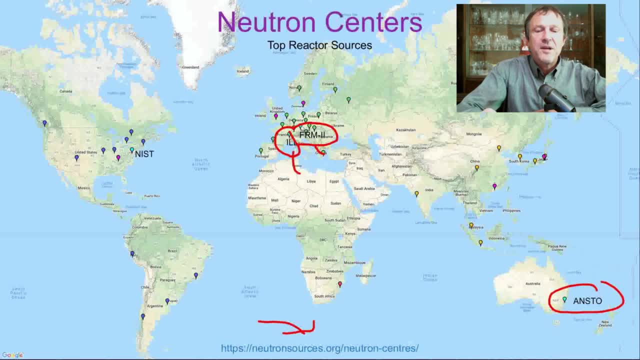 At FRM2.. I did my PhD At DILL And I worked at ANSTAL. There is another high level Neutron reactor facility In the USA, Which is the NIST, The National Institute of Standards and Technology. 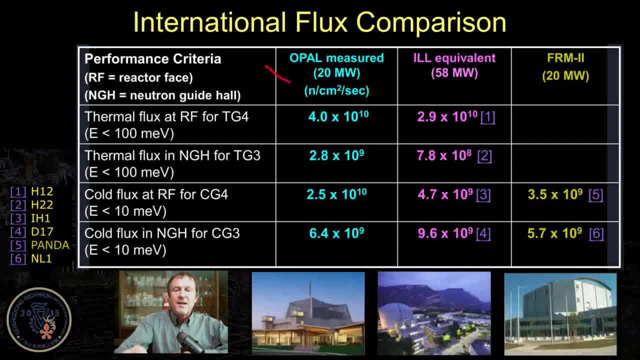 Here I have an internal flux Comparison chart Regarding the Opel reactor, The ILL, equivalent To 20 MW, And the FRM2 reactor, And you see That the Opel reactor Has a very high neutron flux At the reactor phase. 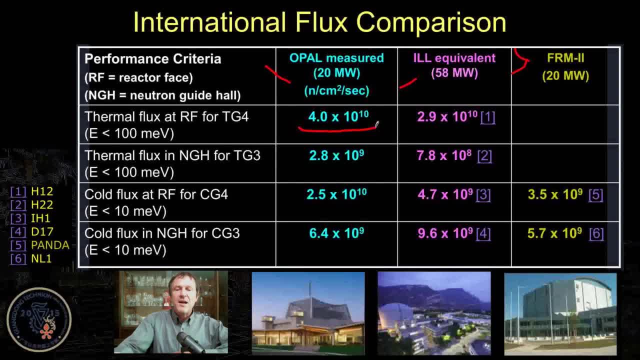 For the thermal guide 4. Which, normalized to the 20 MW, Is even higher Than at the ILL. Other numbers are shown here. If you are interested, you study them. So typically we have a few 10 to the 10 neutrons. 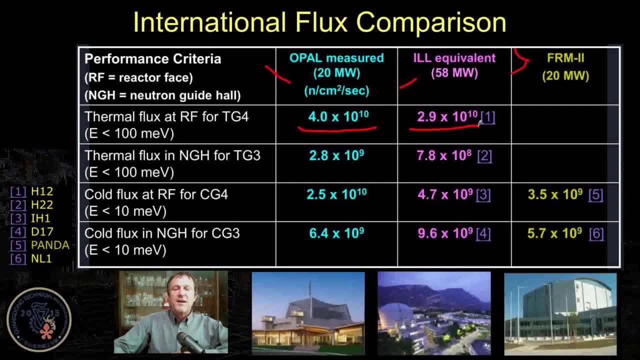 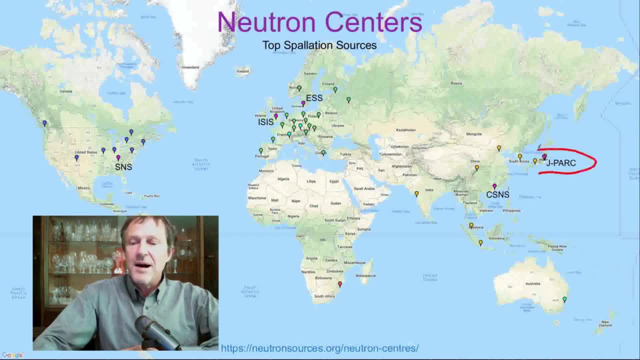 Both for the thermals Or for the cold neutrons Close to the reactor phase. Here I like to show The spallation sources. There is J-Park in Japan. There is the ISS facility, One of the older facilities. 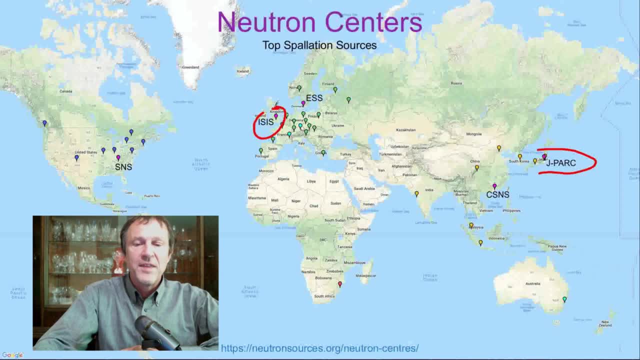 But still very Competitive facility. In the UK There is the first Very big facility, The spallation neutron source. In the USA There is the Chinese Spallation neutron source In Dongguan And soon coming up. 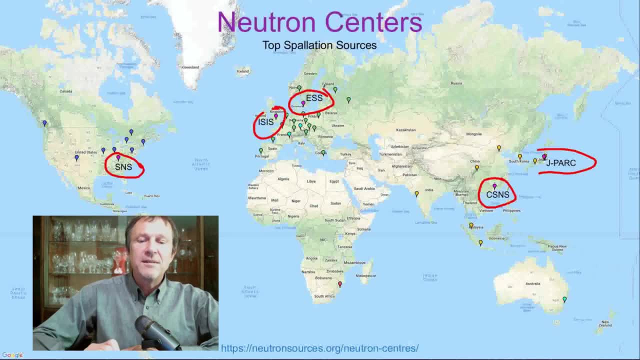 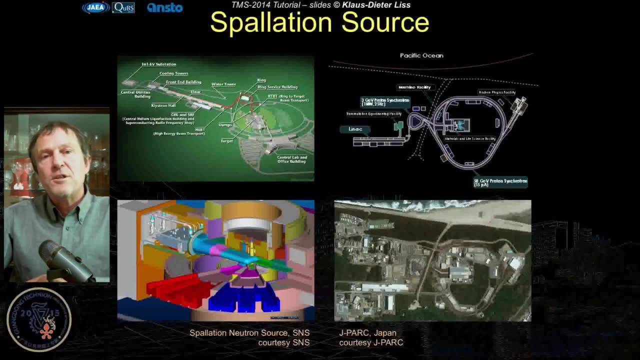 The European spallation source In Sweden. The other spallation sources as well. There is Los Alamos, For example. So how does the spallation source Look like from the principle? Here are some layouts Of the SNS. 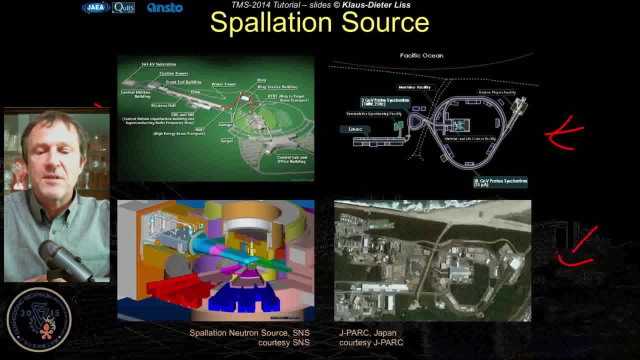 And of J-Park, Together with aerial photographs And technical drawings, What is happening inside. So we have neutrons coming Onto this bluish target. That target Is the spallation target, Where the proton To neutron reaction takes place. 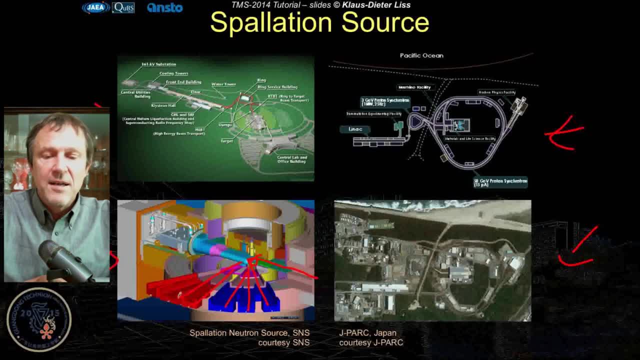 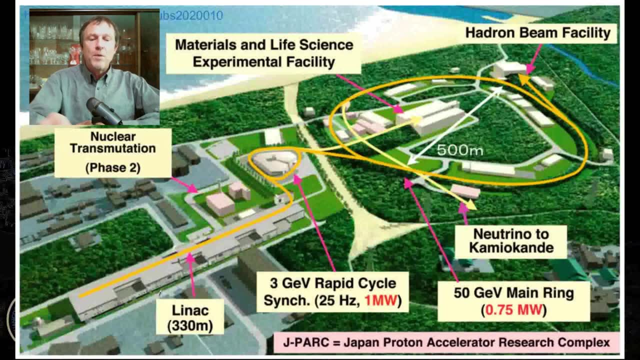 There are moderators, And then it goes Into neutron guides. Let's zoom in Schematically at J-Park, Where we have a linear Accelerator, Hydrogen minus Ions Created and accelerated Over 300 meters. 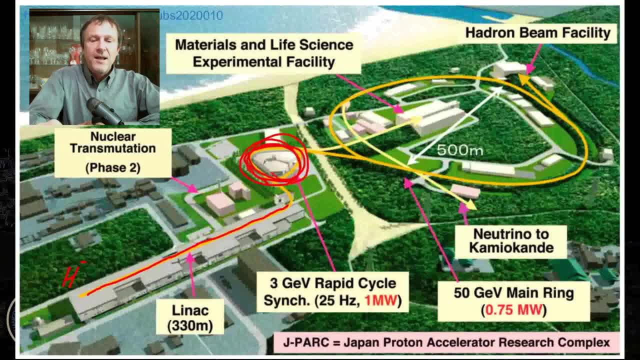 And then fed Into a synchrotron. In that synchrotron They are ramped up And going faster Into the neutron target In this Materials and life science Experimental facility. So this is a neutron facility. 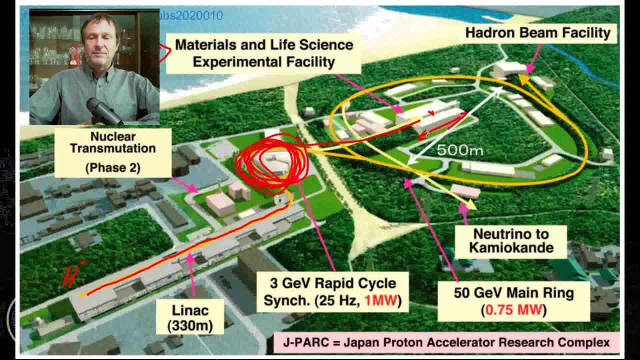 Of about 100 meter Length, With two huge Experimental holes, Of which I will talk later. J-Park is not just the materials And life science facility. They also run the Hadron beam Facility Instead of dumping the protons. 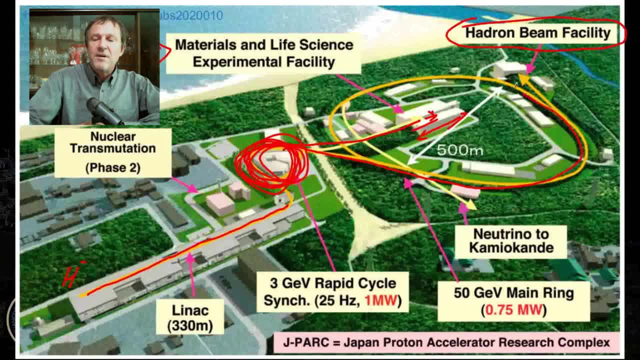 Into an installation source. You can take them into Another synchrotron ring Where they get even Higher and higher, accelerated To 50 giga electron Volt energy. And then Do some Hadron experiments: We change the quarks of the nuclei. 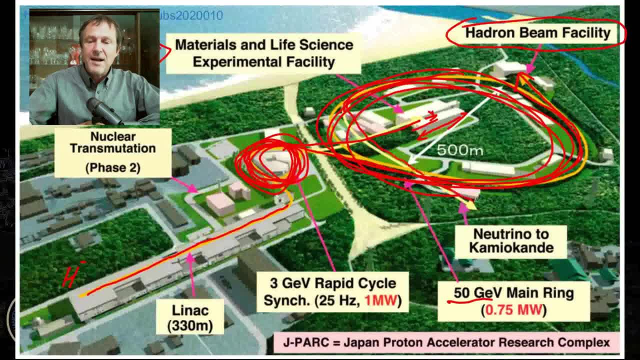 Or You can dump, this way, High energy proton beam Into the neutrino target, Producing neutrinos, Which are kind of Very light Particle leptons Which go 300 kilometers Through the earth, Through the mountains, To Kamiokande. 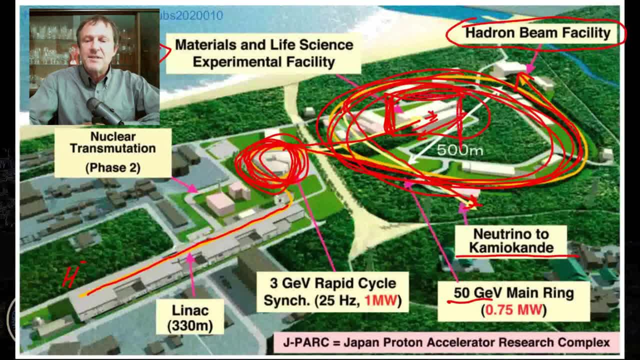 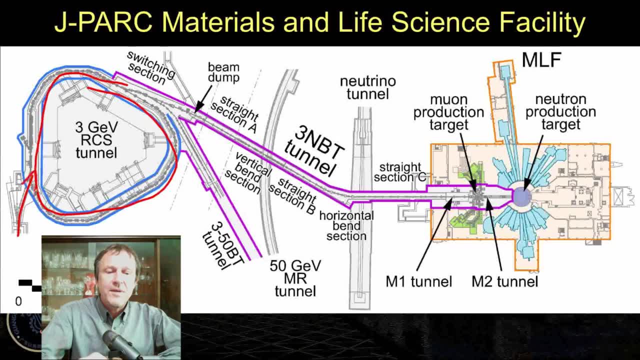 Where they have a detector At the other side of the Japan Honshu peninsula. We are interested here In the materials life science facility In the center And let us zoom in And actually They hit the targets here. So we have two targets. 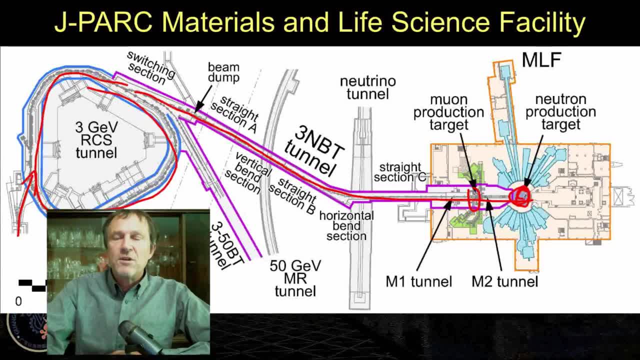 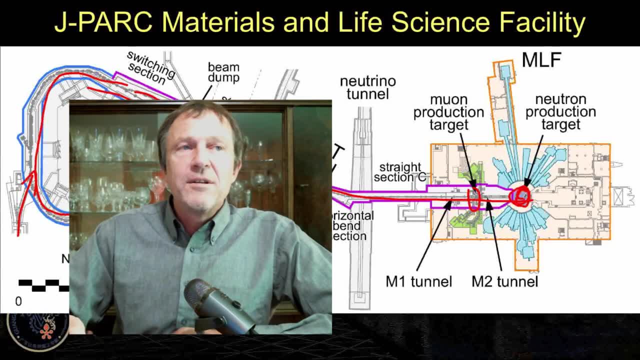 We have a muon production target And we have a neutron production target. In this course We are interested in the neutrons, But I want to say There are also muons. Muons are particles 200 times heavier than electrons. 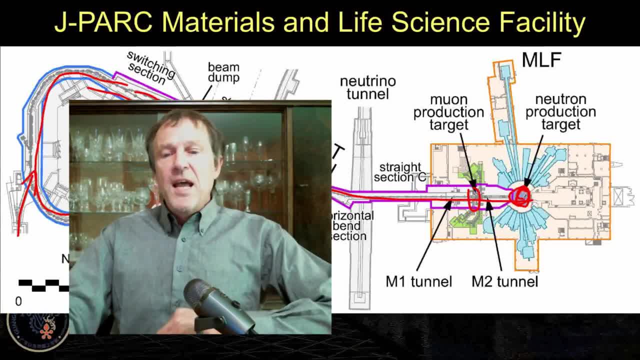 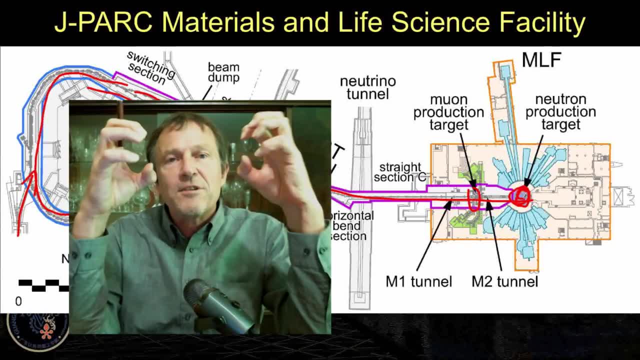 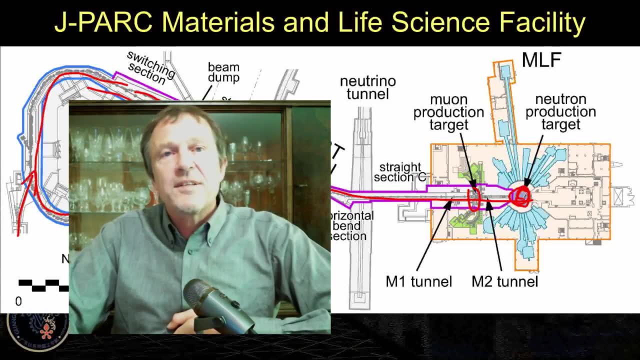 But otherwise They are like electrons. They can be positive or negative. They can go into the material And thermalize And sit in the crystal structure And decay, And when they decay They can irradiate Gamma radiation. You can measure this gamma radiation. 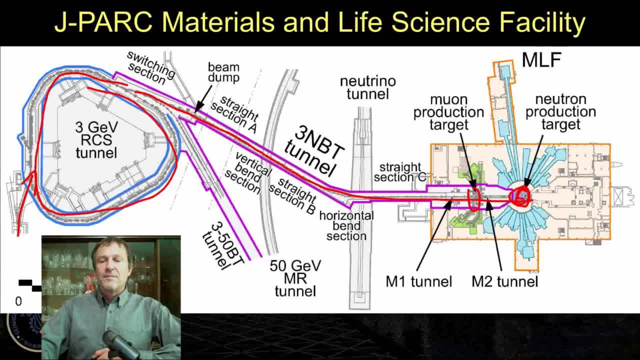 And then work out What has been the magnetic field In your crystal At that stage. Okay, Back to the neutrons. Neutrons are produced here. That one beam line here Is 100 meters long. The list is shown here. 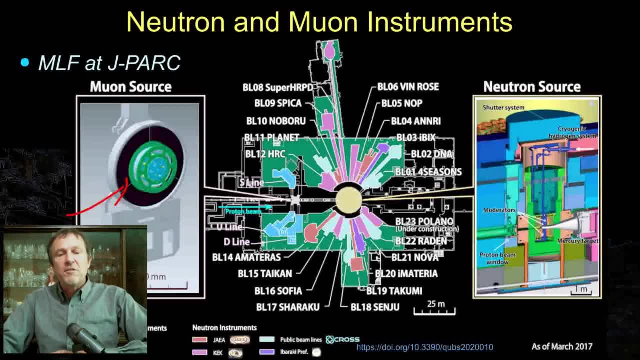 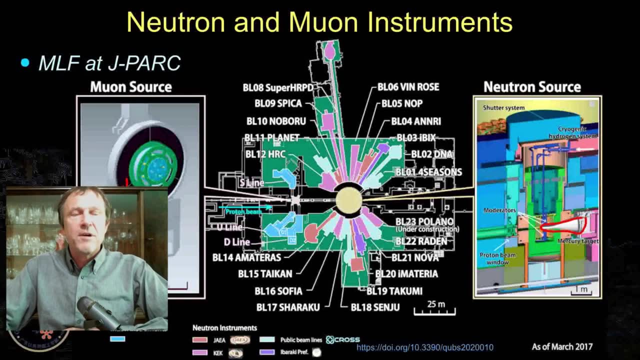 From complete less than muon source, Which is a thin foil of carbon. The protons are Basically transmitted And then hit the neutron target, Which is a huge vessel Of liquid mercury. Also needs a lot, Takes a lot of power. 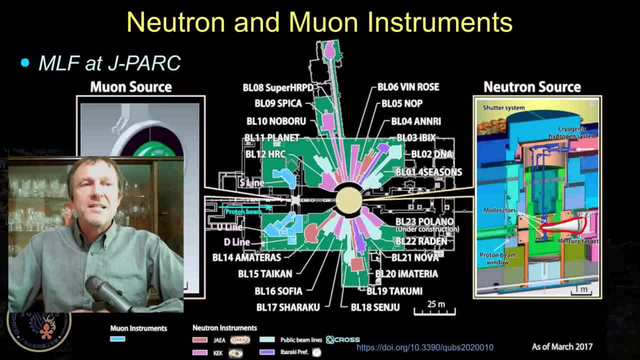 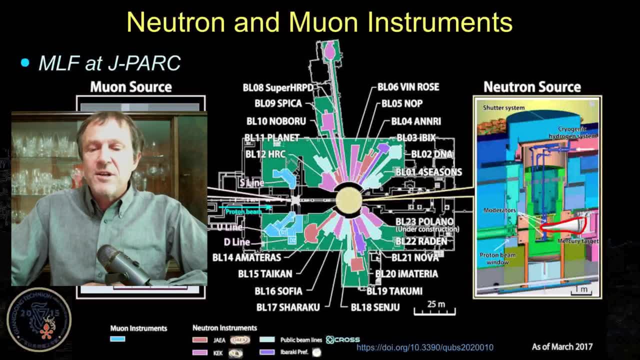 It takes about a megawatt power Which has to be dissipated. It comes in pulses, They have to be dealt with Cavitation and so on. So it's not easy. You get a lot of radiation damage, But you get neutrons out. 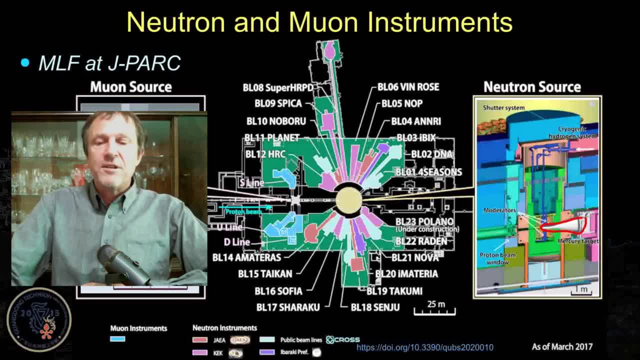 Of this high technology Going into the instruments. And the instruments are listed here. They have names: BL for beam line 06.. Windrose, Raden- Imateria- I used this year. Takumi- I used a few years ago. And planet. 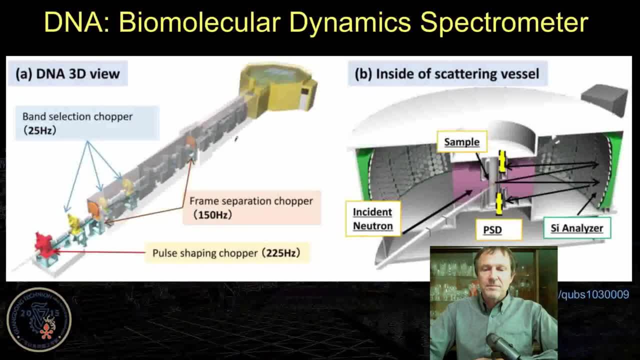 I will introduce The beam line later. DNR Is a biomecular dynamic spectrometer. Just as an example, The neutrons coming here from the source. You have a neutron pulse, But you want to make the pulse A little bit better. 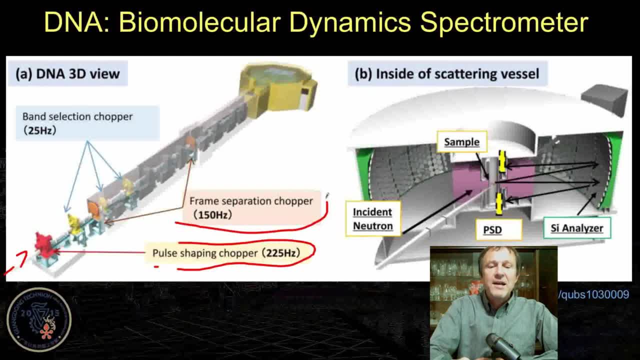 So you want to shape it, And then you want to select the right pulses, So you want to suppress the wrong pulses And eventually The neutrons, they fly To the sample Middle in the center Of a big detector vessel. So this is the vessel. 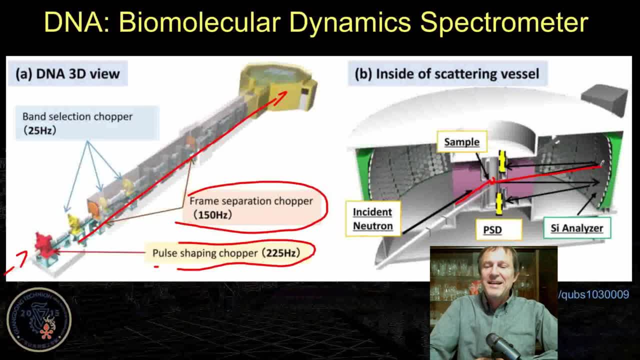 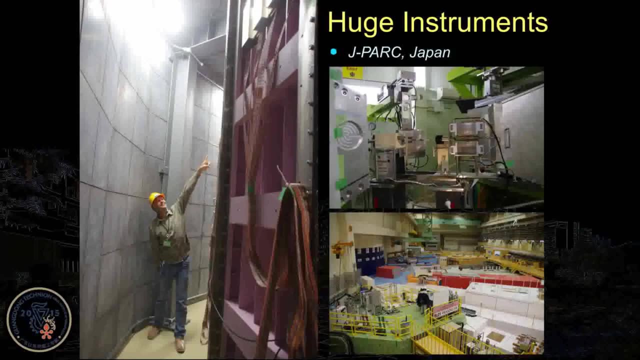 Full of vacuum, The initial neutrons hitting the specimen. Then they hit After some parts of flight Analyzer crystals And scatter into position sensitive detectors, PSD Position sensitive detectors. Impressively, These instruments are very big, So this is one of the detector panels. 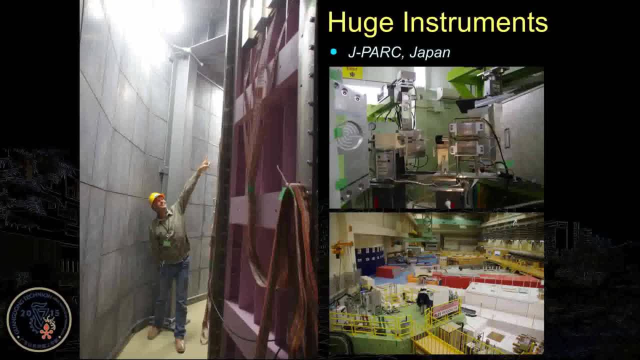 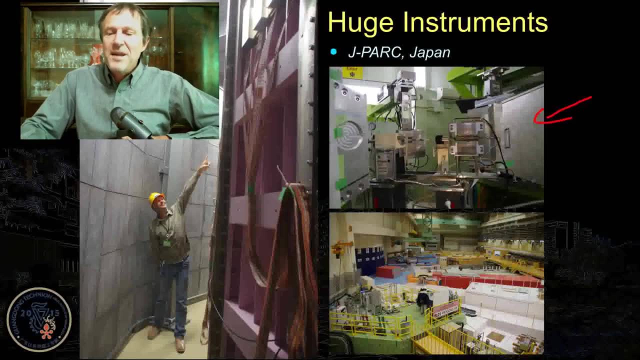 Of one of these huge instruments, Me standing inside there. Here we see the sample station At the Takumi Diffractometer, Where you can measure also stresses And loads in materials. So this is for the mechanical and materials engineering. 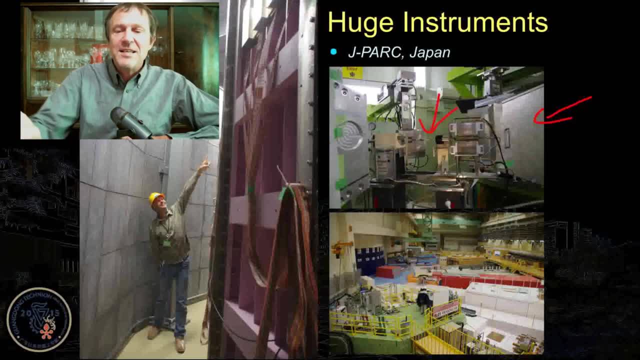 At that stage. We have a furnace here So we can heat the sample To 1000 centigrade. There are two experimental holes. One hole is shown here, The one which I have shown you earlier At the very beginning of the course. 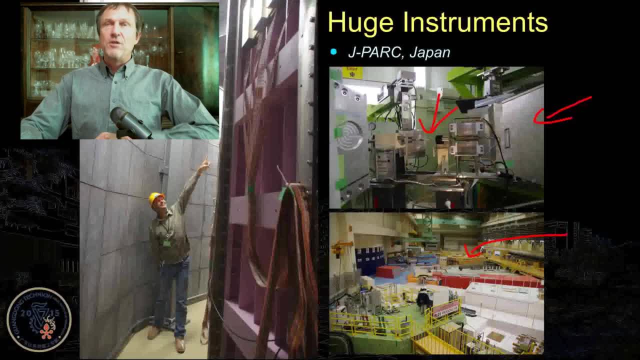 And here You see this orange box. It is a huge box. It is 3 or 4 meters high. It is the beam line called planet. It is called planet because It is a high pressure beam line And people They want to go to very high pressures. 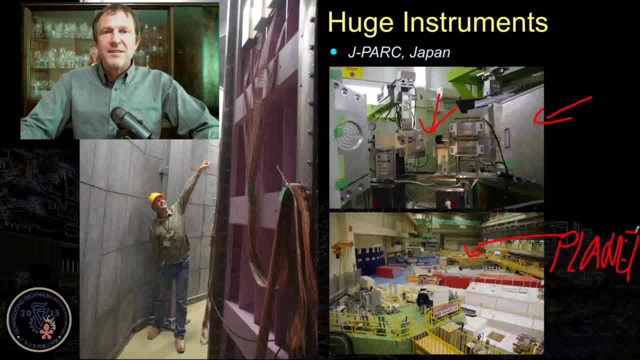 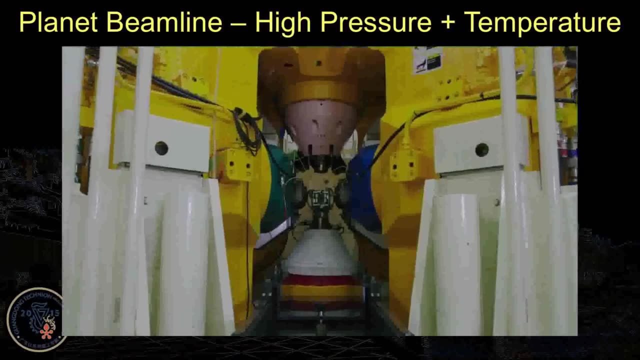 Like in the interior of planets Or the interior of the earth, But we also can Use it for studying metals At high pressures, And two students Sitting in this course here Are now analyzing data From this beam line In my group. 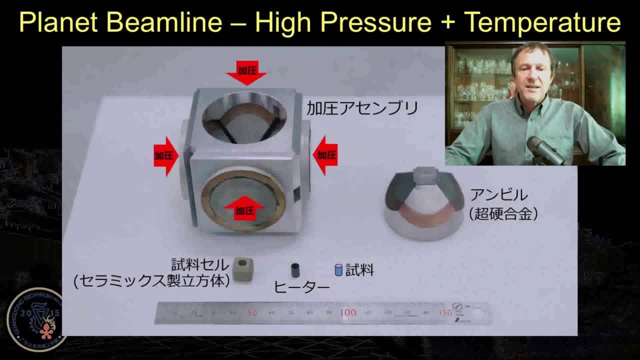 Here a view of the press. This is a huge press Which contains these anvils In the center, So there are six anvils. Basically, the sample is this blue thing at the bottom Which you put into a heater And then into this little ceramic cube. 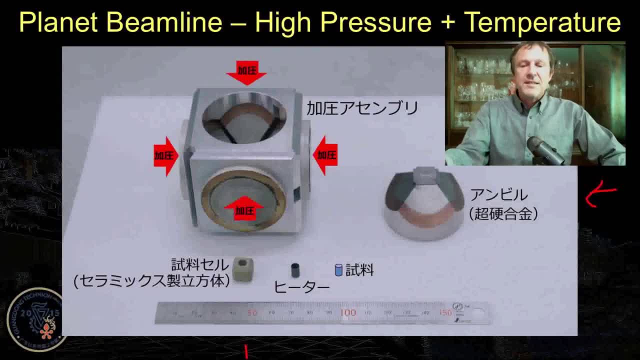 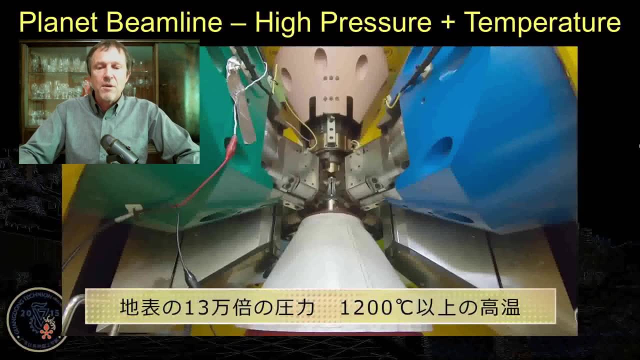 Going at the center Of the anvils, And then you close the anvils By the six sides, Putting them into the load frame. You see the compression here, So the pistons compressing these anvils And like this You can increase the pressure. 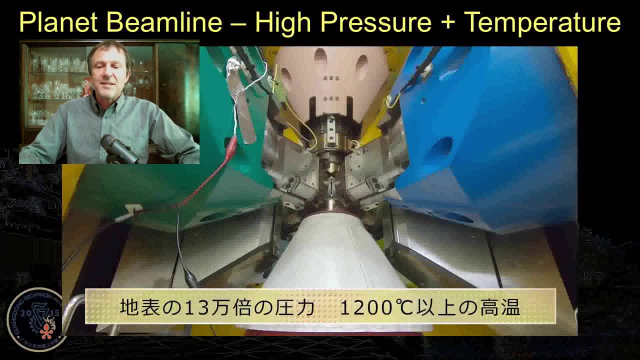 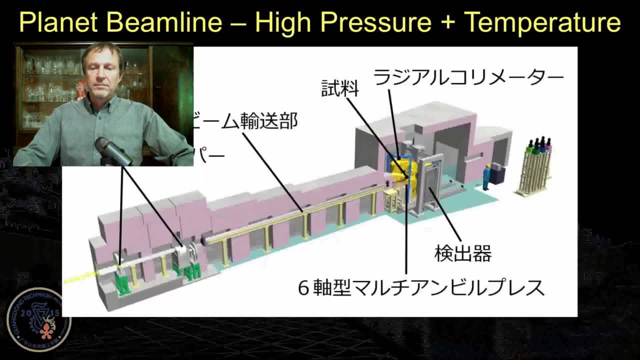 To 13 gigapascal And simultaneously at 1200 centigrade temperature. I show the compression again Now we have the sample here Under high pressure, In the center of this yellow star, And neutrons are coming from the left. 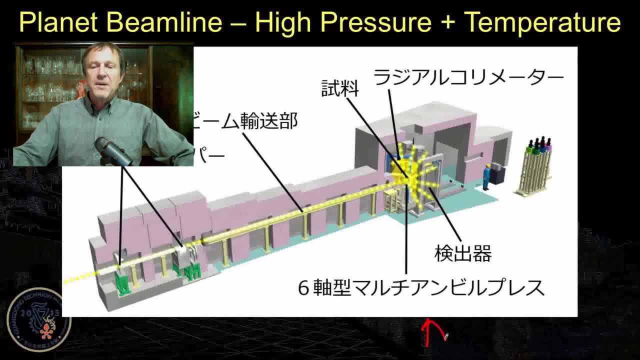 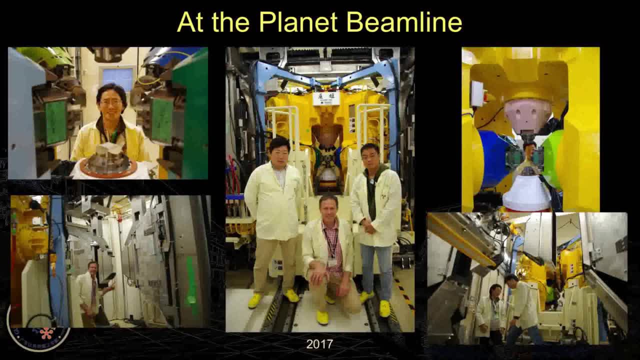 A pulse of neutrons Scattering at the sample And hitting the detectors. Some more pictures Taken during our experiment At the planet beam time At the planet beam line In 2017.. Here my collaborators. This is Pingyang Xu. 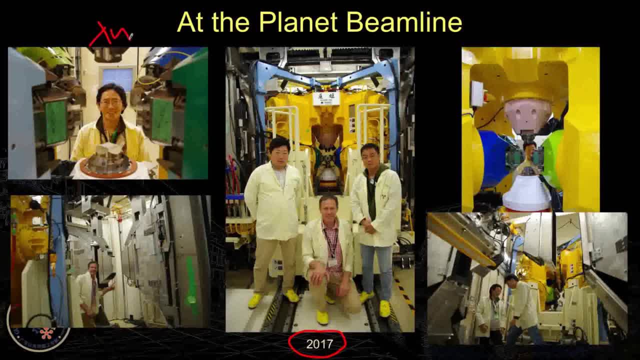 He is a Chinese fellow Working at this Facility. And of course there are other Nice people. There is Fonakoshi san, There is Hattori san, Myself Adventuring between the detector panels here While others align the anvils. 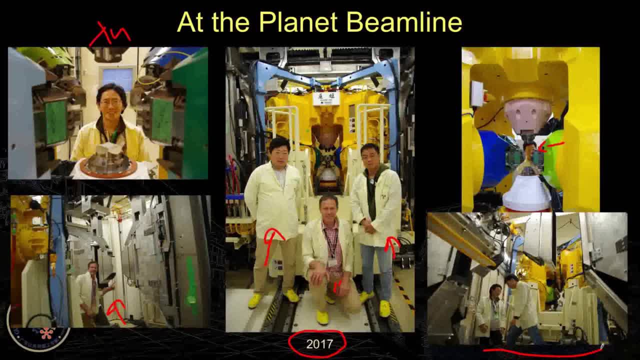 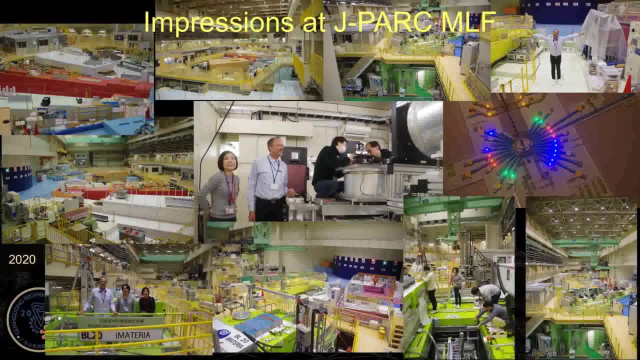 And get ready for the next experimental run. So this is the kind of instrumentation Which I use in my research And where we go At least once per year In this kind of facility- Students- I am talking graduate studies- More impressions. 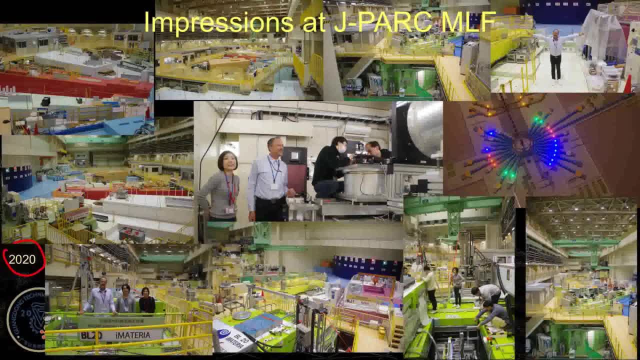 At the Jay Park Materials and life science facility. So this has been now in 2020.. During Corona time, At the very beginning, Where we had beam time At iMateria With the collaboration of Professor Kawasaki, Shown here. 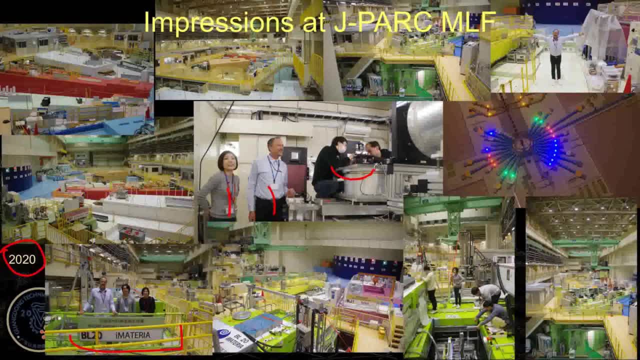 Myself. There is Professor Sano From Ibaraki University. Professor Kawasaki And her student Come from Oregon State University In the USA. You see this huge instrument here Where we have access from the top Through the shielding. 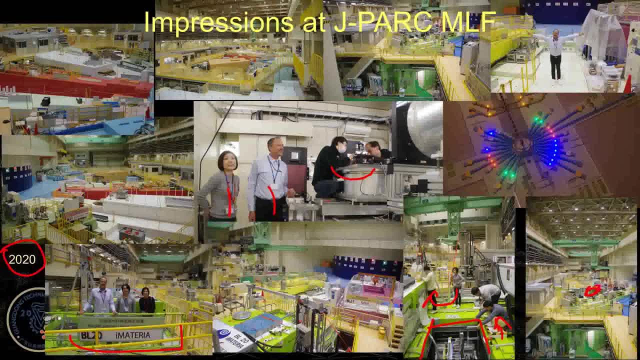 Is just a little dot here In this experimental hole. So that gives you an impression How big everything is. To the top, you see the one hole. To the bottom You see the other hole. This blue wall Are the neutron ports. 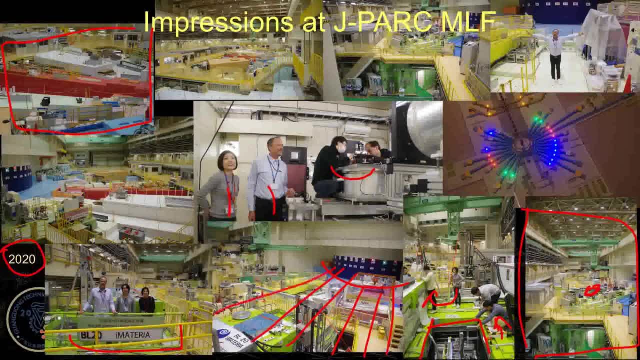 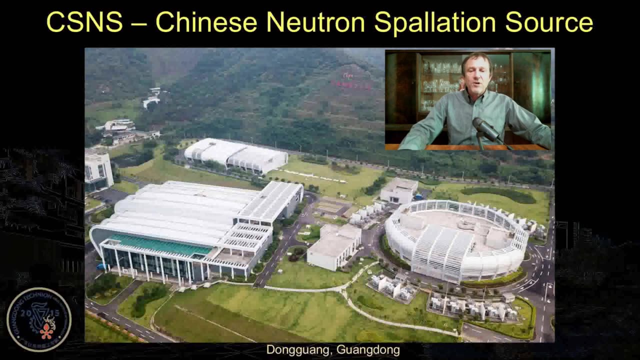 Towards the different neutron guides, So the spallation source Is just behind there And the guides are all radially arranged In a way As shown here By this model. Last, not least, I like to mention the Chinese neutron spallation source. 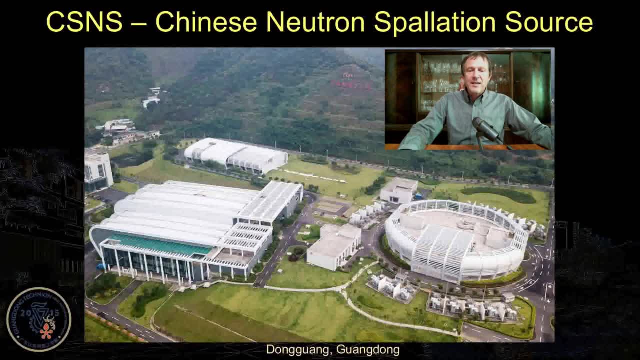 Which has been operational Since 2017.. So, approximately, It is located Only 280 km from us, Namely in Dongguan, In Guangdong province, And can be reached By high speed train From Shantou. 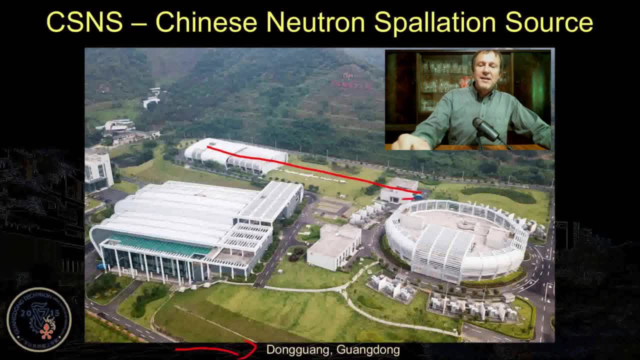 Similarly, We have an accelerator, A linear accelerator. We have a ramp up synchrotron, Where the protons get accelerated To a few GeV, And then We have a target station Inside this hole With neutron beamlines. 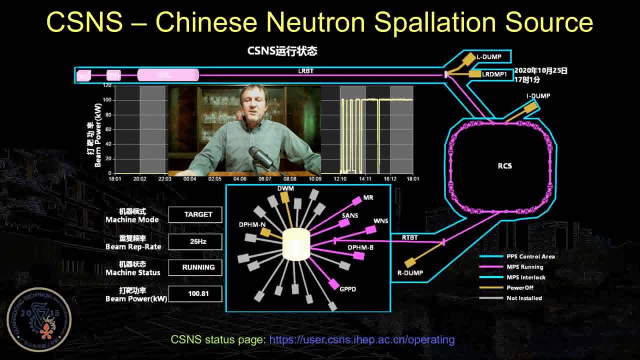 Around. The schematics and the operational status Is shown here on this webpage Again: the accelerator, The transfer line, The booster synchrotron For acceleration And then Hitting the target station here With beamlines around. Three beamlines are operational now. 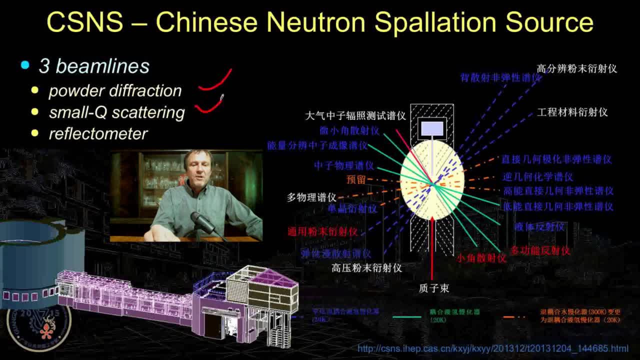 Namely the powder diffraction Beamline, The small Q scattering beamline- Small angle scattering, But Q is more accurate- And the reflectometer With a nice construction. Layout of the powder diffraction beamline Being located here, And the other two. 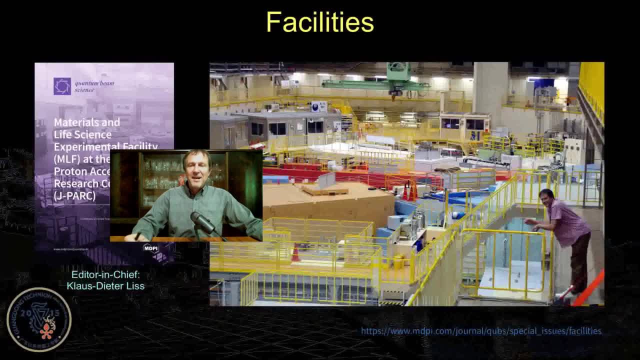 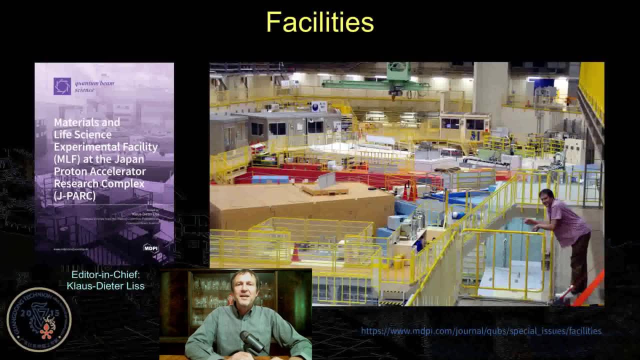 Small angle scattering there, Reflectometer accordingly here. You can read that better than me, I guess. With this We are done with the facilities On the neutron productions. We talked about fission And spallation. Very important is the moderation. 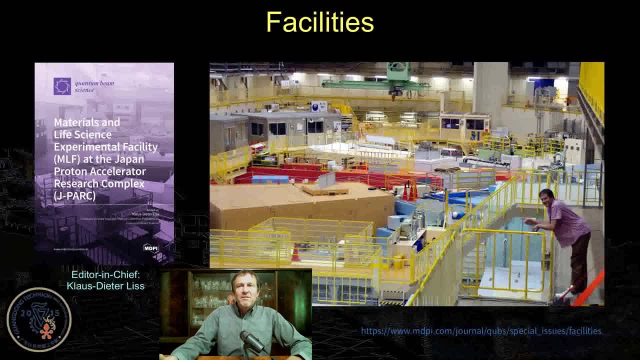 I want you to look up the formula For the moderation, Because the max value and distribution You have not just in neutron science, You have it everywhere. And if you like to know more About some of these facilities, Jay Park, We have compiled this book.